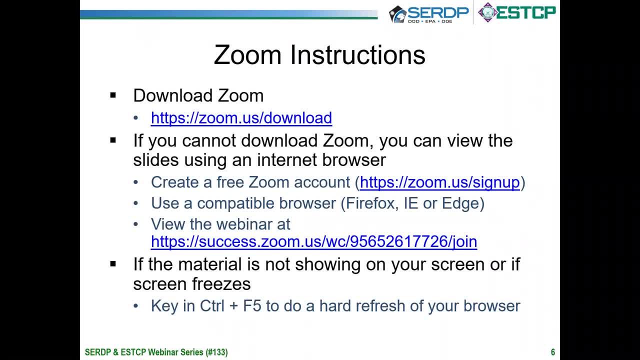 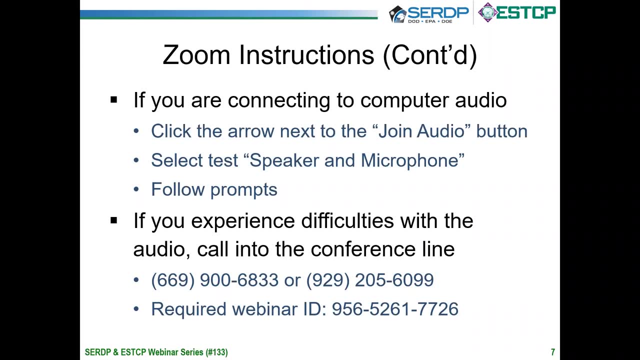 By creating a free Zoom, you can easily download the slides. If you still can't view the slides or if your screen freezes, you can try keying Ctrl and F5 to perform a hard refresh. If you have audio issues and you're accessing the audio through your computer, you can click the arrow next to the Join Audio button, select Test Speaker and Microphone and follow the prompts as they appear on your screen. 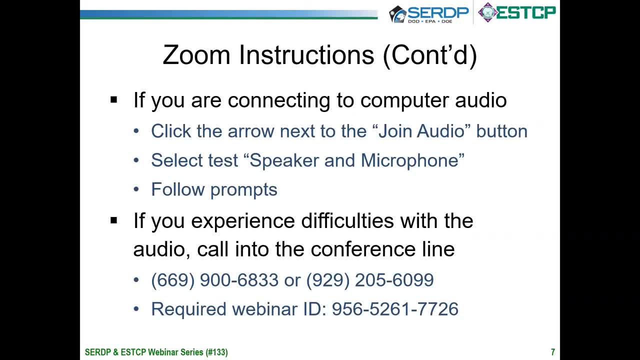 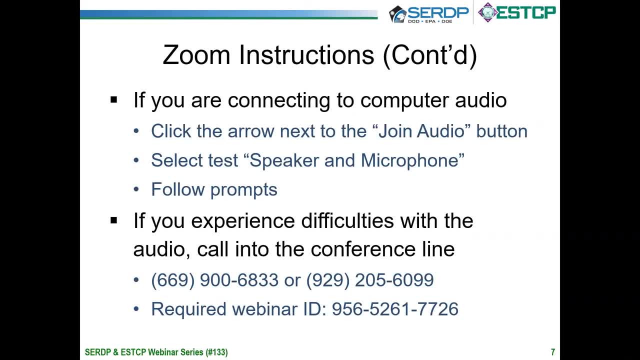 If you continue to experience difficulties, call us or call into the conference line shown here. You can also submit a comment using the chat box. Please use the chat box, though, only for comments related to couldn't all difficulties. The Q&A box should be reserved for questions for the speakers. 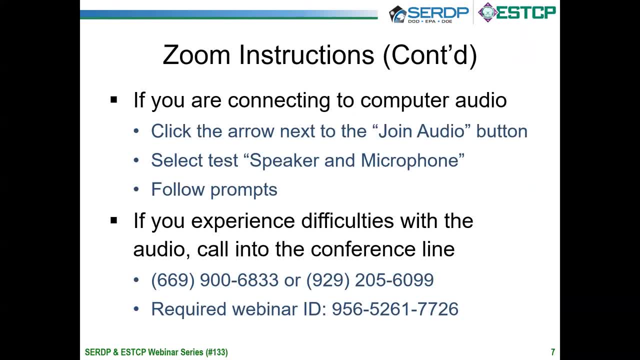 Where we have indeed had in células formulas. it's always helpful to have comment relating to can or after centers On the right hand-maziness, a advertising section Que했는데 for LucasFest 지나던. 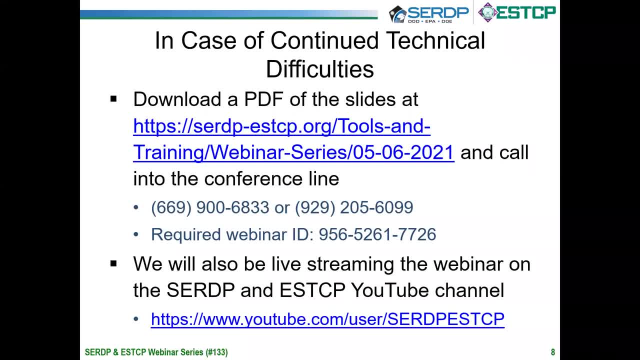 And, in case of continued technical difficulties, you can download a PDF of the slides from the webinar web page and call into the conference line provided to you in your webinar registration email. on the right hand-maziness, a advertising section Que undertaken for the FTS cube. 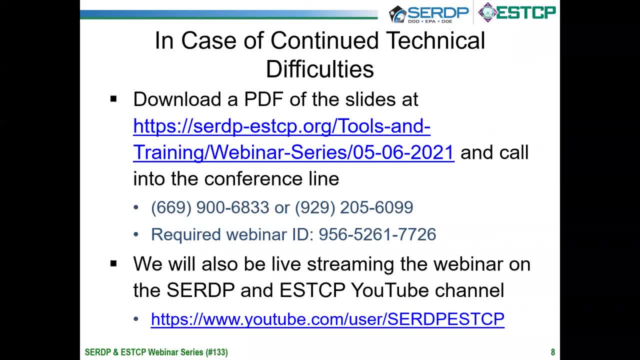 to you in your webinar registration email. We will also be live streaming the webinar on the Certif and ESTCP YouTube channel at the link shown here. Today's broadcast will be listen only. You may submit questions by using the Q&A box, that is. 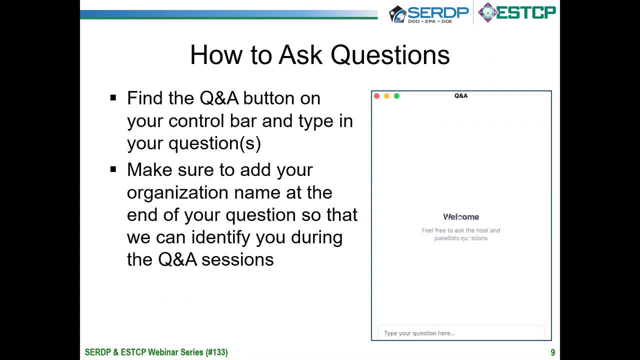 on your screen. You don't have to wait until the Q&A period to submit your questions, and we encourage you to submit them in advance of that session. When you submit your questions, please do add your organizational name at the end of your question. 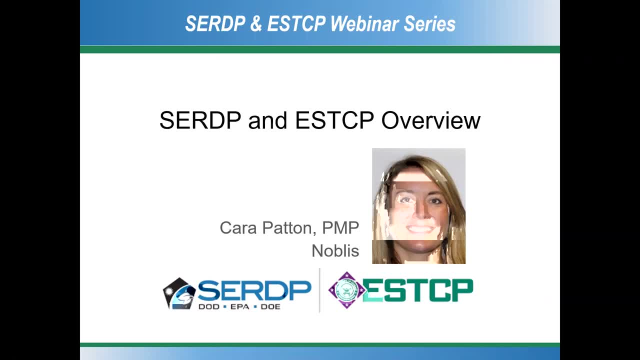 And with that I would like to introduce Kara Patton, an Environmental Project Manager at NOBLIS and the Technical Assistant for the Environmental Restoration Program Area under Certif and ESTCP. Ms Patton has worked with Certif and ESTCP since 2008 under the Environmental 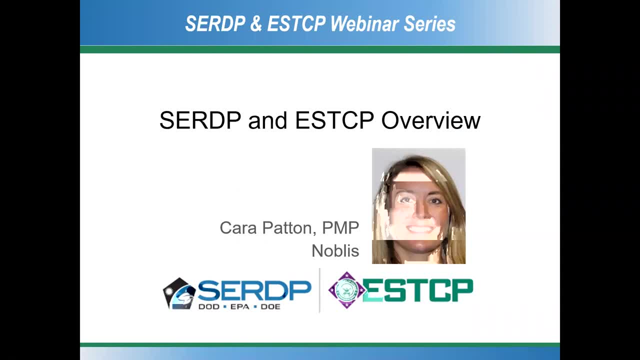 Restoration and Resource Conservation and Resiliency Program Areas. Prior to that, she worked at the Drug Enforcement Administration, where she was a forensic chemist. Ms Patton received her BS and MS in chemistry from George Mason University. Farah, please proceed. Thank you, Jennifer, and thank you everyone for. 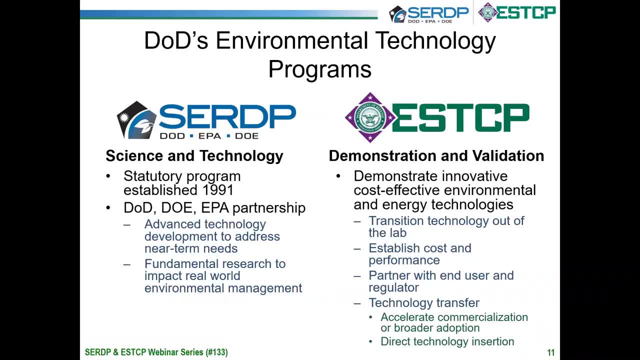 joining the webinar today. First, I want to give you a brief overview of who we are. Certified NEAS- TCP are two companion programs. The Strategic Environmental Research and Development Program, or CERTUP, is a partnership between the Department of Defense, the EPA. 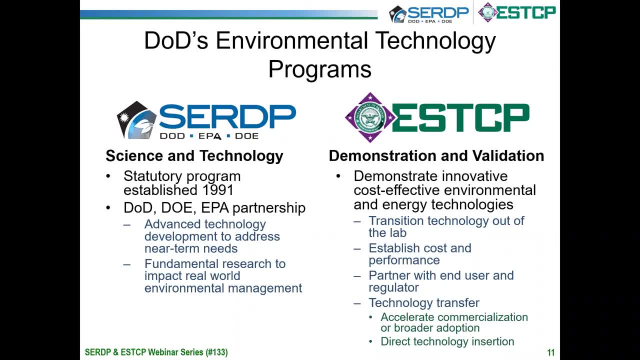 and the Department of Energy and is a science and technology program. We have been around since 1991, and our goal is to develop research from fundamental to more applied so that we can create the knowledge and technologies to impact real-world environmental management. CERTUP operates. 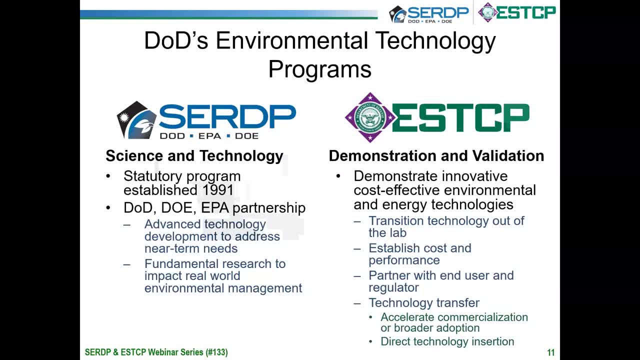 in companionship with ESTCP As a demonstration validation program operated out of the Department of Defense. it is designed to take research knowledge and technologies developed under CERTUP and other research programs and demonstrate them in the field, with the ultimate goal being the technology. 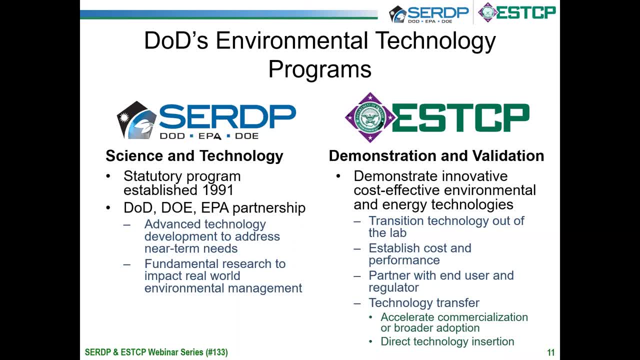 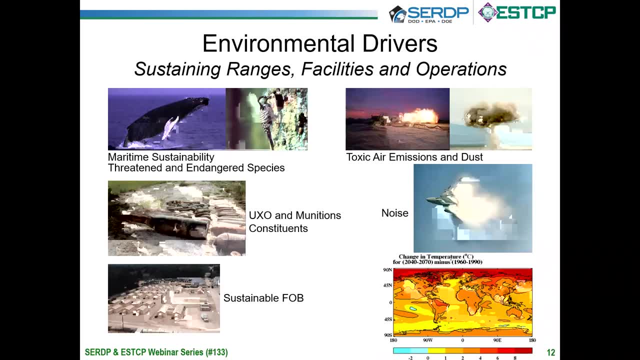 transfer of these technologies to accelerate their broader application and commercialization. Research is guided by a few environmental drivers, the first being sustaining our testing and training ranges, facilities and operations. As you can imagine, this is very broad and covers a range of environmental drivers in itself, such as threatened and endangered species, noise issues. 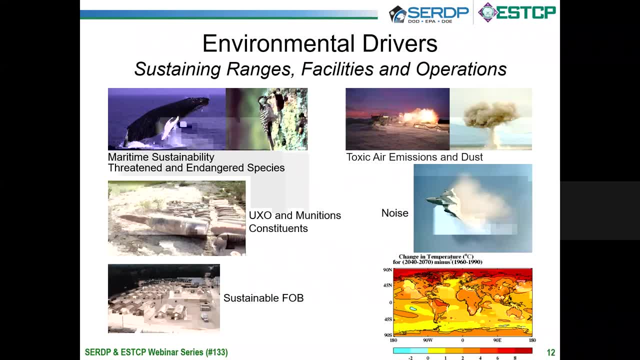 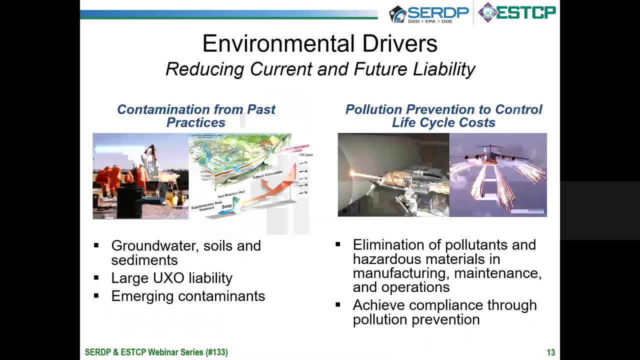 and UXO and munitions constituents. We are also looking to reduce current and future liability, which is also quite broad and can take the form of a long-term and long-term and long-term intervention to eliminate hazardous materials or processes at our military installations. 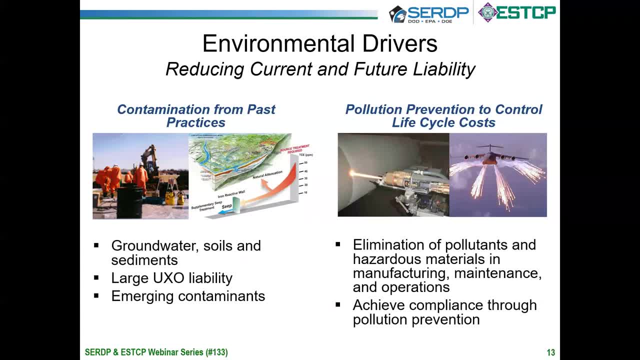 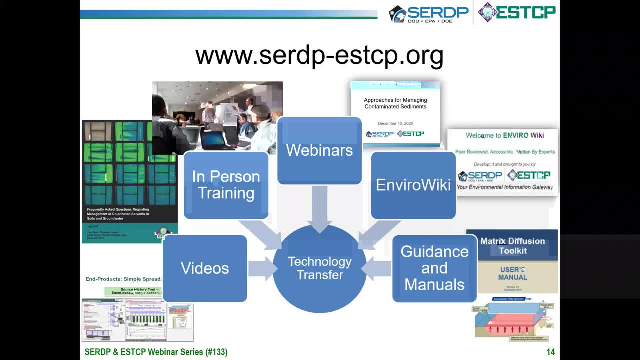 and issues from past practices where we have had impacted groundwater, soils and sediments, and some emerging chemical issues. It is very important for us to transfer the information being developed under CERTUP and ESTCP and we have a number of ways that we do this. 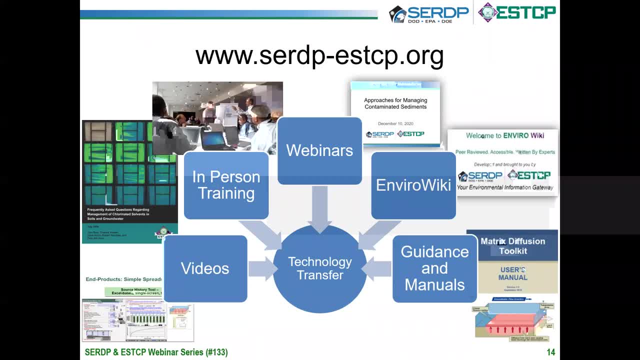 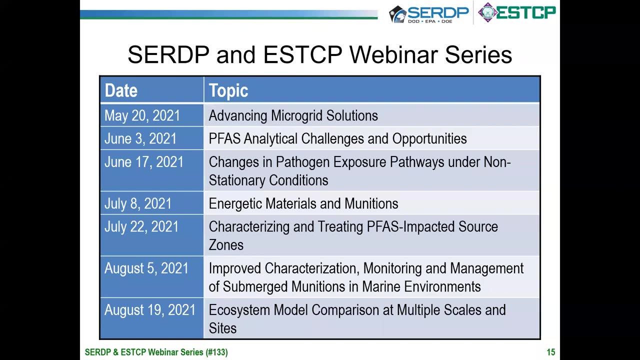 through in-person trainings, videos, guidance and, ultimately, where we are today, our webinars. We are always trying to get this information out to people that are interested in and will use the information Shown. here is a list of some future webinars. We have a few munitions-related webinars in the next few months. 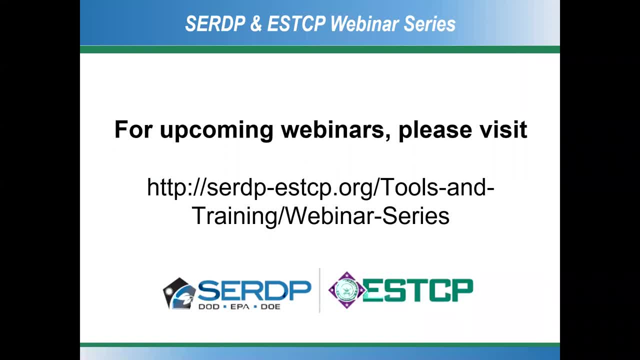 Registration for these webinars are live at the link shown here on this web, on this page and in the webinar chat. You can also access archived webinars at this link as well. Jennifer, I'll turn things back over to you to introduce our next speaker. Great, Thank you so much, Cara. 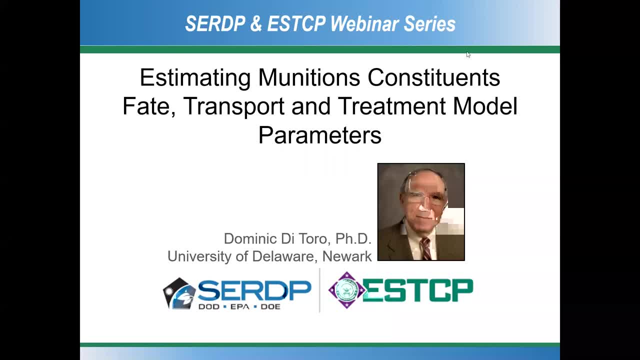 Now my pleasure to introduce our first speaker, Dr Dominique Di Toro, the Edward C Davis Professor of Civil and Environmental Engineering at the University of Delaware. In a parallel professional career, he also served as Senior Research Consulting Engineer at Hydroscience and as Principal. 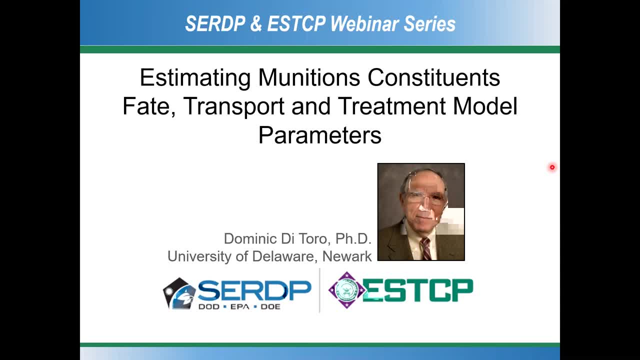 Consultant and Partner at HydroQOL. His major areas of research have been in building models. Dr Di Toro's current research projects focus on PFAS partitioning models and multiple modes of action toxicity models. His awards include the Society of Environmental Toxicology and Chemistry. 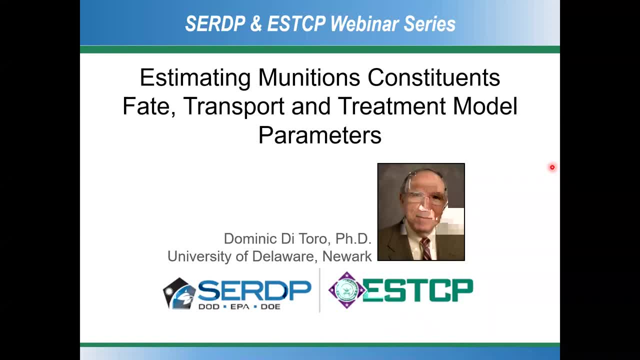 Founders Award and the Institute of Scientific Information Highly Cited Researcher for Ecology and Environment, He was also elected to the National Academy of Engineering. Dr Di Toro earned his Master's Degree in Electrical Engineering and his Doctoral Degree in Civil and Geological Engineering from Princeton University. Dom, please go ahead with. 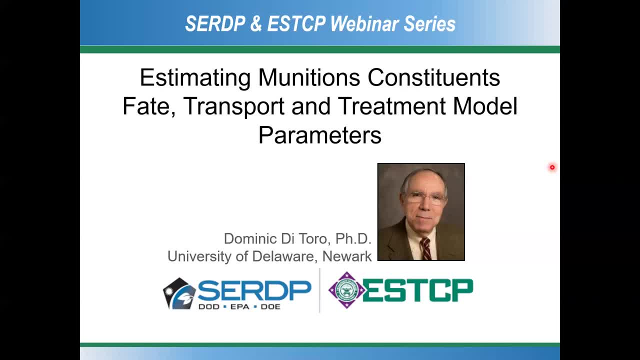 today's first technical presentation. Thank you very much. Good afternoon everyone. Today's presentation I'd like to present to you a model that we've developed for predicting partition coefficients that are required in pretty much every field- transport and, in fact, remediation model, where it's required to determine the 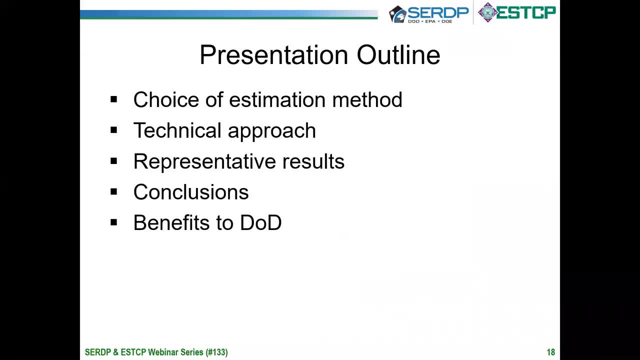 distribution of materials in various environmental phases. So the presentation will start with a choice of the method that we, why we chose the method that that I'll speak to you about how it works, what the technical approach looks like, give you a look at representative results, how well it works, and then end. 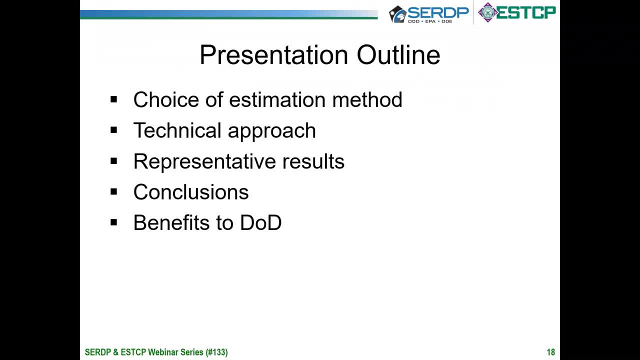 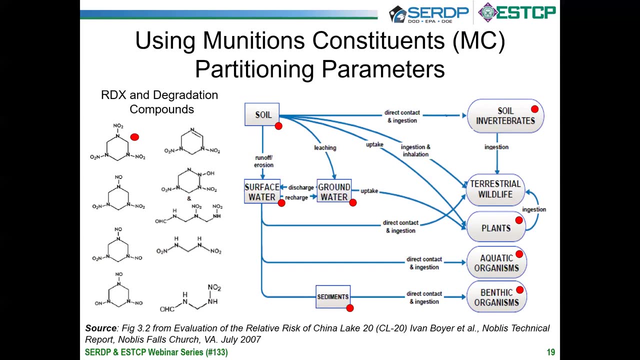 with some conclusions and, finally, a brief discussion of of why you might want to pursue this particular avenue for making estimations. Consider the following situation, which is pretty much characteristic of a risk assessment scenario for a munitions constituents. Let's imagine that you're interested in. 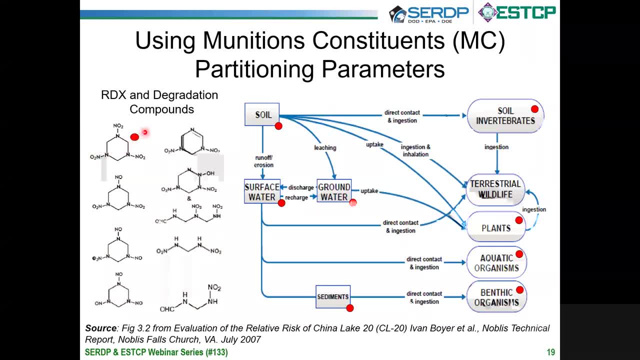 in dealing with R and RDX and you'd like to make predictions that you're interested in dealing with R and RDX and you'd like to make predictions of its partitioning between the contaminated soil, let's say, and all of the other environmental phases that interact with it, So, for example, soil. 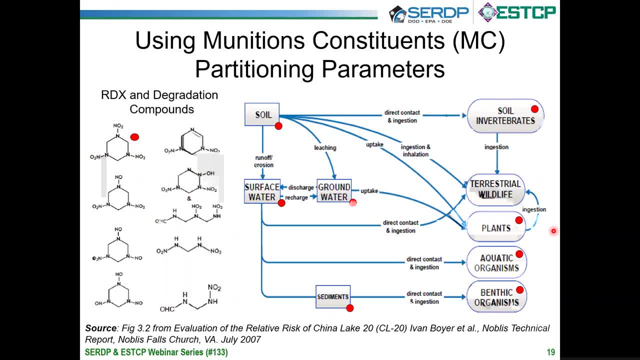 microorganisms are directly contacting the soil. Soil-water groundwater interactions will provide concentrations of the material in groundwater, Groundwater and surface water interactions will a concentration of the material and surface water and from those three exposures you'd like to be able to predict what's going. 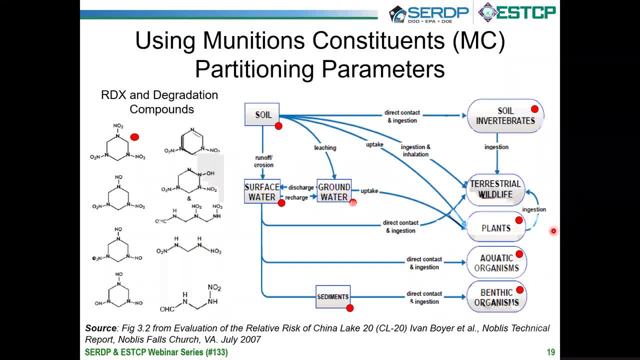 on in the plants that are exposed to the soil, water and aquatic organisms that are exposed to the surface water, benthic organisms that are exposed to the sediments and soil. invertebrates that are exposed directly to to the soil. For a compound like RDX, there's been quite a lot of experimental investigations that 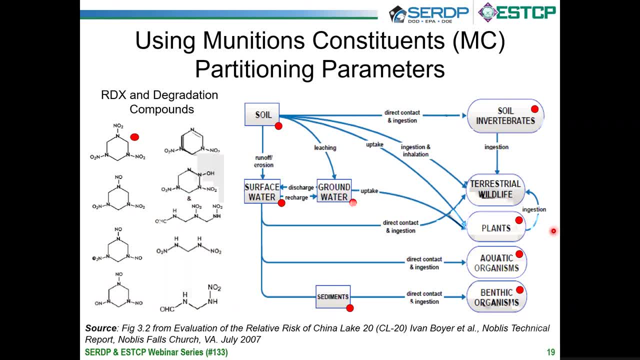 have established one of the. what are the environmental characteristics of the soil? John, you can go ahead and take that out of the. Sorry, I'm getting a message. I have got the. Is the volume better at this point? So the trick is to Beverly. is there a problem? 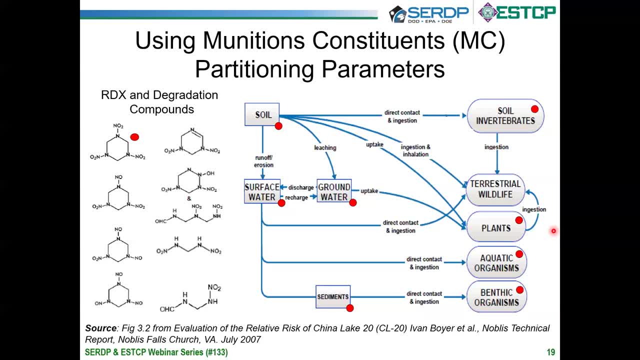 Dom, you're coming through just fine, Okay, sorry. Okay. so what we'd like to do is for RDX, we have experimental information, But what about another compound, For example the first degradation product of RDX? Is there a way that we can estimate the partition coefficients that we need among all of the environmental phases? 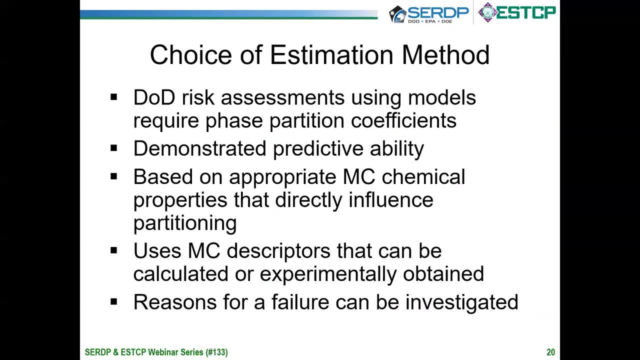 So how does one choose an estimation method? This problem has been around for quite a long time, So this is not a new issue. The risk assessments that the Department of Defense does, and everyone else does, pretty much require partition coefficients. So what? we'd like to choose an estimation method that has demonstrated predictive ability. 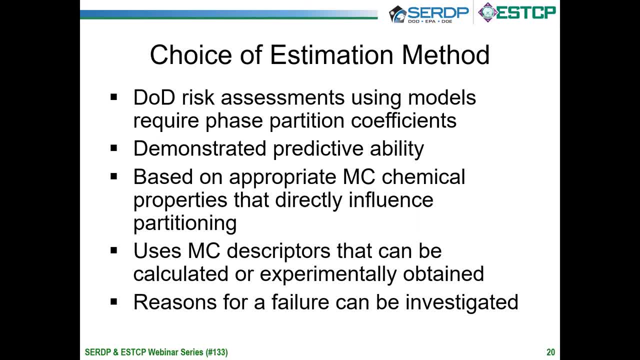 We'd like it to be based on the appropriate chemical properties that directly influence partitioning. In other words, we'd like the thing to be developed using the chemical understanding of what's going on. This is quite different than some of the methods that are currently being used, which basically rely on rather elaborate regression analyses without a direct focus on what really is happening in terms of the chemical properties. And you'll see what I mean when we show you what the method looks like. 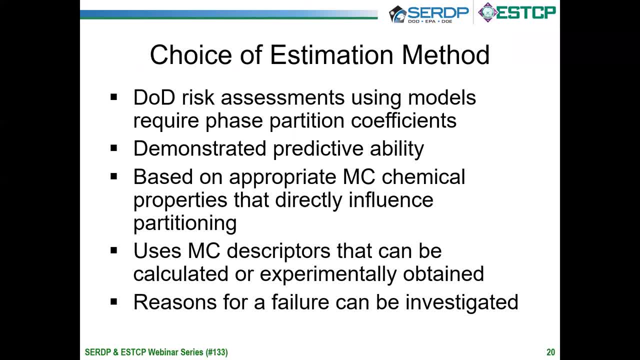 And we would like, by the way, to have descriptors that can be experimentally obtained, if possible, so that we can check at least that the estimates that we're making using the methods we're going to propose are operating sensibly. And, finally, we'd like a method where, if the estimation is failing, 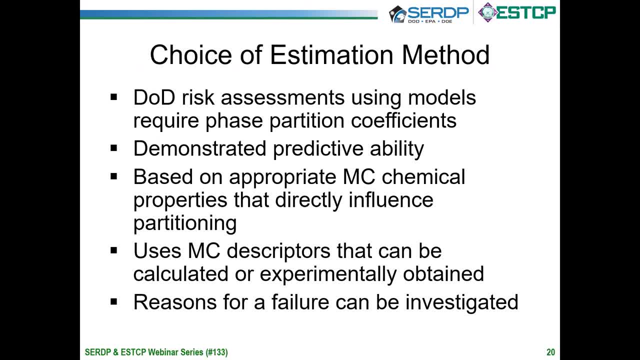 we have some idea what's going on. We have a way of investigating what is causing that failure, And one of the major impediments for using black box type estimation methods is that you have no idea why it's failing. Worse, you probably have no idea why it's working. 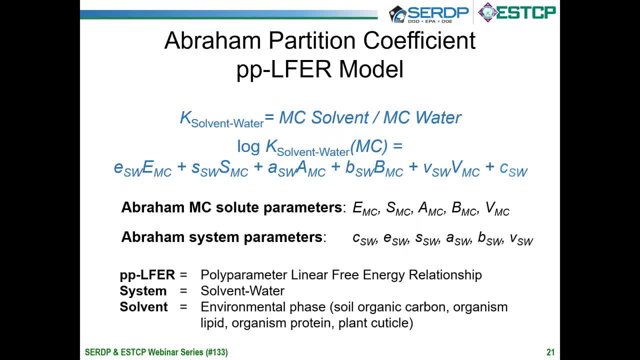 Either of which is a sensible way to operate in my opinion. So the choice of partitioning model we adopted is the so-called Abraham partition coefficient- PP-Lieffer model, which is a mouthful. Michael Abraham developed this many years ago- actually It's quite old and it's been used quite a lot by various groups of people. 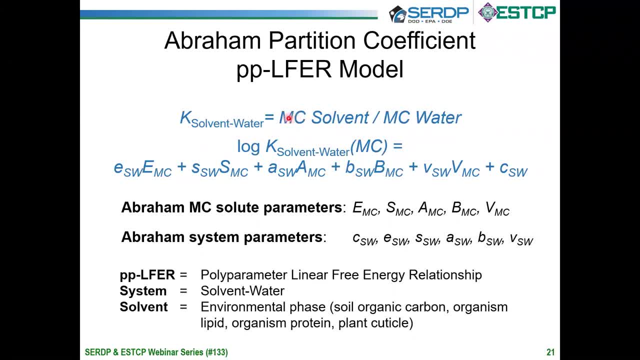 And it's set up as follows: The partition coefficient equation- think, initially it dealt with the partitioning between solvents and water. So think octanol, water, partition coefficient. And it is the ratio of the concentration of the RDX, let's say in the solvent octanol, over the concentration of the munition constituents. again, RDX in water. 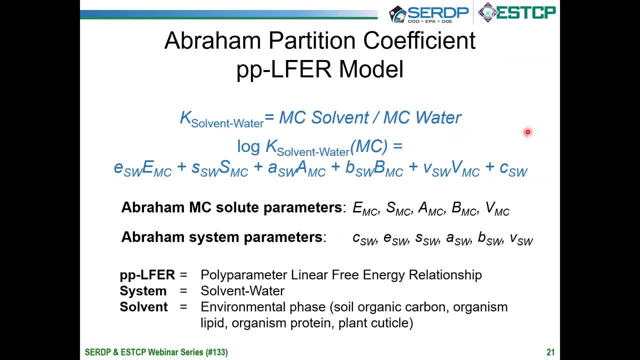 So the Abraham model is set up this way. The log of the partition coefficient is equal to a series of six terms which are additive in the equation, And the reason that it's called a PP-Lieffer is that it's a polyparameter method, which means there are six terms linearly and that the terms actually have direct chemical meaning. 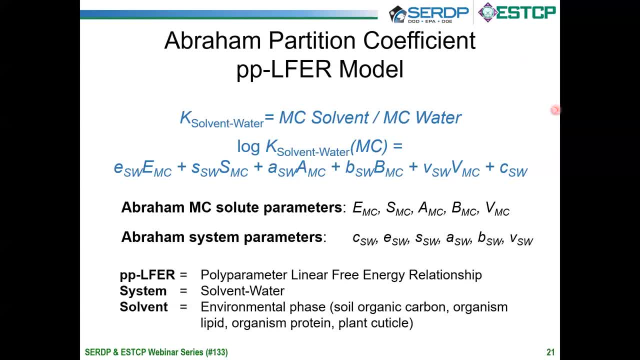 I remind you that the log of a partition coefficient is proportional to the Gibbs free energy of the reaction, the reaction free energy, And at equilibrium that reaction free energy is zero. And so you'd like to calculate what is the delta G- And that is the way Abraham set this up- is that each of the terms in the equation is a contribution of that particular chemical interaction. 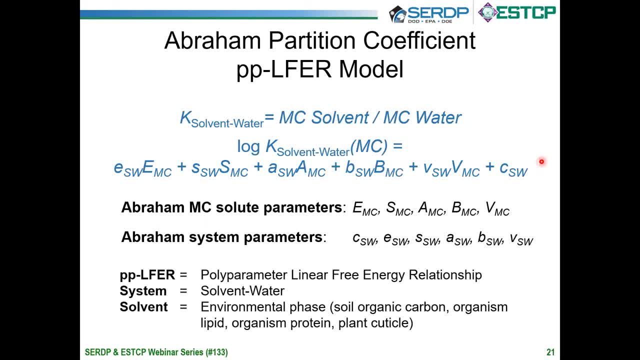 between the solvent and water And in particular, on the next slide I will show you what they mean. But just to get some of the nomenclature clear, Initially this was all solvent water, partitioning octanol water, hexadecane water and so on, And so the nomenclature has persisted. 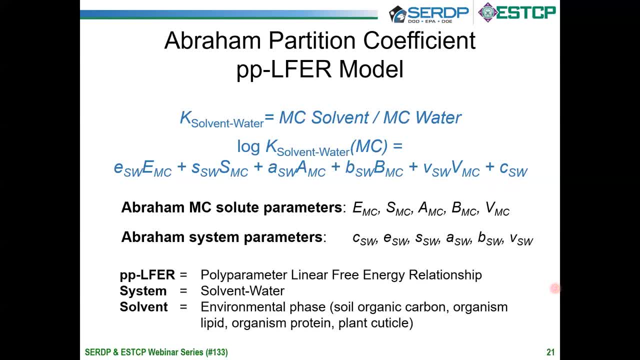 When you hear me say solvent, think soil organic carbon or organic organism lipid or so on. And when you hear me say system, think either a solvent and water, octanol water, for example, or soil organic carbon. Okay, so the partition coefficient is the ratio of the concentration of the chemical in organic carbon, let's say, divided by the concentration in water. 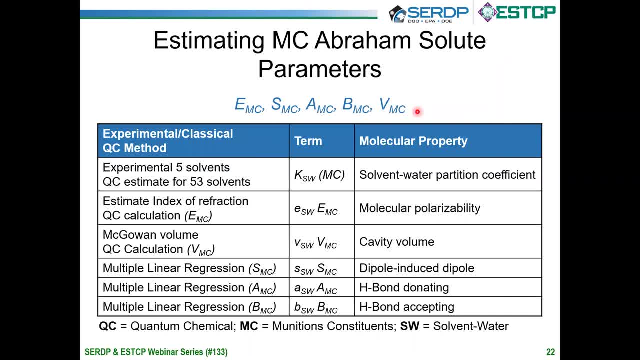 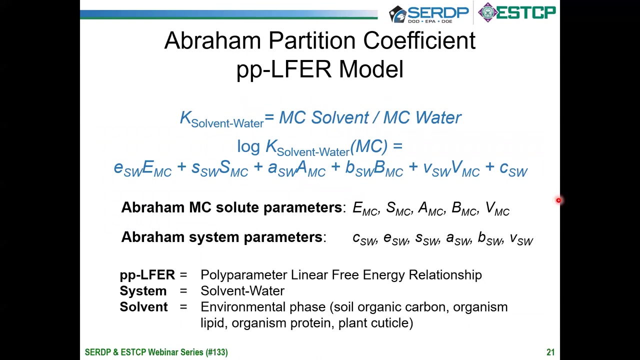 So how does this work? The terms in the model express direct chemical interactions that contribute to the reaction. free energy of the. the Gibbs: free energy of the reaction. The first quantifies molecular polarizability. The uppercase letters. uppercase letters are the parameters that are associated with the solute RDX. 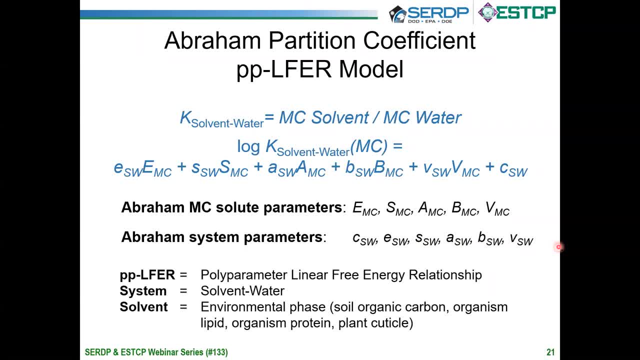 The system parameters. the lowercase letters are associated with the system that you're dealing with. Think octanol water or soil, organic carbon water. How we get both of these parameter sets I'll discuss in a minute, but I'd like first to discuss what it is that they are modeling. 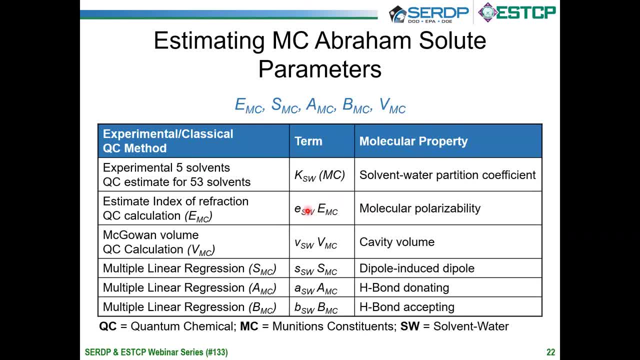 So the product lowercase letters, which are the system parameters, and the uppercase letter, which is the solute parameter, is modeling molecular polarizability. Basically, the idea is that if I have a molecule and it comes up against another molecule that has, and of course the electron distribution generates an electric field. 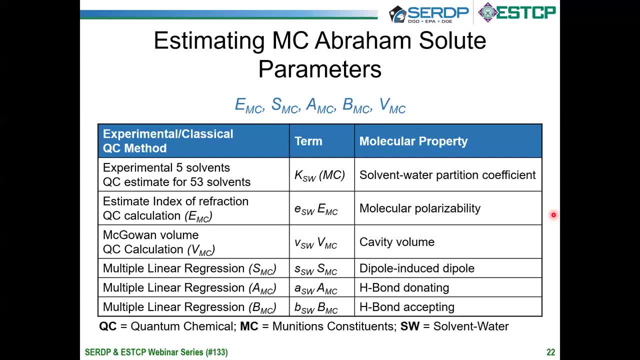 and you get interactions between the, the electric fields, the solute will polarize and that polarization causes an attraction and that attraction is the effect of molecular polarizability. That is effectively the Van der Waals interaction that occurs. It's the weakest of the interactions that 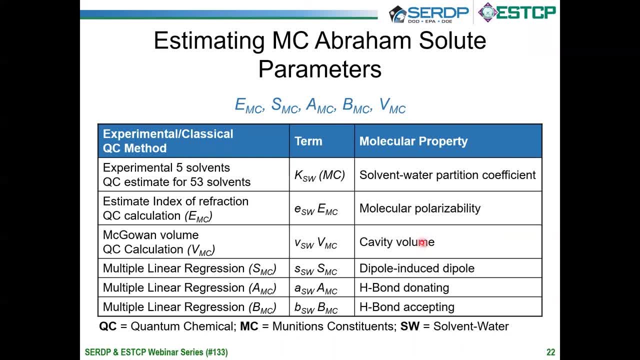 one deals with. The next one is the interaction having to do with the formation of a cavity. When you take a compound, for example RDX, and take it from octanol into water, you have to, you have to generate a cavity in water that's large enough to hold the molecule. 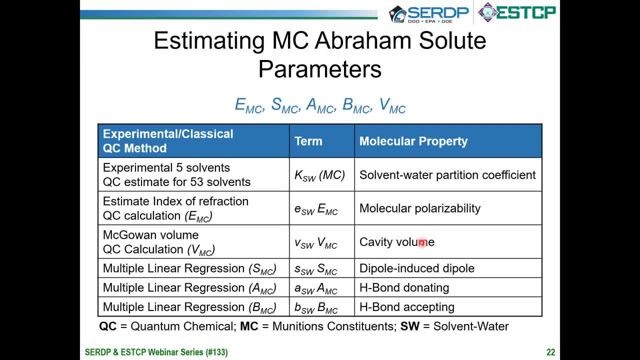 Water is a highly structured solvent. It's pretty close to a solid. The freezing point is not that far away from the laboratory temperature and as a consequence, it's strongly hydrogen bonded. It takes a lot of energy to punch a hole in water and, as a consequence, the volume term dominates, the so-called hydrophobic effect. 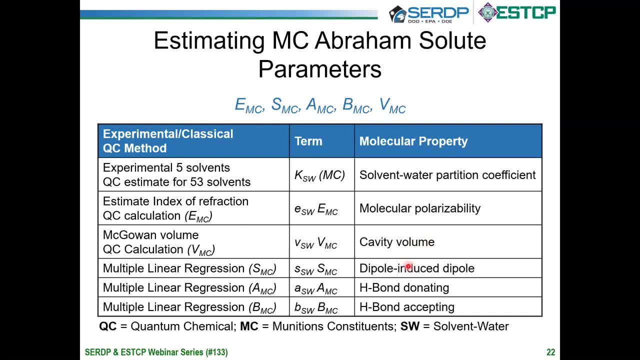 The next three are associated with other interactions. The dipole-induced dipole interaction: most molecules have a permanent dipole and if you take a permanent dipole and put it up against the molecule of the solvent that that can deform, you generate again an interaction and that dipole-induced dipole interaction causes an attraction. 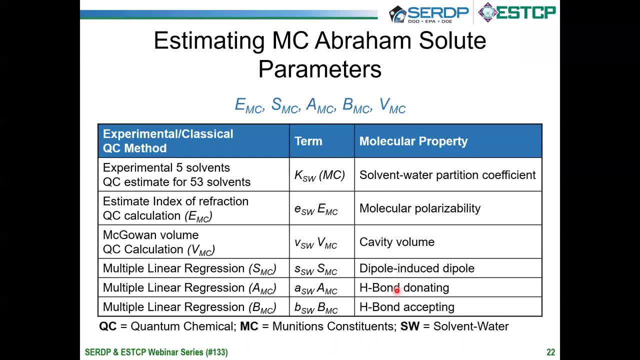 And finally, the two most most important, but certainly in many cases important, are the hydrogen bonding terms. Water is both a strong hydrogen bond donor and acceptor, and the solute if it can donate a hydrogen bond. so, for example, phenol, the hydrogen on the OH. 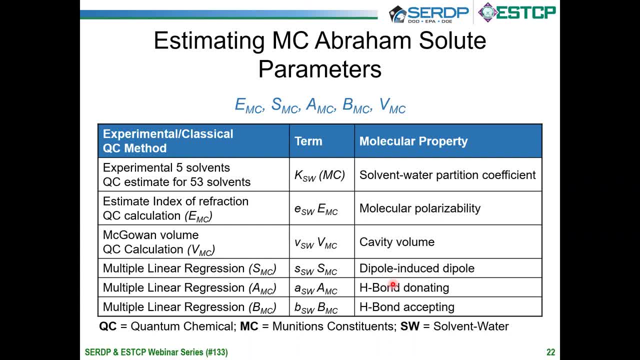 can donate a hydrogen bond and bond with the oxygen in water and form a relatively strong hydrogen bond. On the other hand, if, if the solute RDX has strong hydrogen bond accepting capabilities- partially negative atoms and nitrogen groups, for example- then the the solvent will interact with that and you will get a hydrogen bond accepting. 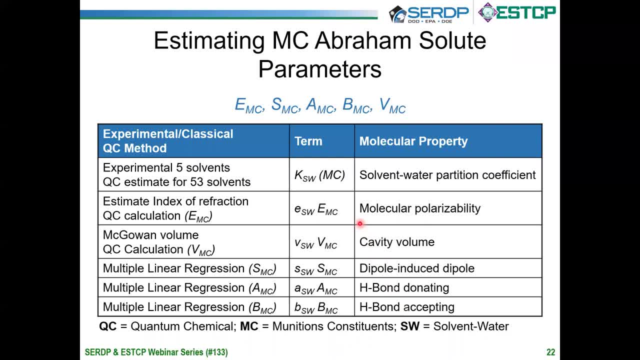 So notice the way the model is put together, Each of the terms in the model. they're not some unusual or not understandable term in a regression, the kinds of things that you see in in machine learning. These things are direct chemical interactions which are understood. 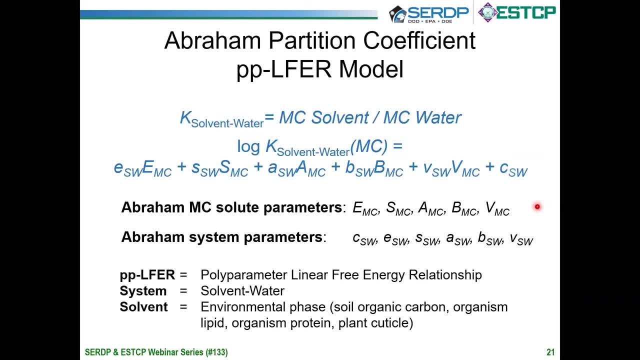 Okay, so how do I get the numbers to actually do this? The system parameters actually were the beginnings of this whole, this entire model, which were not developed by Michael Abraham initially, but his mentor, Mortimer Tamlett, who actually worked at the United States Naval Academy. 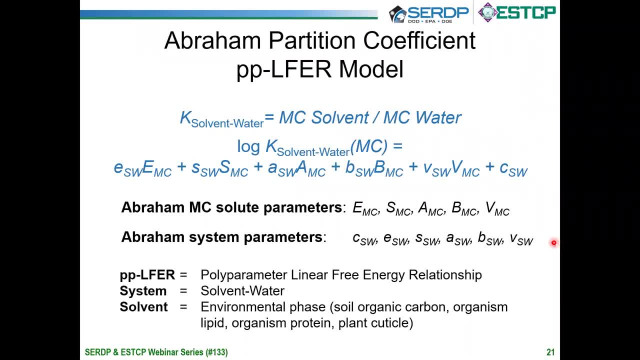 And he. he was interested in trying to figure out how solvents affect spectral shifts of various chemicals and came up with a system. what are now the system parameters? So these things pre-existed- The, the solute parameters, And Michael Abraham had the idea of trying out the same thing, using the system parameters as as characteristics of the solvent water system and then generating solute parameters for now the compounds of interest. 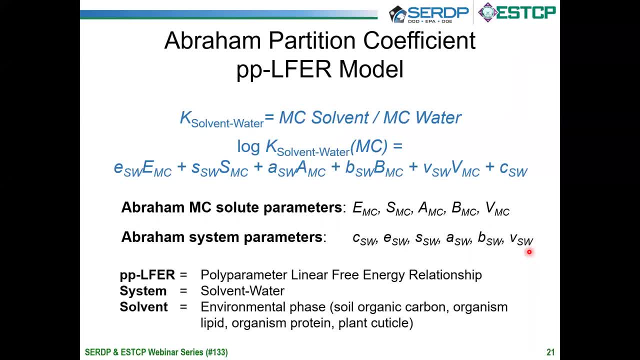 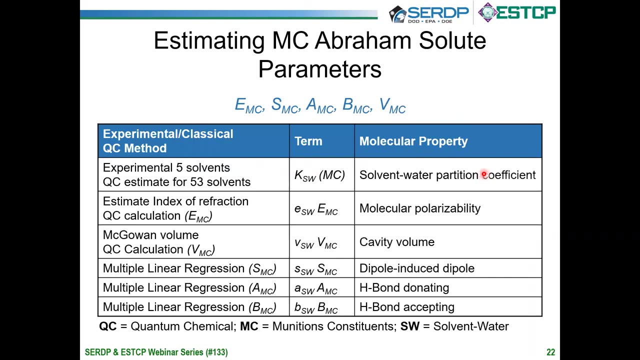 So, for example, RDX, And his idea was as follows: If we know the lowercase parameters, then these are a linear. you can solve for the, the solute parameters, the uppercase letters, by a linear regression. Here's how he did it. 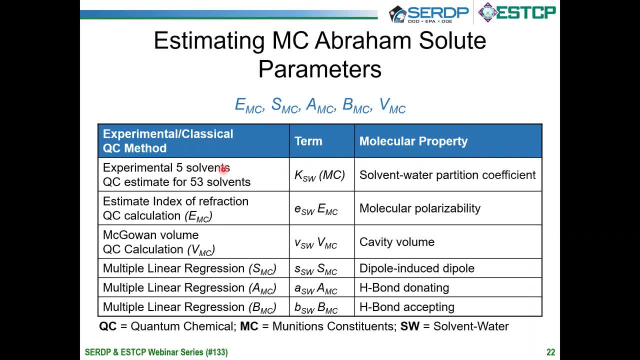 He said, actually it was some other workers that finally established the current method. But anyway, you, you, you experimentally measure the partition coefficient between RDX and five solvents: octanol, cyclohexane and so on. That gives you five data points. 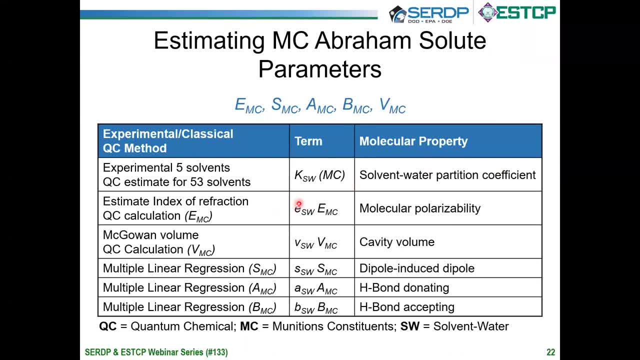 You estimate the index of refraction of RDX. That's difficult because this initially started off with solutes that were liquids And of course you could figure out what the index of refraction is for octanol, for example. So they have a method that is basically a fragment method to make that estimate. It's not very satisfactory, but anyway, that's how it's done. 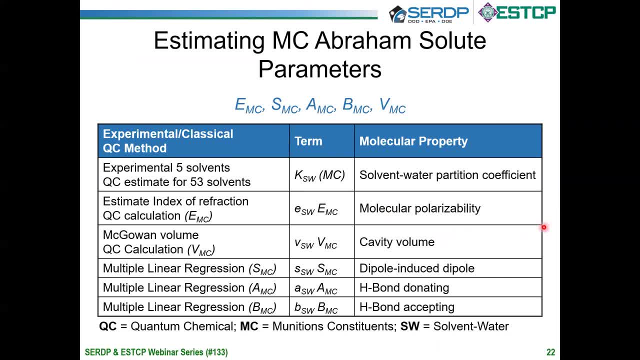 The cavity volume of the molecule is easy. There's a technique called a method called the McGowan volume, which is basically an atom and bond formulation which is very simple to apply and actually works very well. It's very close to to the more modern method that we use, And so you have then generated. 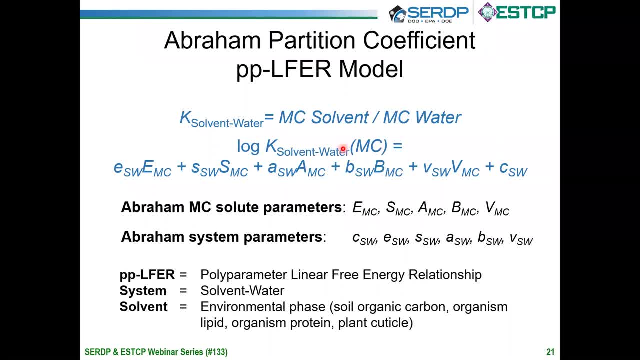 the following information: measured octanol water partition coefficients, for example, or organic carbon water partition coefficients. You've estimated the polarizability, you've estimated the volume, you know the constant. you bring the knowns to the left hand side of the equation and now you have a regression analysis in the dipole, induced dipole and hydrogen bonding solute terms. 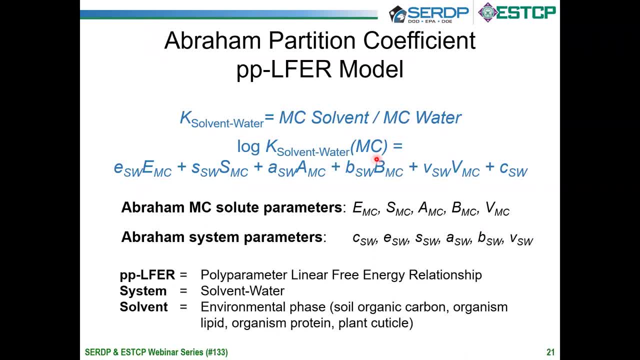 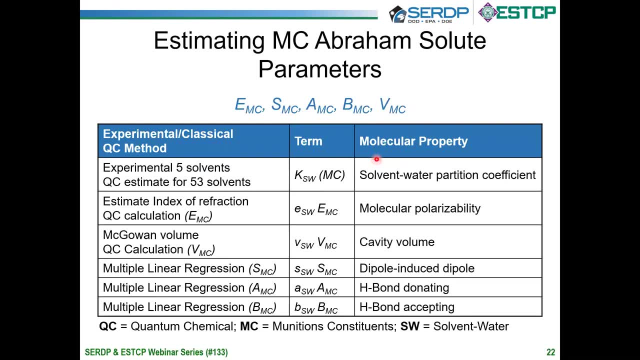 Three unknowns, five equations. It's a simple regression. The answer falls out. Our idea was to replace experimental solvent work water partition coefficients with quantum chemically calculated solvent water partition coefficients. Modern quantum chemical methods have relatively reliable solvent water modeling capabilities, but the primary difficulty is that they're not very accurate. 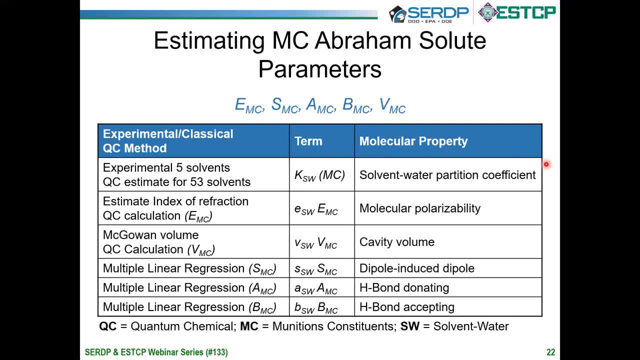 Quantum chemistry can make estimates of many things, but the accuracy is nowhere near the accuracy of experimental determination. So our idea was, instead of having five data points, let us calculate 53 data points. Let us calculate the solvent water partition coefficient for RDX in 53 solvents. 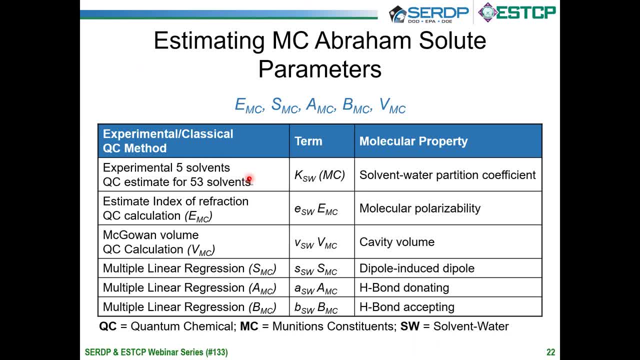 And those solvents were chosen because we know what system parameters are available- lots of them for the solvents- and we also know we have to match that with the solvents that the quantum chemical methods can calculate And the current method that we use are based on the Gaussian, which is the industry standard. 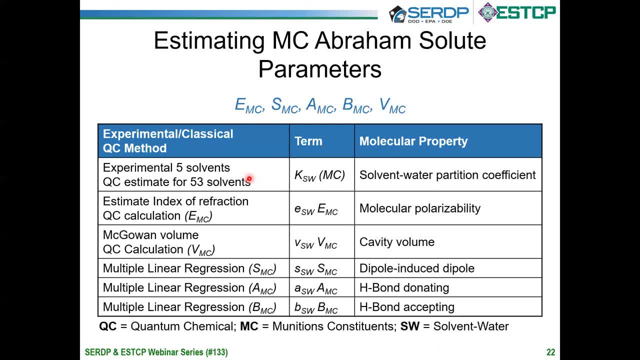 quantum chemistry program and they have roughly 50 solvents where that match is made. The only other important contribution was to calculate the uppercase E from molecular the index of refraction, to calculate it directly from a quantum chemical. calculation of molecular polarizability. 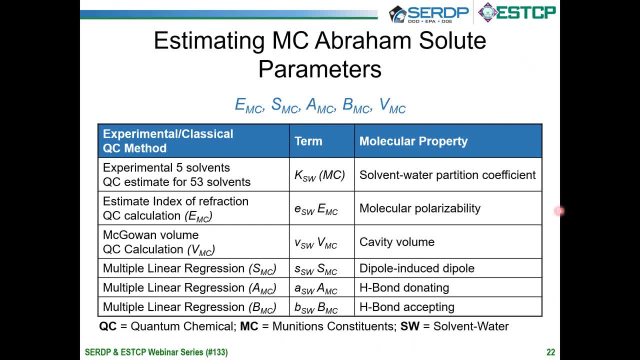 That is a standard calculation and there's an equation that relates molecular polarizability to the index of refraction and that then solves the problem of how do you get the index of refraction for a solid. Basically, you just calculate the molecular polarizability in the gas phase and apply the formula. 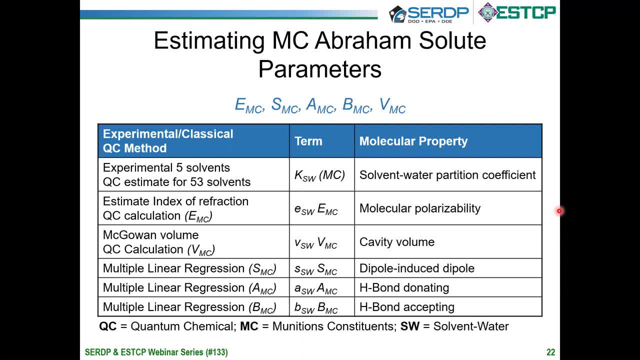 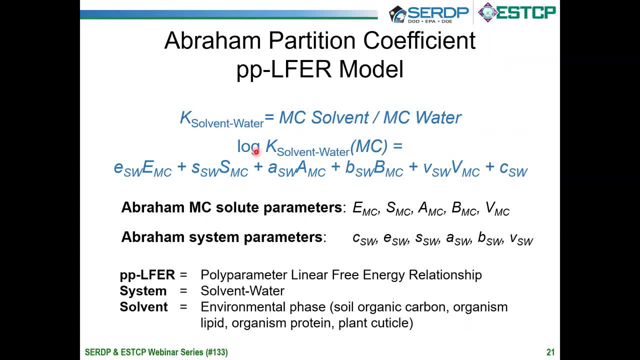 The rest is exactly what follows how the experimental techniques work. So now you have a regression analysis. You have not five solvent water partition coefficients, but 53, and you're estimating three parameters. and that's how we do it. So that is the method, the quantum chemical method, that we use for Abraham: estimating Abraham partition coefficients. 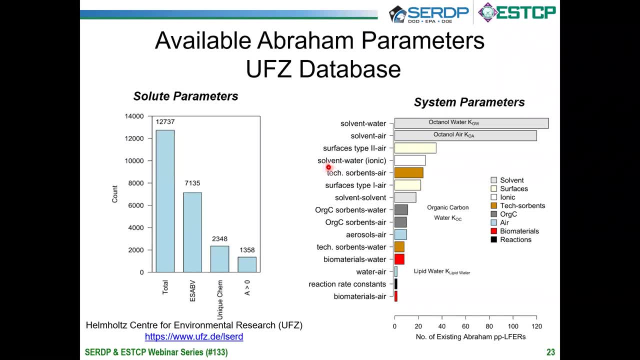 This model has been around a long time and, as a consequence, there is quite a lot of information that's available from a database that was called the UFZ database, and it's at the Helmholtz Center for Environmental Research in Leipzig. 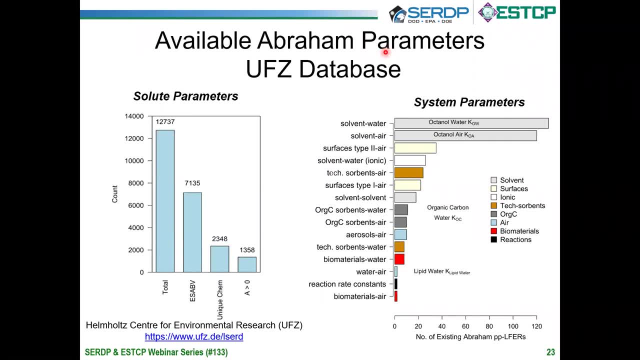 The website is at the bottom of the slide And if you do a global download, which you can do- of all the solute parameters that are there, there are essentially 12,000 parameters that are available, of which 7,000 roughly are. 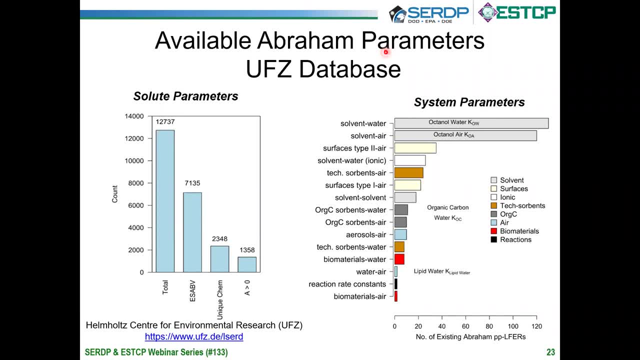 the ESABVs, the parameters that we use, where the cavity volume term is one of the parameters. If you ask yourself how many unique chemicals there are, there are about 2,300 unique compounds for which there are solute parameters. Now, not all of these are experimental measurements. 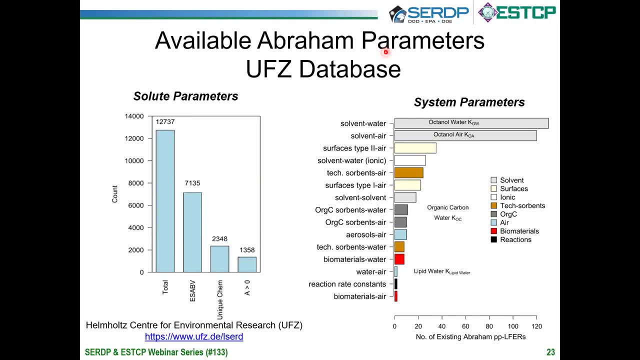 A lot of these are determined by estimation techniques And if you're curious about what's there in terms of molecular properties, about half of them actually can donate hydrogen bonds. So that's interesting. On the system parameter side, which is really what you care about, because the only reason you want Abraham parameters is to join them up with the system parameters for a particular system that you're interested in- 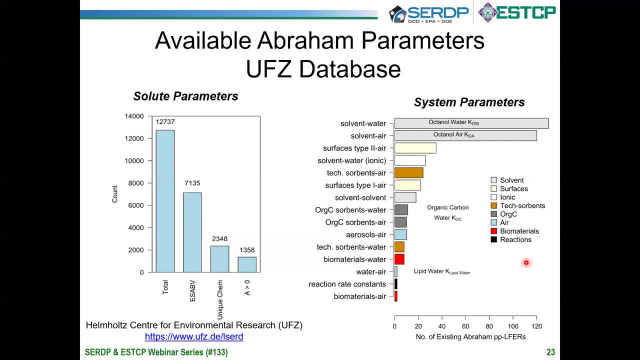 So there are about 120, 130 solvent water partition coefficients, of which octanol, of course, is one of them. There are solvent air partition coefficient of octanol air. There are surfaces, There are sorbents of various types. 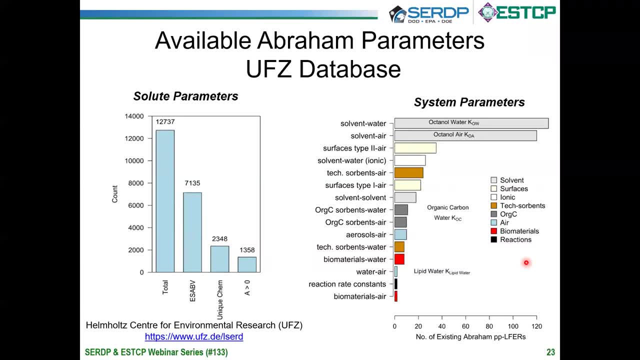 There is organic carbon, There are aerosols, There is a lipid water partition coefficient, And all of them are designed to work in parallel with the solute parameters. So if you have a solute parameter set, you can then calculate the partition coefficient. 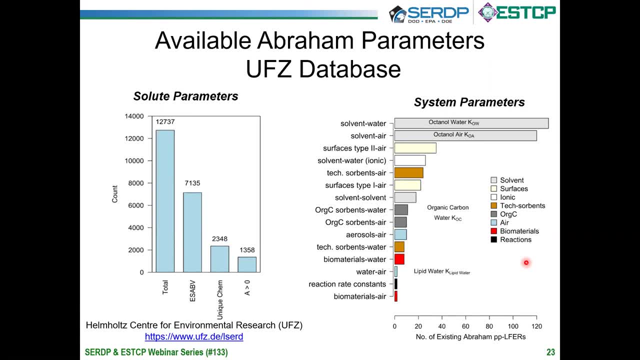 for any one of these systems. That's the power of the method: That once you've spent the effort to get the Abraham solute parameters for RDX, you can calculate what is the partition coefficient of RDX with all of these solvents and systems. 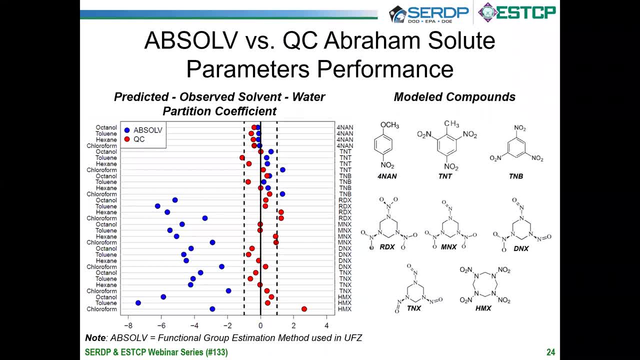 Well, how well does it work? The we for the for this, the CERTA project, where we developed this initially, we made some measurements of the partition coefficients of some MCs, in particular RDX and its friends HMX, and a few others for NAN. 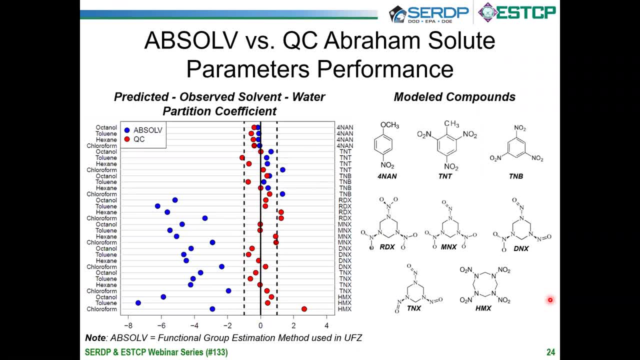 And we compared the predicted versus the observed solvent water partition coefficients for the solvents listed on the left-hand side of the of the figure and the solutes on the right-hand side. The blue dots are absolve predictions. Absolve makes predictions using functional decomposition. 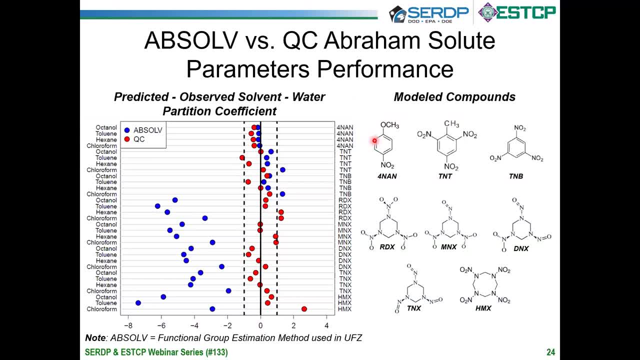 It just takes apart the molecule. It says, well, I have a benzene ring, Okay, it's, it's. it's functional group is a methoxy group that adds so much energy. There's a nitro group at another position that adds so much energy, and so on. 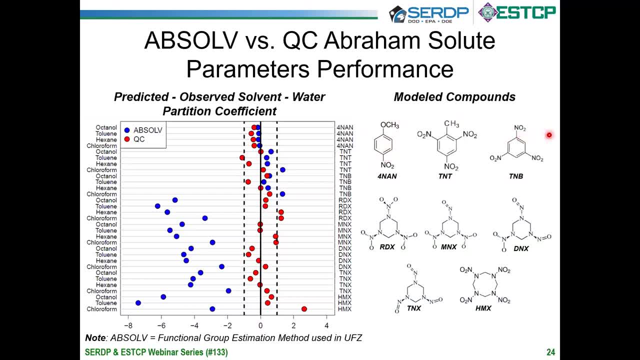 So it doesn't. it just uses essentially the configuration And you can see that for some of the compounds it does about as well as the quantum chemical method does, which is estimate the partitioning in 53 solvents and so on. But when you get to RDX and its friends, suddenly it just falls apart dramatically. 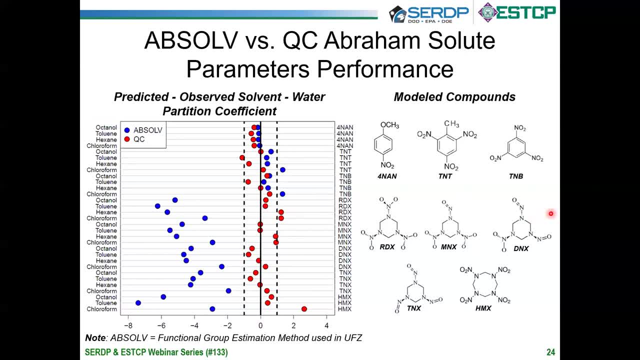 And the reason is that it is built on fragments that have been established from experimental data, And it turns out that absolve doesn't know about the NN group between the heterocycle and the nitro group, But it doesn't bother to tell you that it doesn't know. 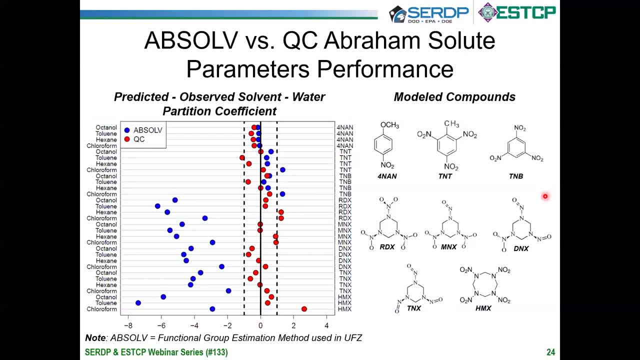 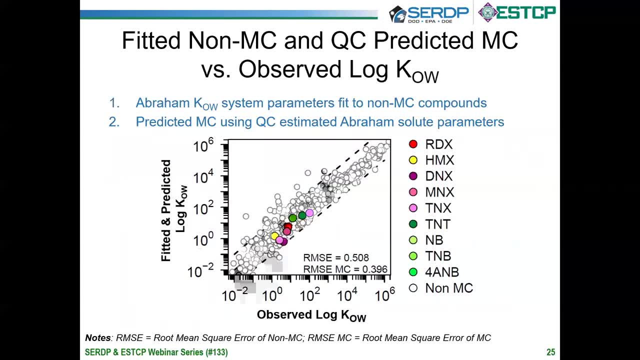 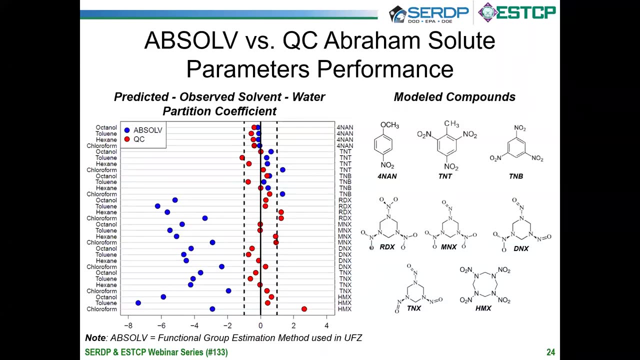 It just gives you wrong answers. So that's very disturbing, And the problem with it is that it's a black box, A number comes out and that's it So so it looks like the quantum chemical methods are okay. I remind you that we don't use any experimental data to generate the Abraham parameters for molecules. 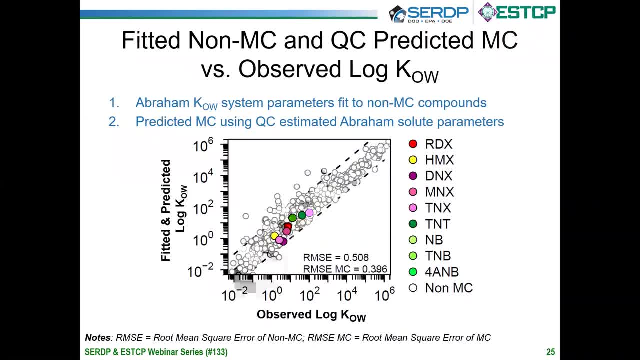 We just use the molecular structure and quantum chemical calculation. Well, how well does it go? Here's an example of the prediction of the optimal water partition coefficients for these munition constituents. What's plotted here is on the y-axis is the fitted versus observed log KOW from which the system parameters were obtained. 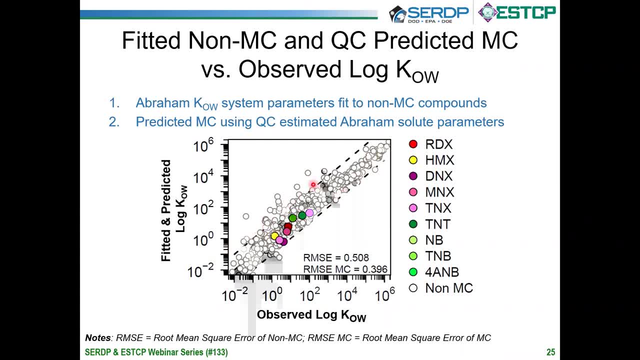 So of course this just shows that the system can reproduce the numbers that you use to get the system parameters. Of course you have to have the solute parameters as well. So what we did was just take the solute parameters that we calculated for the munition constituents and just make a flat out prediction. 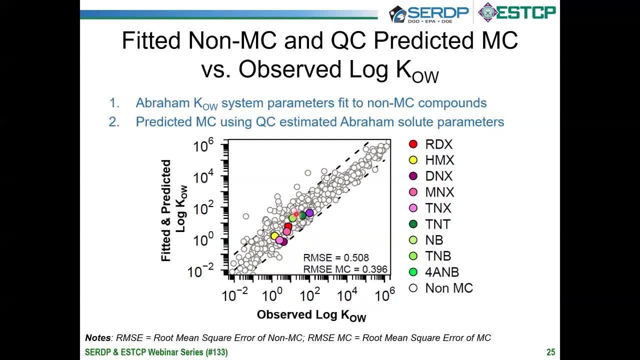 That's the colored dots. I remind you that the system parameters have never seen munition constituents, So this is a flat out prediction. You can see that the root mean square is typically about 0.5, is 0.5 for all of the unfilled circle. 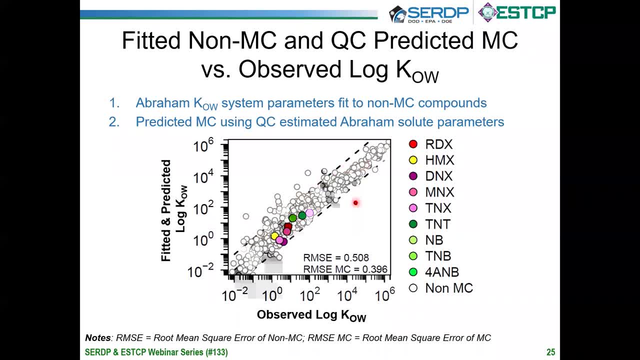 That's all the data that was used to set that up The system parameters. When we ask how well it predicts the munition constituents, it gets a root mean square of about 0.4.. These are typical ranges of the accuracy. It's the same situation for log AOC. 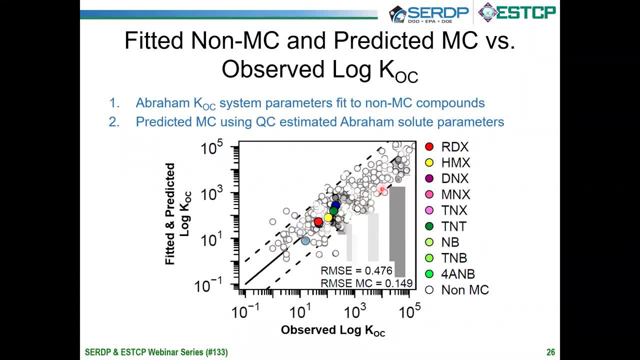 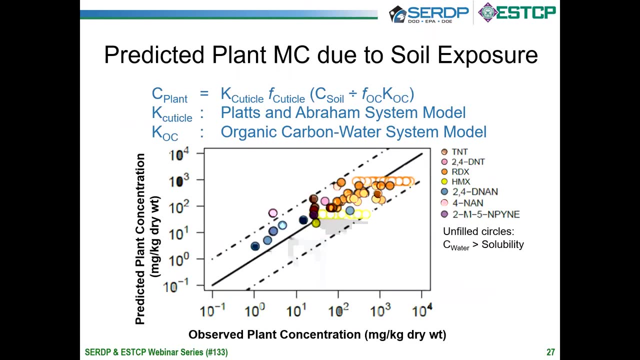 Same thing. The unfilled circles are the data used to get the system parameters. The colored data are predicted. Here it did remarkably well, almost too well. Here's a more stringent test. I'd like to predict plant concentration. These are grasses that we grew in the SIRTA project. 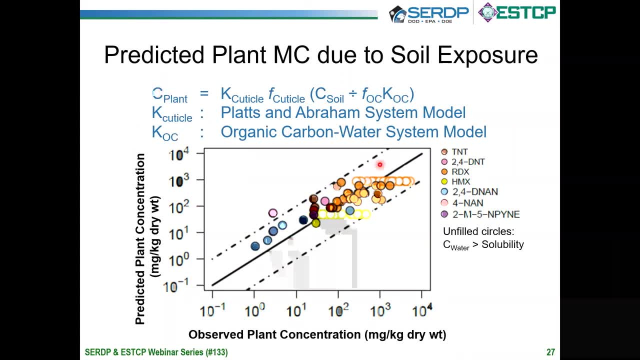 I'd like to predict the concentration in the plant from the soil concentration that was measured. So, soil to plant. In order to do that, you need a partition coefficient between the soil and water, And then you need a partition coefficient between the plant, water and soil. 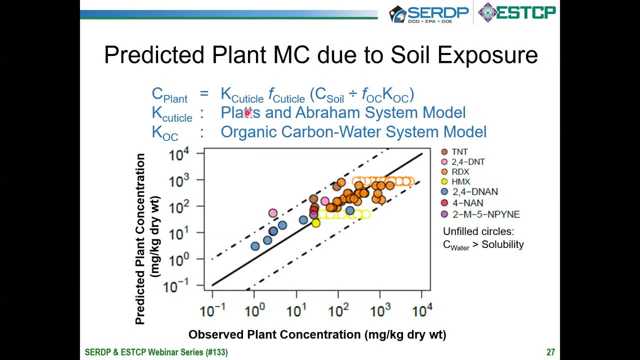 And the plant cuticle. These system parameters were gotten from, in one case, published data that was done by Platt and Abraham, And in the second, the KOC model that I just presented. And here's the equation And you can see this is the observed plant concentration. 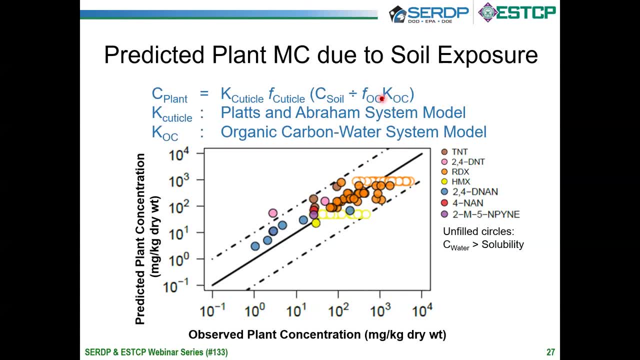 And this is the predicted plant concentration. Now, none of these systems have ever seen munitions constituents. And here's the compounds that we had data for This, The unfilled circles, by the way, those horizontal lines are a data set that were in the literature where the exposures exceeded the solubility of the compound. 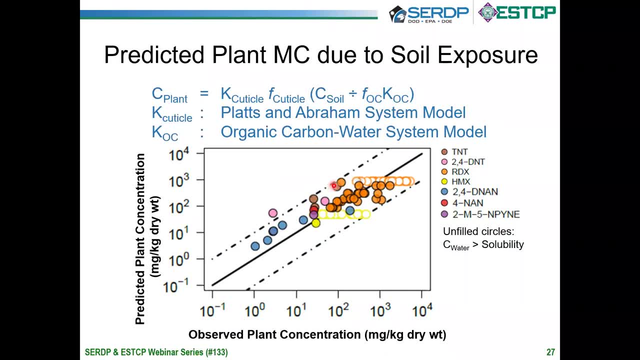 And so what we do in that case is we just use the calculated solubility as the predicted water concentration, And that's why they're constant. Again, you can see, within All the lines, by the way, are order of magnitude differences. 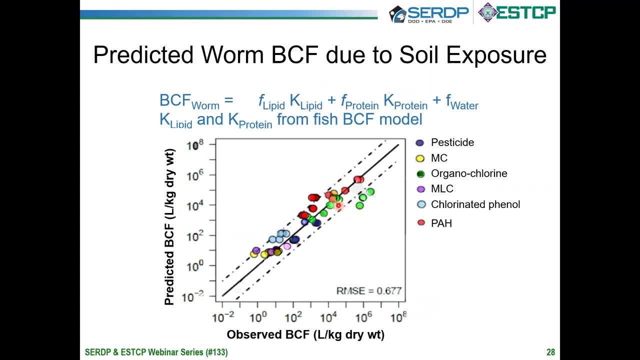 You can see that we can do a reasonable job. Finally, here's the same thing for worms. We did a prediction for the bioconcentration of acinia and earthworm in contaminated soils, And the way we did it was using partition coefficient from a fish bioconcentration model. 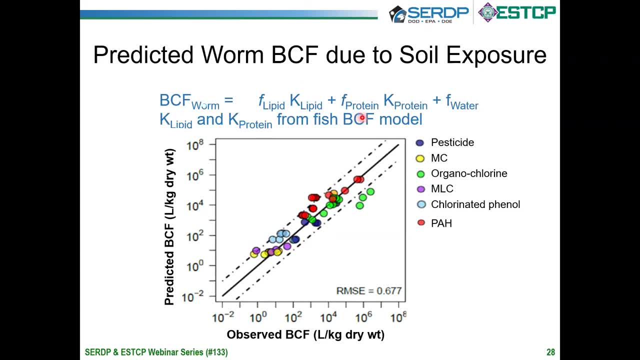 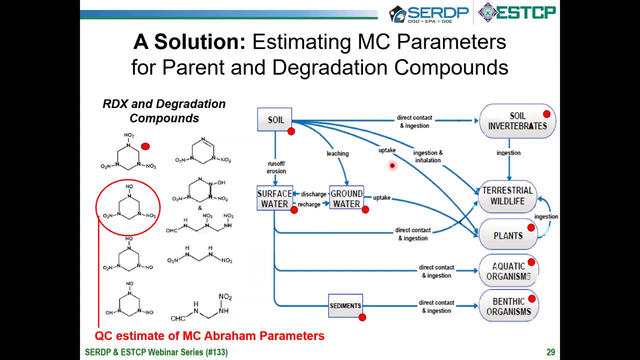 So it had never seen any of the munition constituents. And we get about the same kind of behavior. So I think you can see that, If you need to calculate what's going to happen to a degradation product, what you simply simply 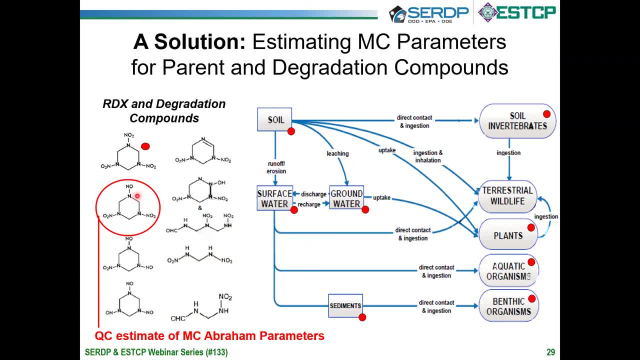 What you need to do is to calculate the Abraham parameters for the molecular structure. Once you have the solute Abraham parameters, you've got it for all of the other phases in which you have to make predictions. So it is a very efficient method once you know how to do the prediction. 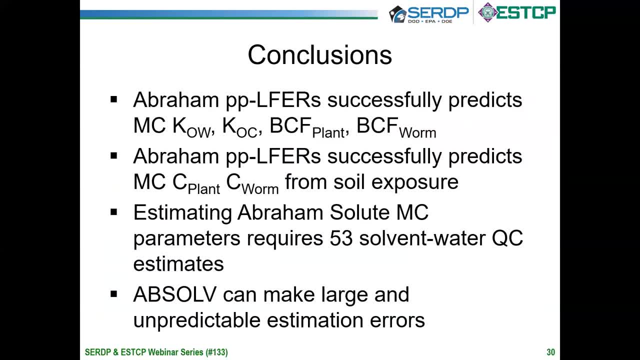 So, to conclude, I think you can see that it's successful. It successfully predicts partition coefficients. It, more importantly, successfully predicts the concentration in the end targets in the plants or in the worms, And it predicts it from soil exposure, which is exactly what you need to do in any kind of risk assessment. 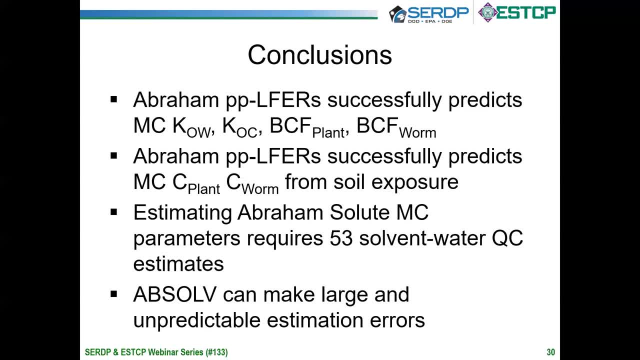 Of course you need 53 roughly solvent water quantum chemical estimates of solvent water partitioning. That's the difficult part, And it clearly is better than ABSOL, because these functional decomposition methods can make errors and you just don't know why they're breaking. 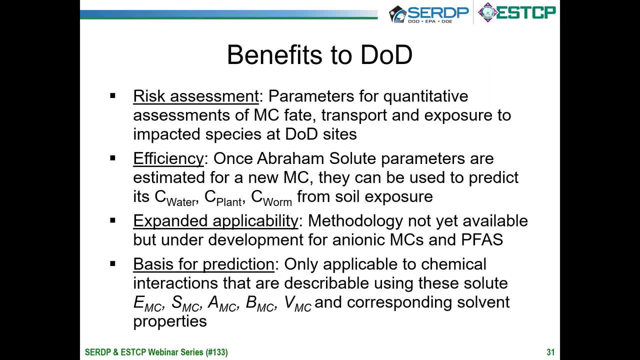 So, finally, if you're going to do risk assessments, you've got to have partition coefficients, And the Abraham method, using quantum chemical calculations, is very efficient, because once you've got it for a new munition constituents, you're there, You can make the calculations for anything. 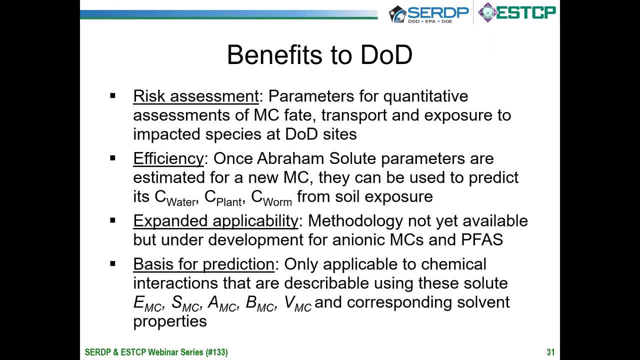 You can make the calculations for any of the partitioning systems that you have constants. for A couple of difficulties, The methodology is not yet available for anionic munition constituents, for example NTO and the currently being investigated- the fluorinated materials. 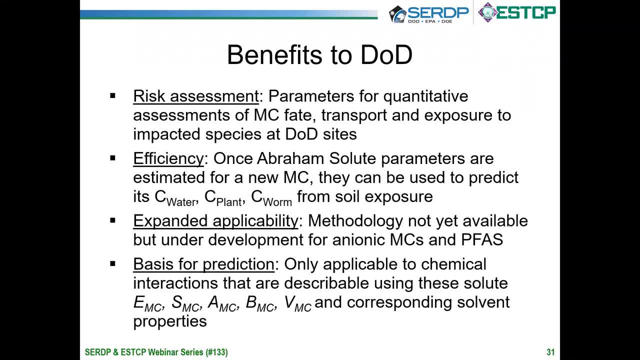 We can discuss where that is and what's going on. And finally, you should understand that this is not a universal tool. It will only make a reasonable estimate for interactions that are describable by the five molecular mechanisms that it knows about. So, for example, if something odd is happening, there's a steric inhibition, the protein has a specific binding site that isn't just hydrogen bonding. it will fail. 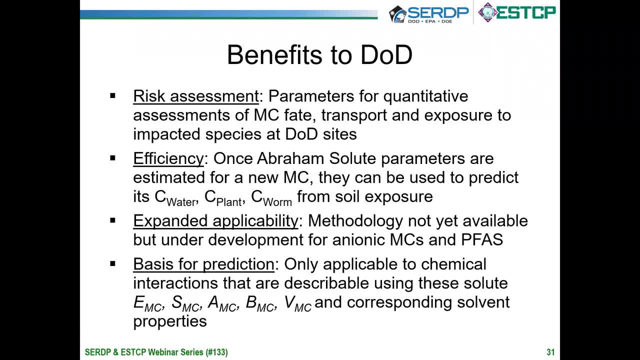 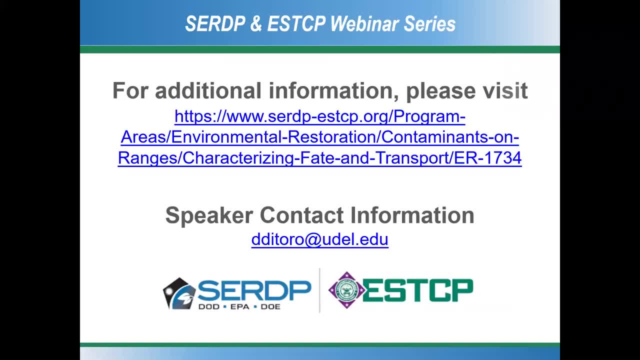 It will not. it may do a reasonable job, but it is certainly not getting at exactly the chemistry. One final comment, And that is: it is very important when you're doing quantum chemistry to have at least one or two real measurements. It is very easy- I tell you from experience, it is very easy- to get wrong answers. 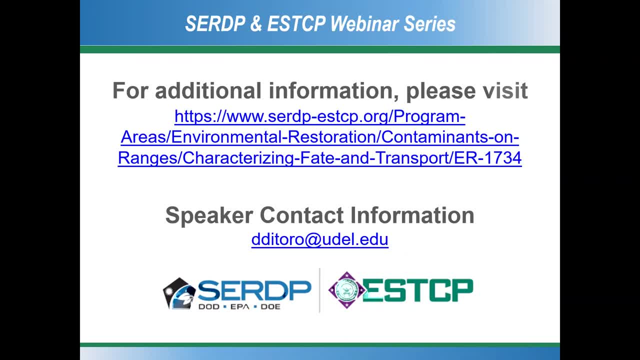 And because it is a difficult calculation that you've got to get right. So you need at least one number of octanol water partition coefficient, or something for a chemical that's like it, Just to be sure that everything is right. Okay. So thank you and I look forward to your questions. 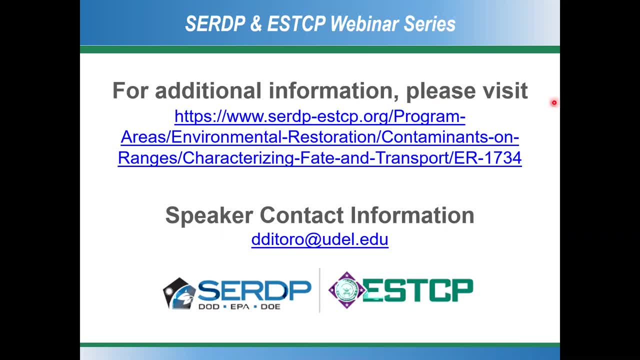 Wonderful. Thank you, Dom. At this time, I would like to remind the audience to submit your questions using the question and answer box at the on the zoom screen, if you hover over the zoom menu. We have received our first question today from EPA. 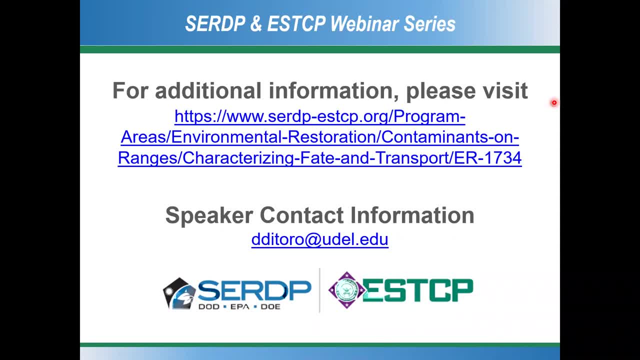 The question is: given that most explosives are solid That ambient temperatures, Does this model or approach inform the prediction of solid to liquid dissolution kinetics for things like RDX or TNT? The Abraham model doesn't do kinetics. It can be used to make some calculations which might help in formulating models for kinetics. 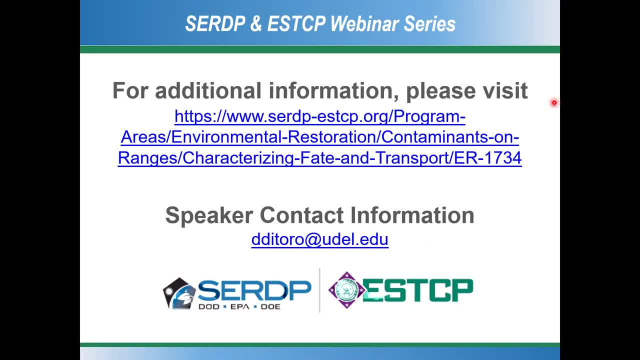 But it certainly will do the solubility problem Because in fact it knows. It knows about the molecular configurations and there are system parameters for solubility. That is not a simple problem, by the way, Because it is not basically a solvent water interaction. 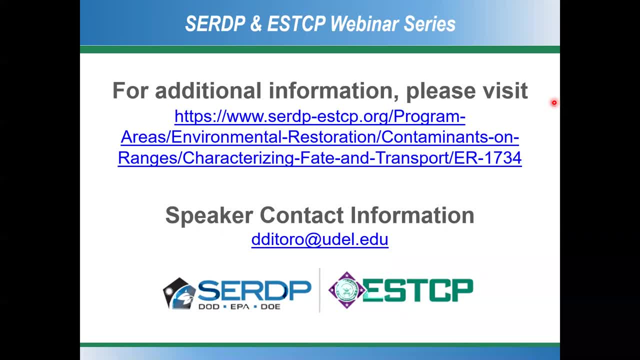 Okay, Thank you, And can you place your approach In the background or amongst the variety of quantum chemical methods? How does your method differ from other methods? That is a good question. There are essentially two other methods or two other classes of methods that use quantum chemistry. 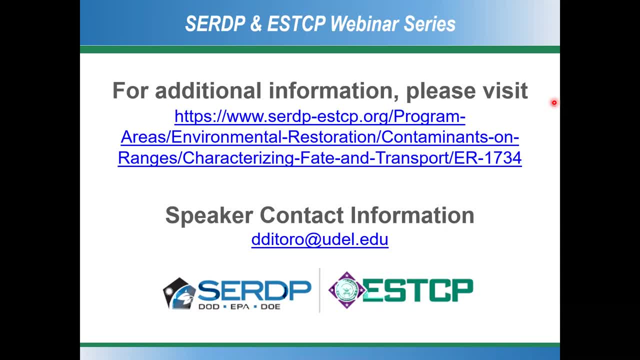 The first is a method that uses the Cosmo theorem, The computational technique. What they do is they use moments of the electron distribution And have a regression that correlates to the moments of the electron distribution. So they are not focusing on chemical interactions. 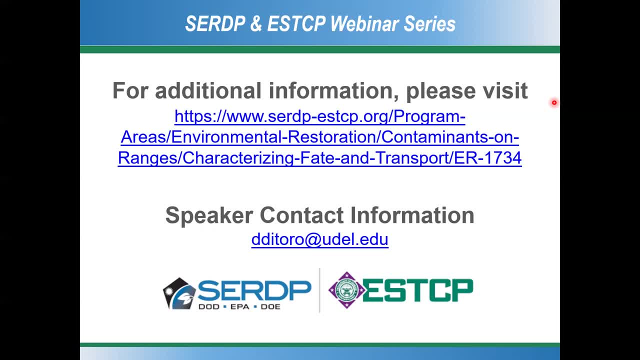 They are using a regression method And so if it breaks you are not sure why it broke. The others, which are the majority of methods. what they normally do is they will calculate 100 or so quantum chemically derived molecular properties And then they will apply regression analysis to the data that they have got. 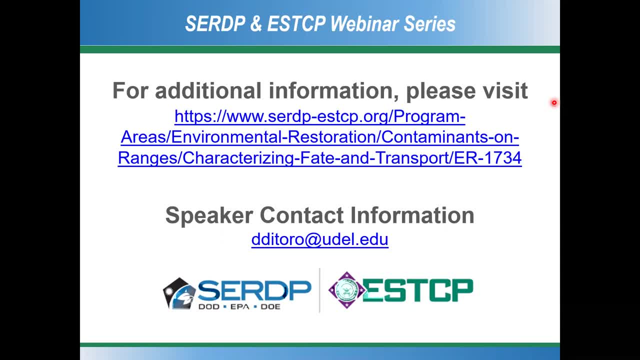 The experimental data that they have got And then establish a regression model. Again, the problem is you don't know why it picked the parameters that it picked. It just did And, as a consequence, if the thing doesn't work, you don't know where to go next. 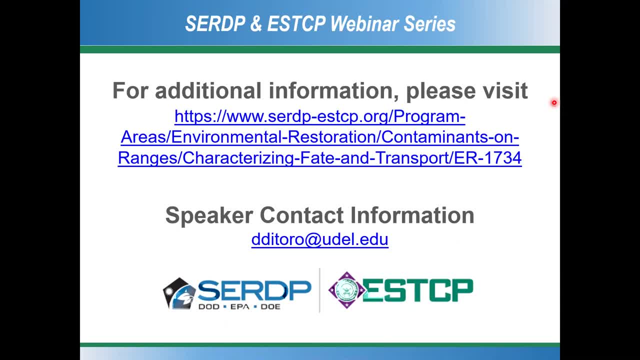 And the reason we chose the Abraham model is that it is set up in a chemically sensible and interpretable way. It is very mechanistic, Or as mechanistic as you can get in this kind of a calculation, And that is the reason for the choice. 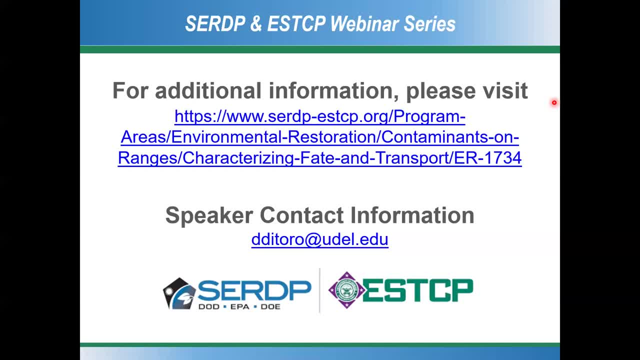 Okay, Great, And we have received a couple of questions about the failure of the predictions. So how do you evaluate prediction failures using the Abraham model? And then, what is the next step if the prediction is not correct? Yeah, That is a good question. 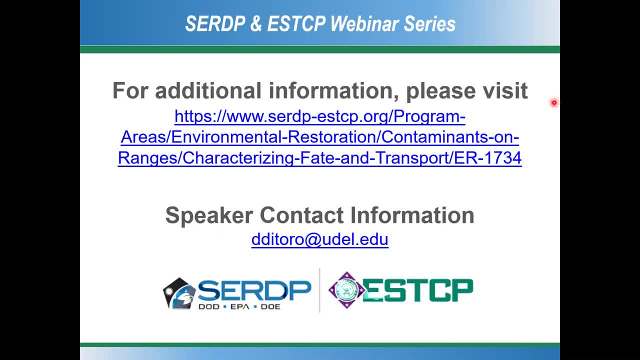 You know from the history of Abraham parameters that have been estimated for all the solutes that are in the UFZ database. you have a good idea of the range of, for example, hydrogen bond donating and accepting capability, molecular polarizability and so on. 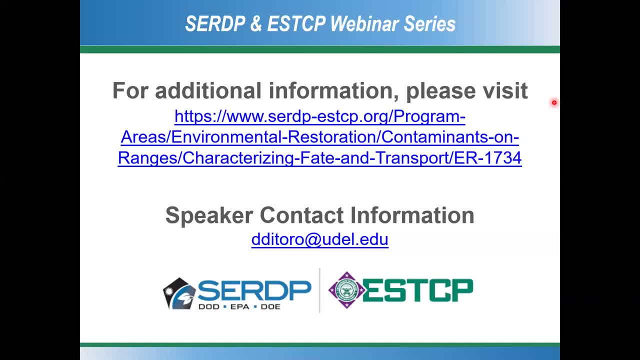 So you can examine what your quantum chemical calculations gave you for those five solute parameters and see if they are looking strange. That is the first thing. The second thing is you can, and I strongly recommend that, if you need these parameters for a real risk assessment. 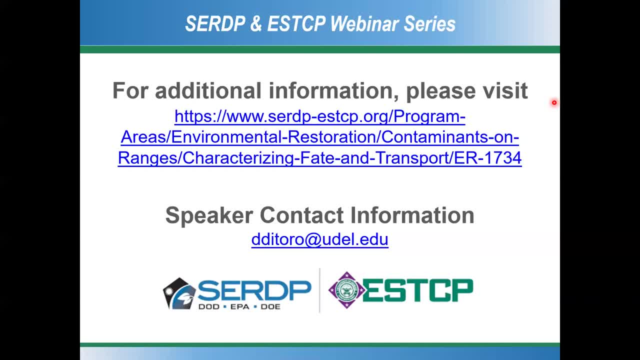 that you invest in at least one or two solvent water measurements. Those are fairly straightforward nowadays- Well, not for PFASs, unfortunately- But at least have one or two data sets where you can check And if the thing is not working then you can figure out. Your normal, by the way. Your normal assumption is that there is something went wrong in the quantum chemistry, And usually the problem is conformers. You may not have the molecular structure right, Especially in complicated molecules, caged molecules, for example. There are lots of structures that are close, But if they are off by a kcal or two, that is enough to foul up the partitioning calculations. So you have got a next step, which is what is going into the calculation, namely the computational chemistry part. 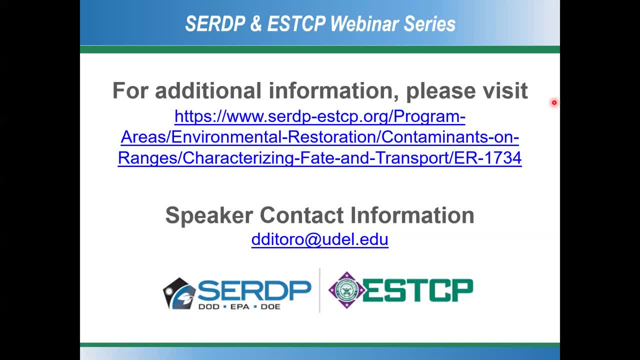 Are you following the rules that are required? And secondly, are there conformers that you have to worry about where the methyl group has to rotate the other way? That sort of thing, Okay, Thank you, Dom. Can the Abraham model be corrected for temperature? 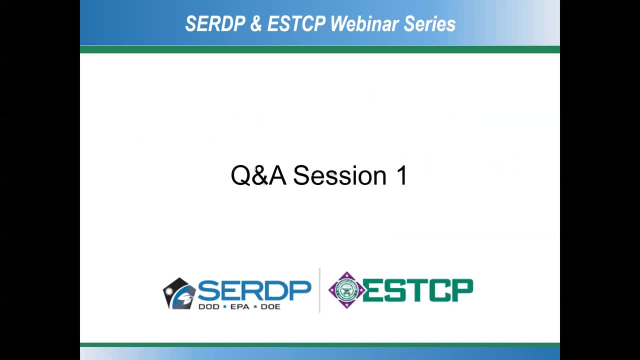 That is a good question. Well, if you know the enthalpy of the reaction, there is actually, if memory serves, system parameters for an enthalpy correction. That has been worked out for certain solvents. But basically it amounts to: do you know the enthalpy of the reaction? 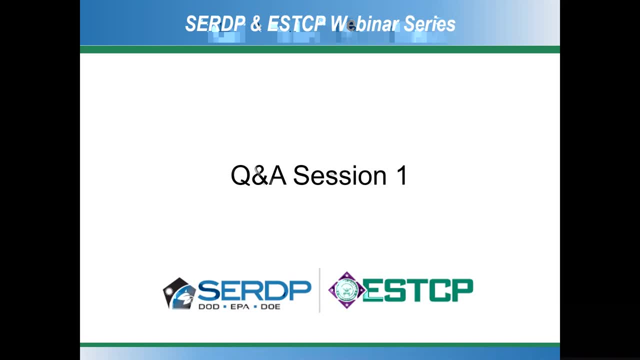 It cannot calculate enthalpies. You would have to actually look at that directly. It is an interesting question. I do remember that there is a system parameter or two for the enthalpy correction. Okay Great, Is your approach related to machine learning methods, or can machine learning be used with the basic approach that you have described? 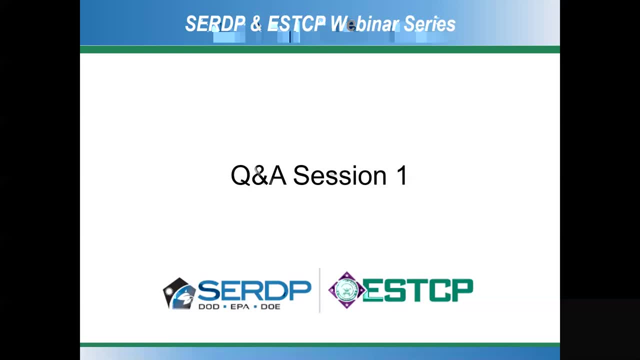 It is about as far away from machine learning as I can imagine. The way machine learning works is that you have a very large data set, hundreds of observations of partition coefficients, And then it looks for regressions, Complicated, perhaps nonlinear regressions, that relate these hundred or so parameters that you have gotten from quantum chemical calculations. 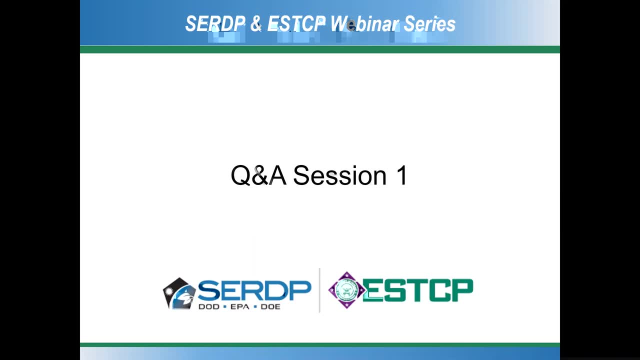 Or intuited from structure, topological indices, graph, all kinds of stuff, And then it makes a regression analysis and generates a prediction for the partition. Well, first you have to calibrate it And you can understand that that is a fairly blind black box kind of a method. 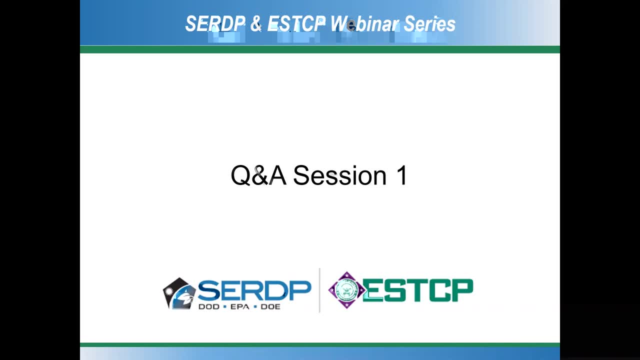 You just don't know why it is doing what it is doing. So, in the sense that regressions are utilized, yes, both of the methods use regressions, But I point out to you that in the Abraham model, the regression only estimates three parameters. 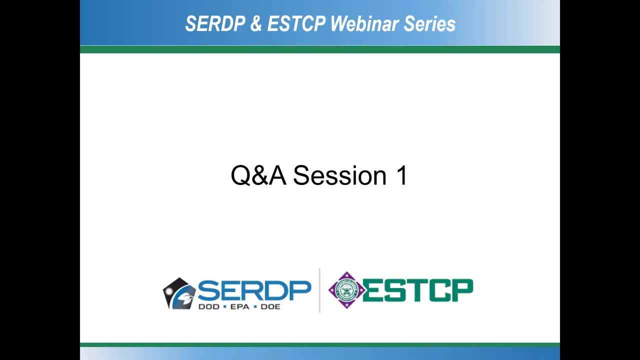 And, as a consequence, it is a lot less subject to regression difficulties and nonunique regression equations and so on. I am afraid I am not a fan of machine learning, because if you have a problem, you need a solution to it. If you have a problem, you need a solution to. 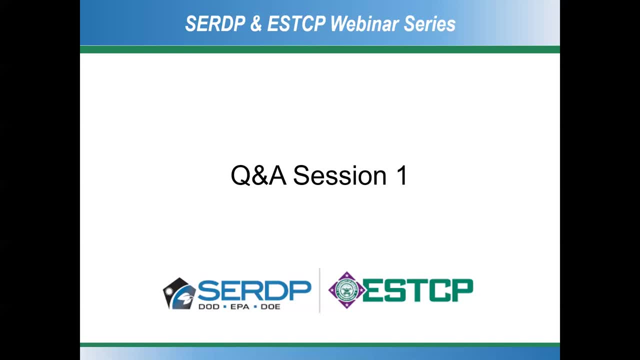 You then generate a machine learning based algorithm. And now, but you don't understand it because it just gives you numbers out of a black box. So you start off with one problem: You don't know the partition coefficient. You now have two problems. 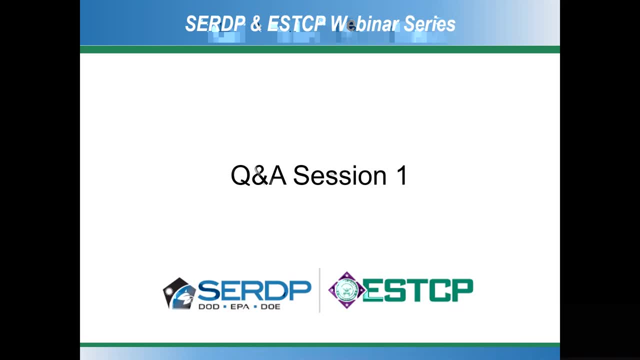 You have a model that you don't understand either. So it is, I think, the polar opposite, frankly, of machine learning. You can see I have a bias in this subject Understood. The next question has to do with biological transformations. 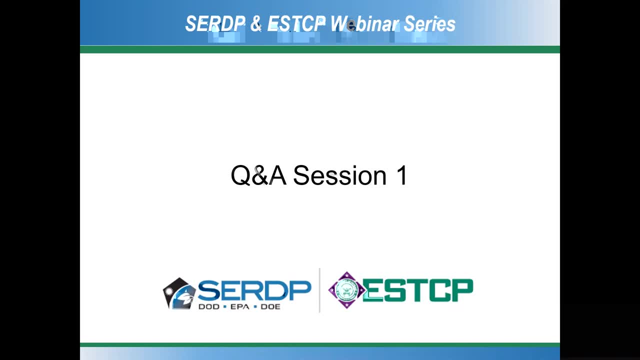 Can this approach describe biological transformations like TNT to the amino DNTs, Or can it, at least you know, describe the potential biological reactions that would be possible? Yeah, that's a good question. The short answer is no. The Partitioning calculations are equilibrium calculations. 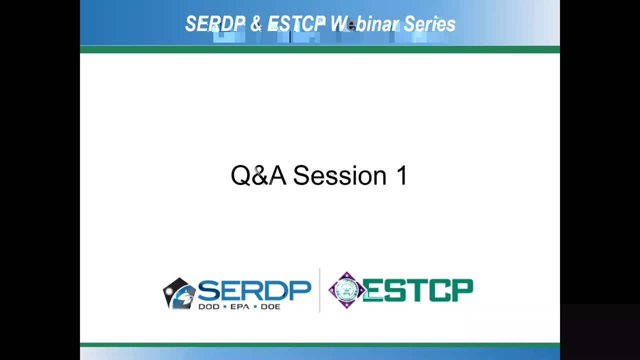 They're essentially thermodynamic equilibrium. It's the same kind of an understanding that the partition coefficients are linearly related to the formation free energies of the components. So it's really an equilibrium kind of a calculation. It can tell you what would be the concentration in organism lipid, organism protein. 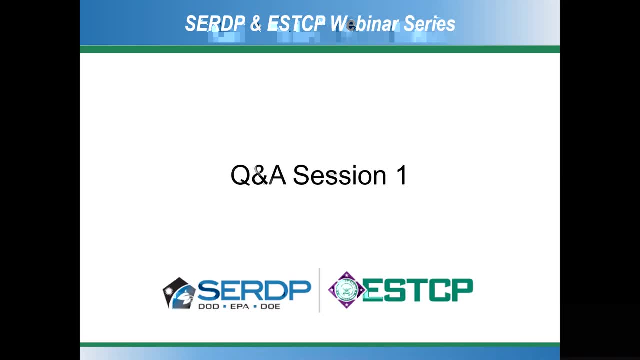 If you have a system parameter for an enzyme, for example, it could tell you how strongly it binds to an enzyme. The protein system parameters we have are for albumin. Well, you could generate if there's an awful lot of data out there. 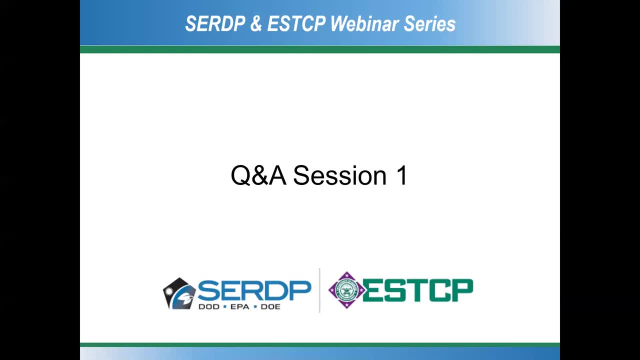 you could generate the partition coefficients to the enzyme that then does the reduction, So the degradation. So yeah, that would be interesting. actually, but not not specifically. I don't know of any direct attack. OK, thank you. What is the typical relative error? 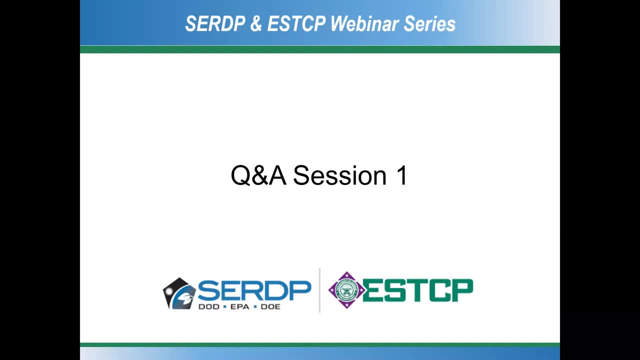 For example, the mean between the calculated and the empirically observed partition coefficients for munitions constituents. Do you have that? Yes, that's a good question, Because the well, in the first place, the root mean square error accounts for both the bias and the and the scatter as well. 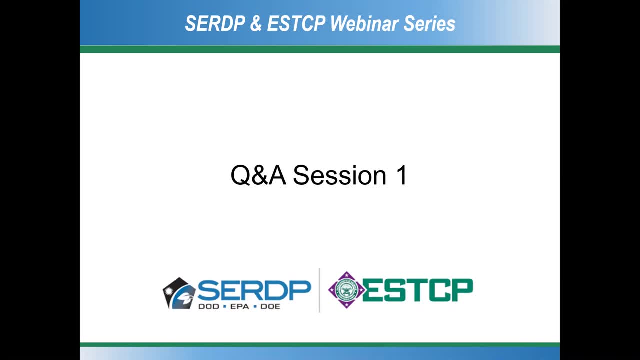 So it is not a variance, It's. if you think about it. it's the sum of the variance plus the mean squared And that number typically in a good model is 0.3.. In an OK model is about 0.5.. 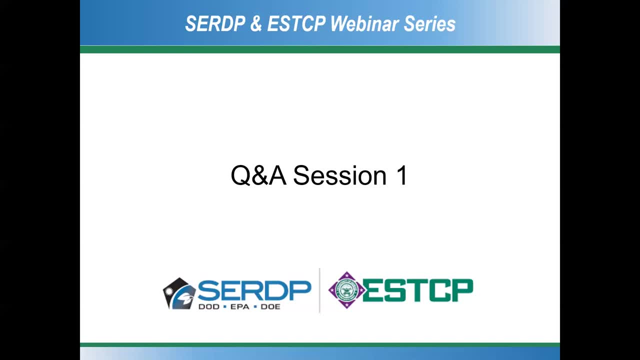 And when you start exceeding up to 0.6 or 0.7,, you're beginning to get a fair amount of scatter outside an order of magnitude. You should understand that none of these methods are anywhere as precise as chemical determinations. They are not. 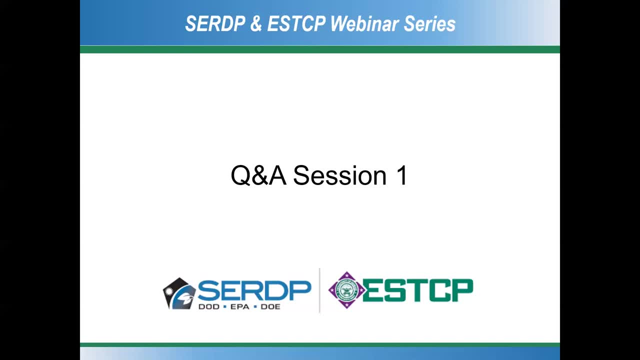 And in fact in the history of quantum chemistry it was suspected for a long time that it would be of no use to anyone ever. That, fortunately, is not the case. And but? but it is not a replacement for direct experimental capabilities. Something like you'll certainly get most of the time within an order of magnitude. 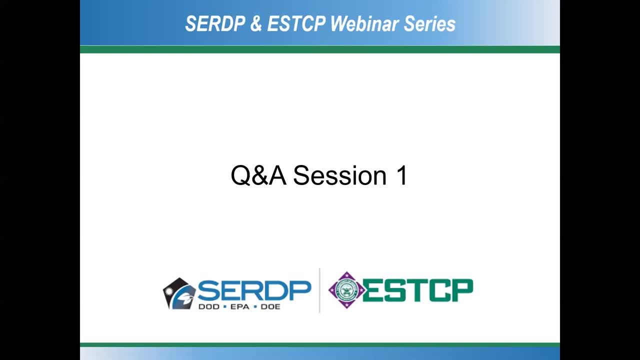 That's almost guaranteed, And you'll probably get, within you know, three tenths of a log unit In fairly well studied and well understood systems. OK, thank you, Dom. we have one final question for you in this session, And that relates to how the members of the audience might be able to use this approach. 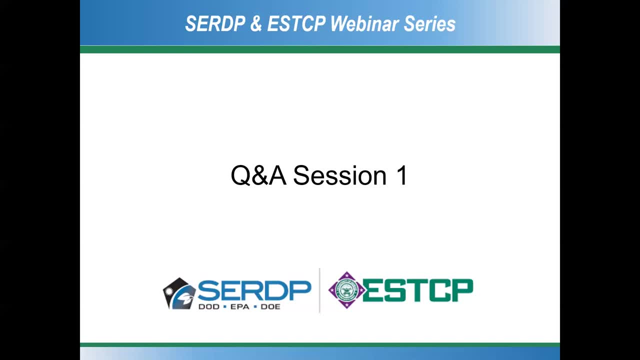 Will there be software of the approach or a tool available for use at DoD sites? Can you describe how Practitioners might be able to use this? Yeah, The method that we used in the SIRTA project that I've described used a solvation model which is not not readily available. 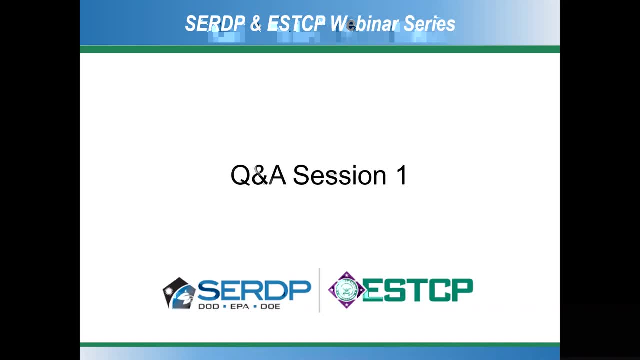 The method that we're developing now under the current SIRTA project uses Gaussian, which is the industry standard quantum chemical calculator. Gaussian 09 or Gaussian 16 are the standard Methods. You can learn to do quantum chemistry on your own. It takes some doing. 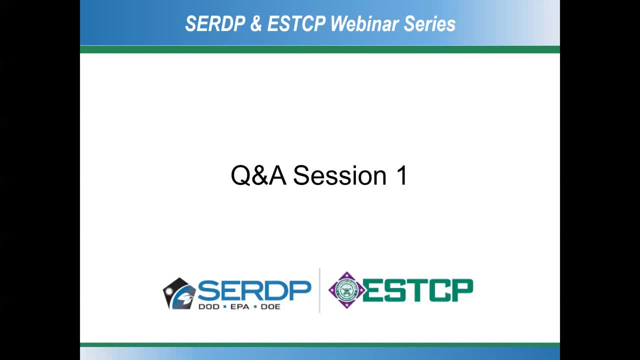 Most PhD students can manage the calculations. They're not difficult in the sense that once you understand what has to be done, you have to make 53 solvent water partition coefficient calculations. After that it's relatively straightforward And the method: All of the data that we use to generate. 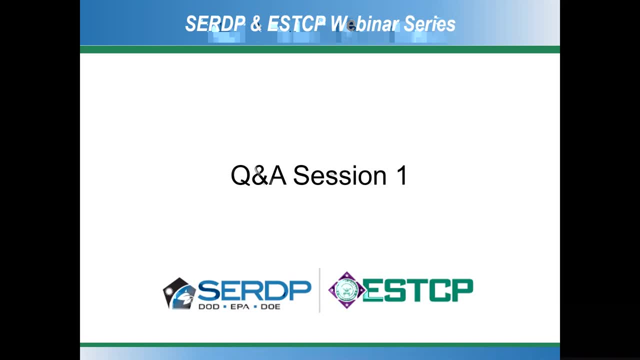 The results in the figures I showed you are all part of the SIRTA final report And there are examples that we've shown in detail so that you can- you can check your own methods. The best thing is to have someone that's a friend of yours that can check your quantum chemistry, or to have someone that's actually a professional quantum chemist. 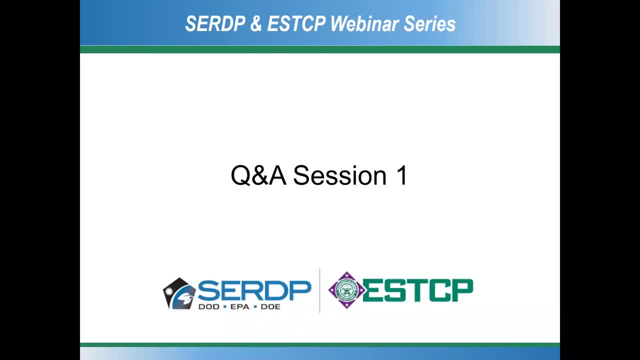 There are a number of such people within DoD That are, you know, state of the art quantum chemists. So it is not something where you need a PhD quantum chemist to do the calculations, but you do. If you're getting some odd results, you certainly need someone to talk to. 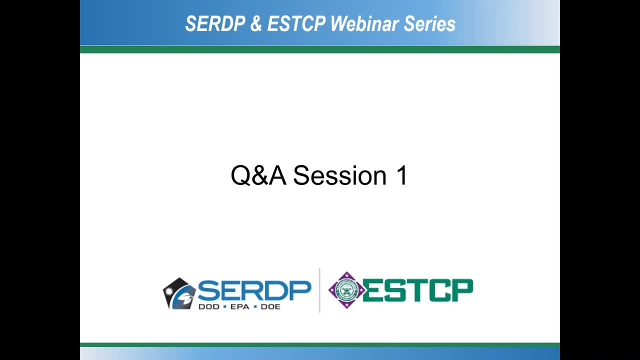 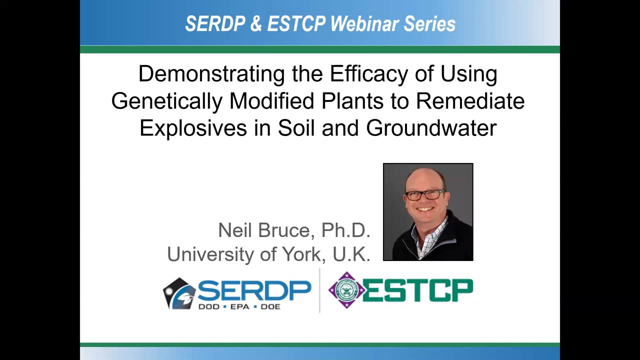 Okay, Well, Dom, we thank you very much for this presentation and for answering questions, and we will bring Dom back at the end of the webinar for a few more questions. Thank you. At this time I'd like to introduce our second speaker, Dr Neil Bruce, the director and professor of biotechnology in the Center for Novel Agricultural Products at the University of York in the United Kingdom. 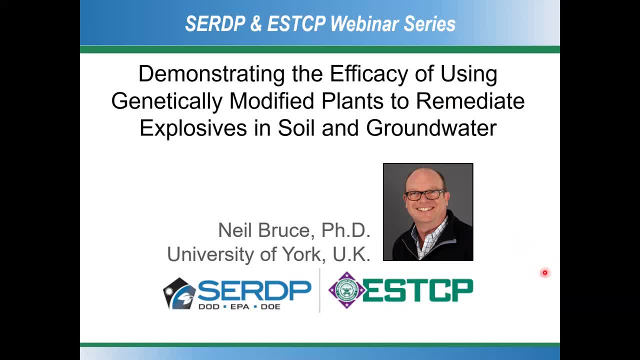 Dr Bruce's research focuses on plant and microbial metabolism of xenobiotic compounds and the characterization of the enzymes mediating these metabolic processes. He has discovered a diverse range of enzymes that have environmental and biotechnological applications. Dr Bruce has been studying the chemistry, biochemistry and molecular genetics of explosives metabolism in plants and microbes for over 20 years. 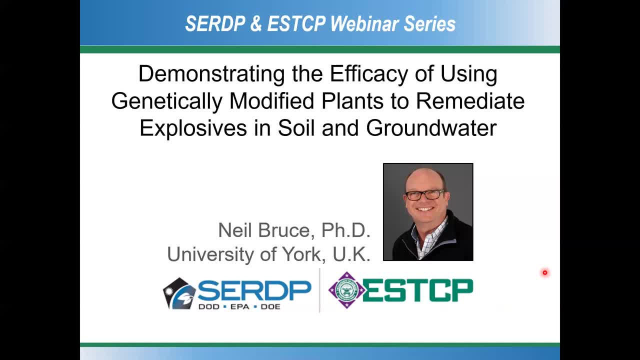 He has co-authored over 150 peer-reviewed papers, many of which focus on explosives biodegradation. He earned his doctoral degree from the University of Kent. Neil, please proceed. Thank you very much, Jennifer, and thank you for the introduction. 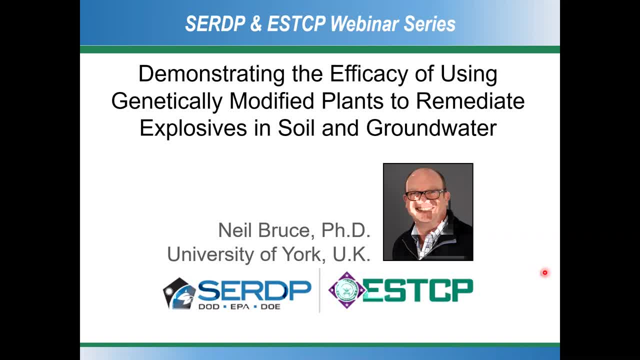 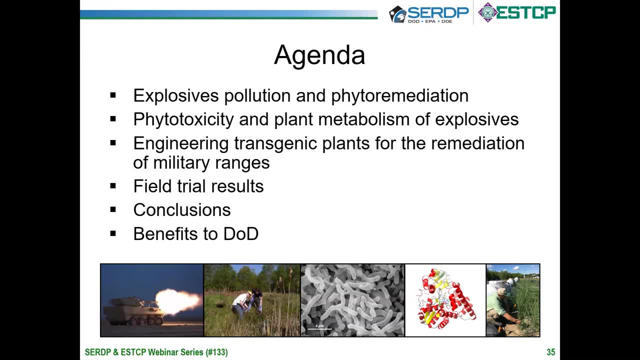 Hello everyone, I'll just start off by giving you a brief outline of my presentation, So I'll just very briefly touch upon explosives pollution and the use of plants to remediate soil contamination, And I want to tell you a bit about the work we've done in terms of elucidating the mechanism by which TNT is highly toxic to plants, and then go on and tell you about some of the work we've done. 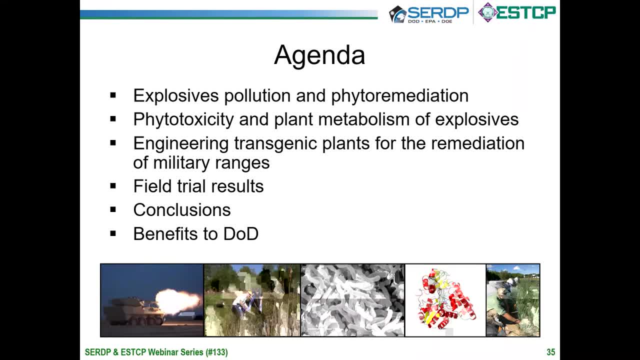 understanding plant metabolism of explosives. Specifically, today I'll be talking about TNT And then I'll touch briefly on some prior work we did quite a while ago now on the microbial degradation of RDX, where we identified a rather novel enzyme, which we call XPLA, that degrades RDX. 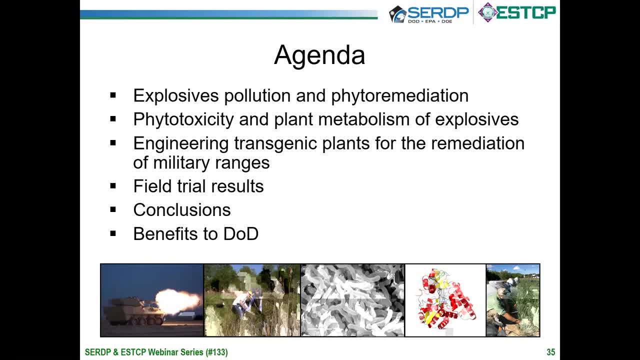 And then how we've been using the fundamental information that we've gained on the plant and microbial metabolism of explosives to engineer, rebuke and control explosives. So robust transgenic plants for the remediation of explosives contamination on military ranges. And then, importantly, I want to present some of the results that we've got from our field trial with our transgenic grasses. 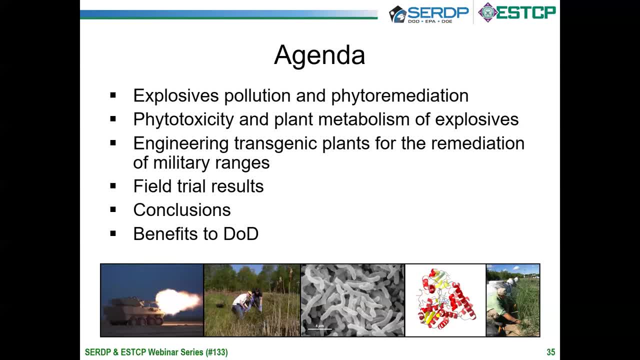 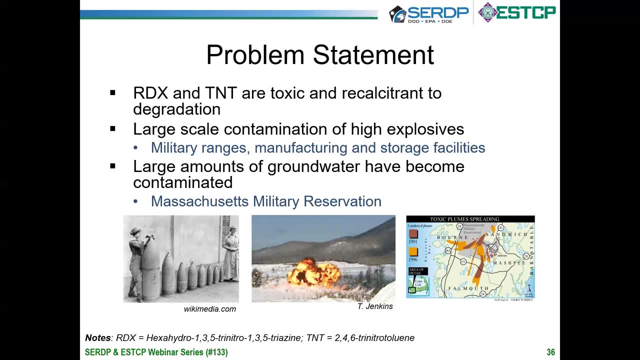 in terms of remediating or removing RDX contamination from contaminated soil. Okay, so problem? I think probably everyone in the audience is aware that RDX and TNT are toxic and they're highly recalcitrant to degradation, So this means that they can persist for very long periods of time in the environment. 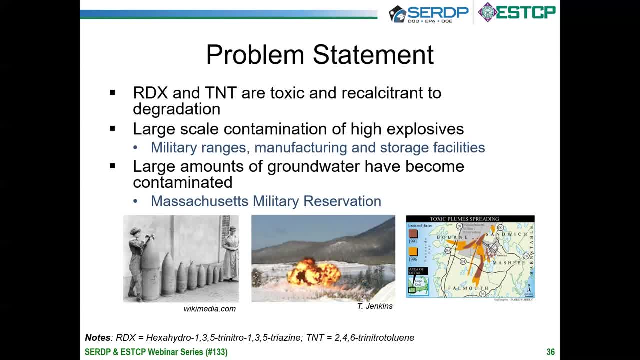 And indeed there are sites sort of dating back to the Second World War that are still contaminated with TNT. But what I want to focus on today is the contamination of military ranges, which is an intractable challenge Because the military needs to train with live munitions. 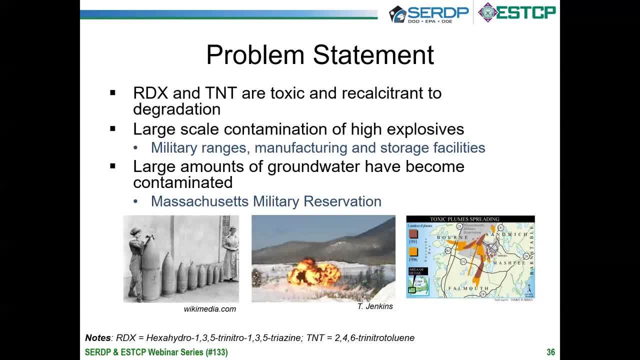 And so you've got continual contamination of these sites And you have the problem of these contaminants migrating through the soil and then going on to contaminate the groundwater, And the scale of contamination really is considerable. So there's a real need to develop a technology that could be used on ranges. 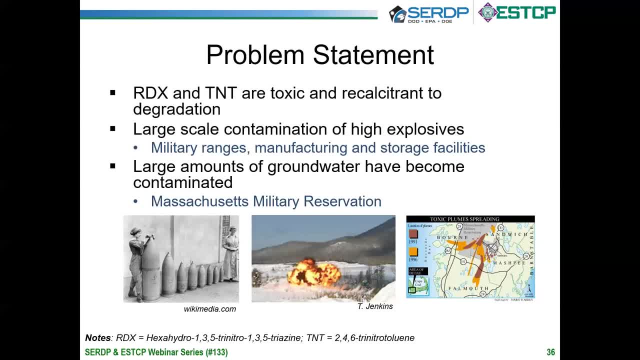 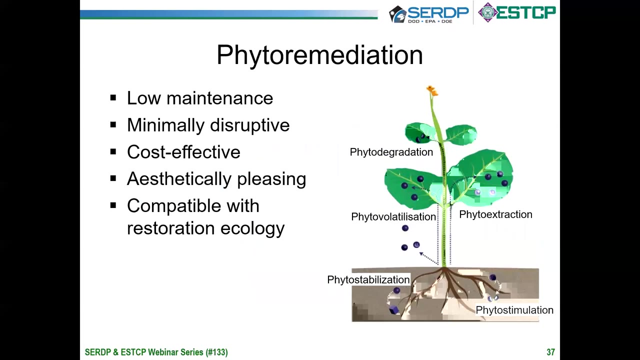 to ideally remediate them but, importantly, to capture and contain those explosive contaminants before they migrate through the soil and contaminate the groundwater, as has been seen at the Massachusetts Military Reservation. So plants in some ways are ideal for this. They're low maintenance, they're minimally disruptive. 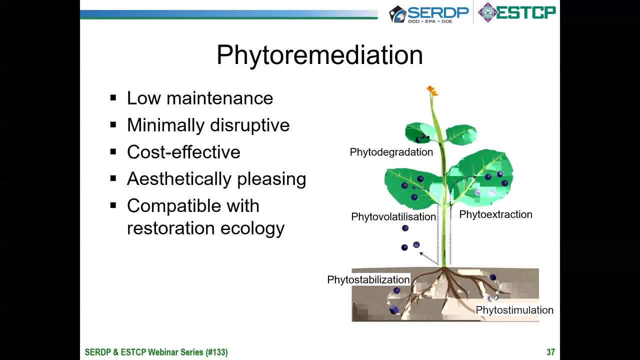 they're cost effective and they're aesthetically pleasing And they'll take up unnatural compounds And they might be able to sequester them within the plant biomass. They may have enzymes that are capable of degrading them And in some cases they can volatilize the compounds into the atmosphere. 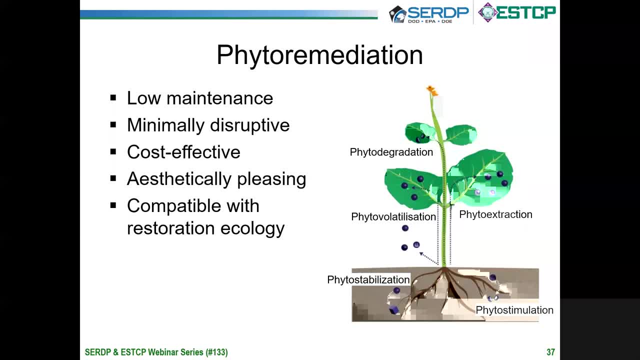 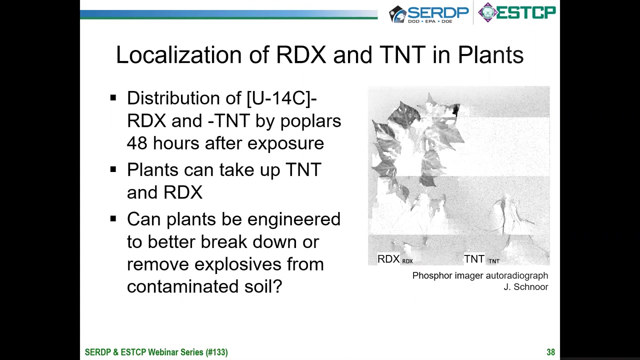 But in terms of using plants to remediate explosives pollution or to contain explosives contamination on site, there's two major inherent problems in terms of using plants, And the first of these is that plants have very limited or actually probably no metabolic activity towards RDX. 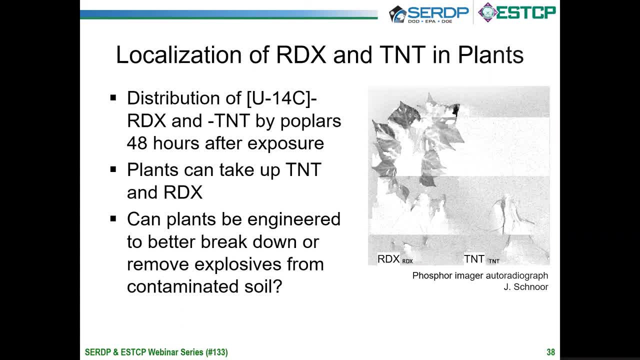 And this can be seen here in this slide, which shows an image of an experiment that Jerry Schnorr's group did, where they visualized the transports of radio labeled RDX and TNT in poplar plantlets, And you can see quite clearly here with RDX. 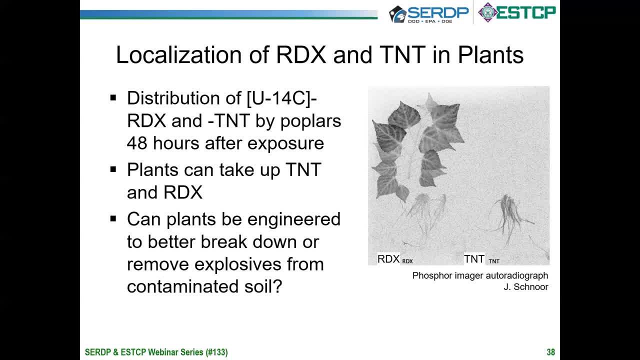 that it goes up through the roots and translocates into the aerial parts of the plant. You can see it throughout the whole plant And RDX will accumulate to a certain level and then the plant won't take up any more RDX. 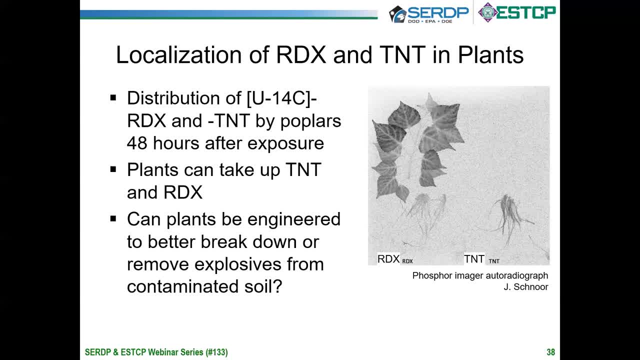 And when the plant dies, the RDX will eventually be returned back to the soil. But if you look at TNT, you can see there's something quite unusual happening here, in that TNT is remaining in the roots. It's sequestered there. 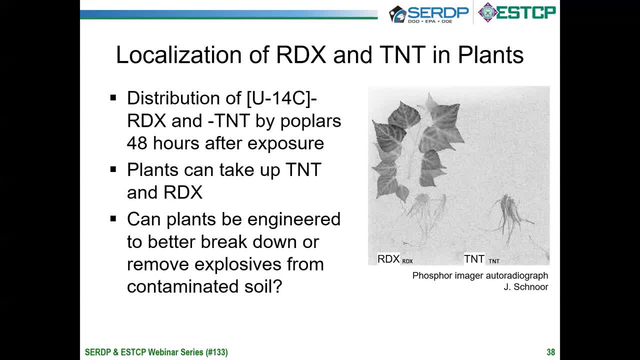 It doesn't get up into the aerial parts of the plant, And that's something that puzzled us. We wondered what the plant was doing to the TNT to prevent translocation into the aerial parts of the plant, And I'll come on to that in a minute. 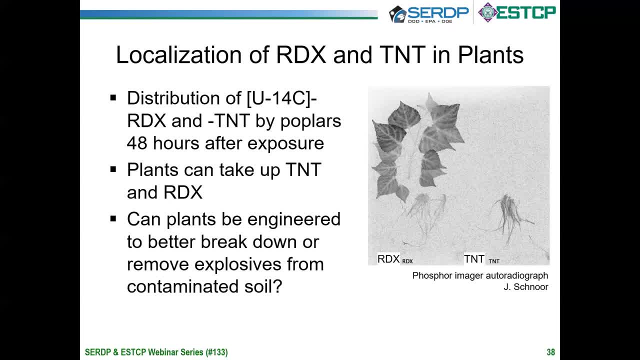 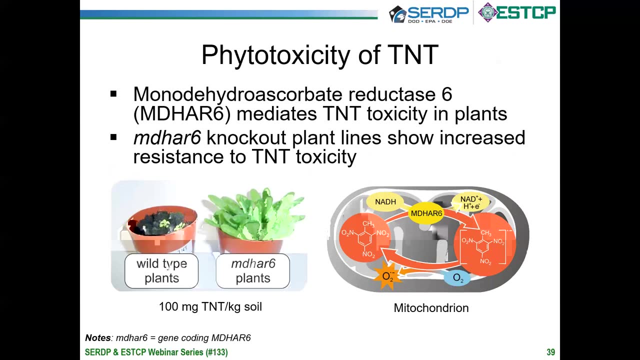 And so this posed the question: could we engineer the plants to improve their ability to take up explosives but, importantly, to break them down? So the other inherent problem is that TNT is highly toxic to plants, And we wanted to illustrate the mechanism by which TNT exerts its toxicity. 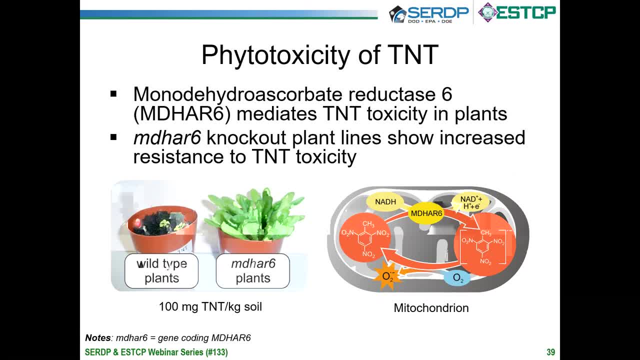 And what you can see here is that we've got these plants growing in soil. The plant is Arabidopsis And the soil contains 100 milligrams of TNT per kilogram of soil, And what you can see is that the plants are incredibly stunted. 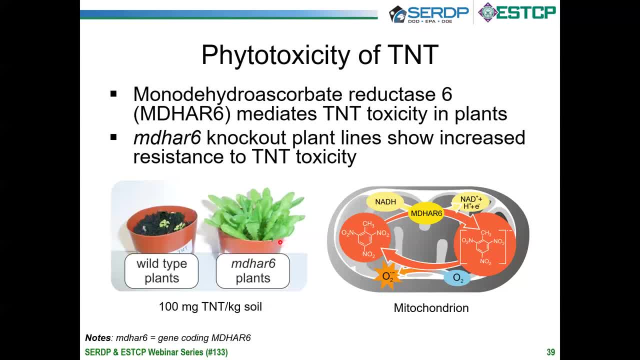 And if there was no TNT in the soil, this is what the Arabidopsis plants would look like. But in fact, here there is in fact TNT, the same concentration of TNT, 100 milligrams of TNT per kilogram of soil. 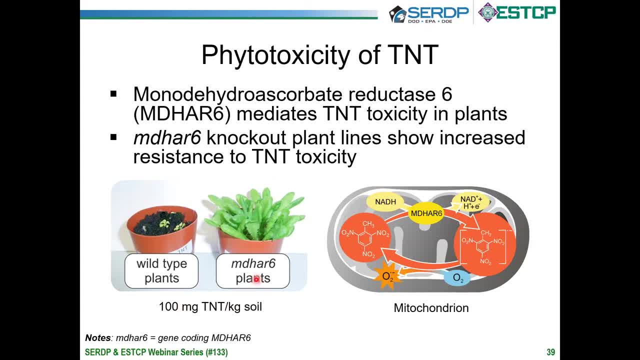 And what we have here is a mutant line that we identified And that mutation allows the plant to tolerate high levels of TNT. And we mapped that mutation And we identified that the mutation was in a gene called MDHR6 that encodes for an enzyme called monodehydroascorbate reductase. 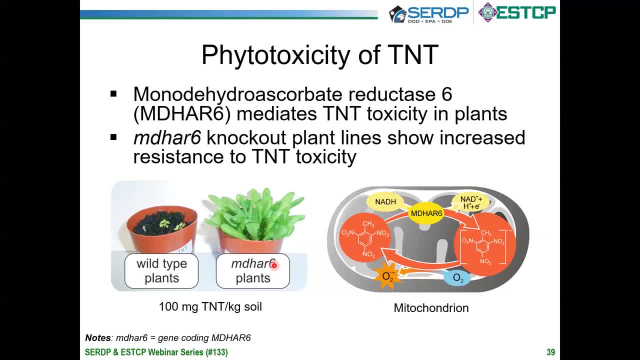 And this enzyme is plant specific And it's found in the mitochondria of plants, the power, the organelle that generates the power for eukaryotic cells. And what happens is that this TNT diffuses into the mitochondria. 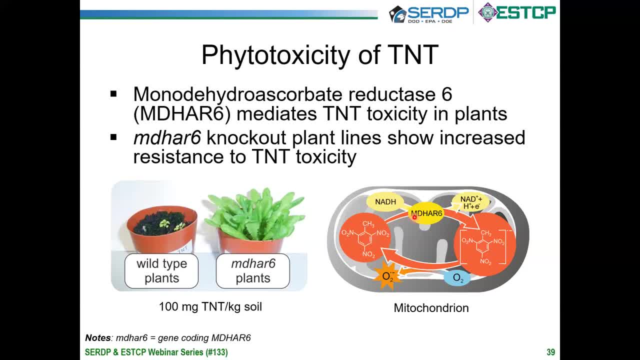 and it's a substrate for this enzyme. And this enzyme uses a cofactor NADH and reduces TNT to a nitro radical, And that radical will react with molecular oxygen to produce reactive oxygen species that are cell damaging, And in doing so the TNT is reoxidized back to. 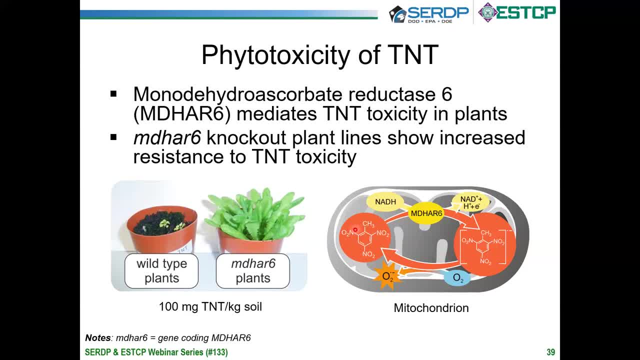 sorry, the nitro radical is converted back to TNT, So you end up with this futile cycle. So one molecule of TNT can keep on going around this cycle, generating reactive oxygen species, And it's these reactive oxygen species that ultimately kill cells and eventually the plants. 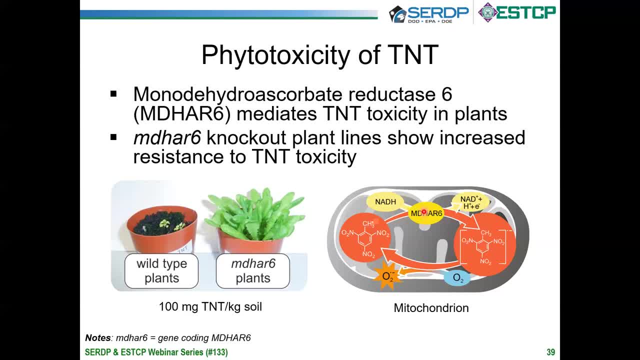 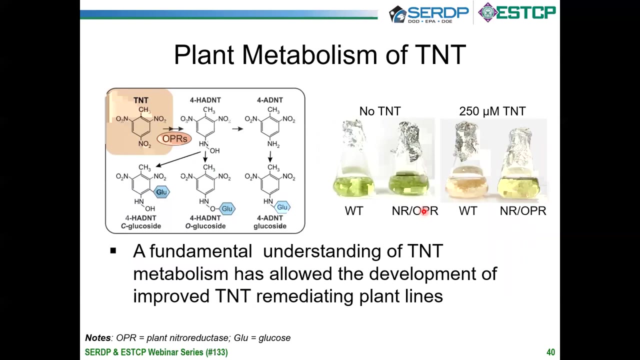 So knocking out this gene confers on the plants resistance to TNT toxicity and providing the possibility of using these plants to remediate higher concentrations of TNT in the environment. So, going back to that image of TNT being sequestered in the roots, we identified the mechanism by which this was happening. 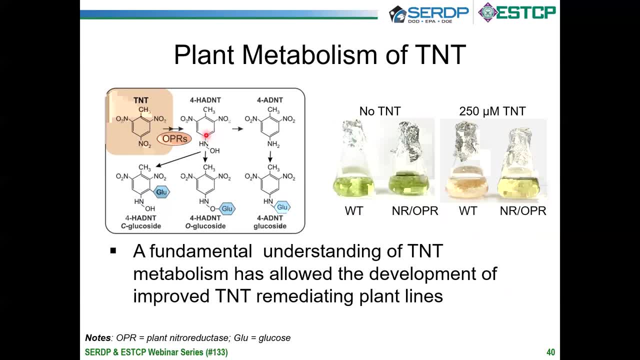 So there's an enzyme in plants, a nitro reductase, that reduces the nitro group of TNT to a hydroxyl amino derivative and then through to an amino derivative, And what that enzyme is doing is adding functionality to the TNT molecule. 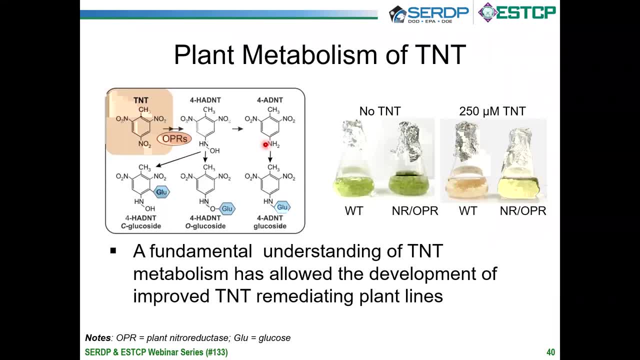 that the plant can then recognize. And so what the plant then does? it adds a glucose molecule to the TNT metabolites, And these glucoconjugates can then be locked up in the plant cell wall. So it's removed, removing these TNT molecules. 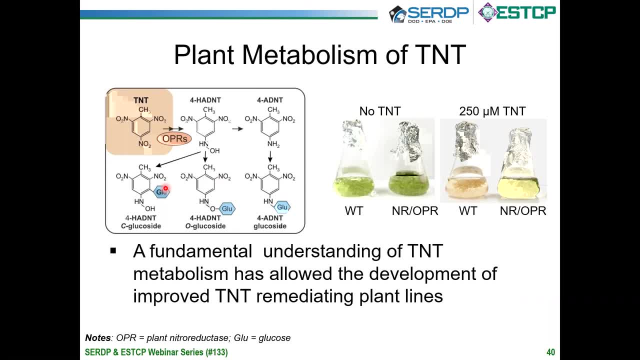 so that they no longer diffuse into the mitochondria. So this fundamental understanding of TNT metabolism allowed us to develop improved TNT remediating lines. And what we did was we overexpressed a nitro reductase in plants, And in this case not the plant's own innate nitro reductase. 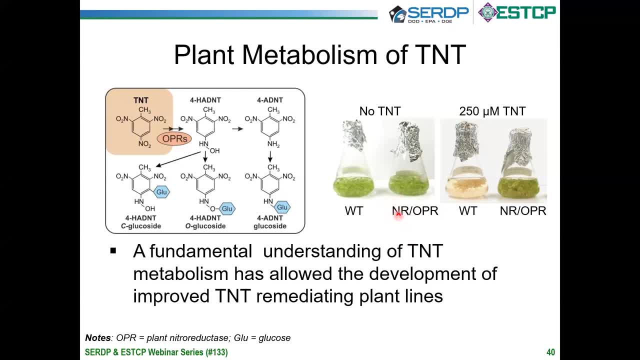 but a bacterial nitro reductase that has much greater activity towards TNT. So the plant cells now are rapidly converting TNT to the hydroxyl amino dinitrotolerant product, which is then getting conjugated to sugar and then locked up in the plant cell wall. 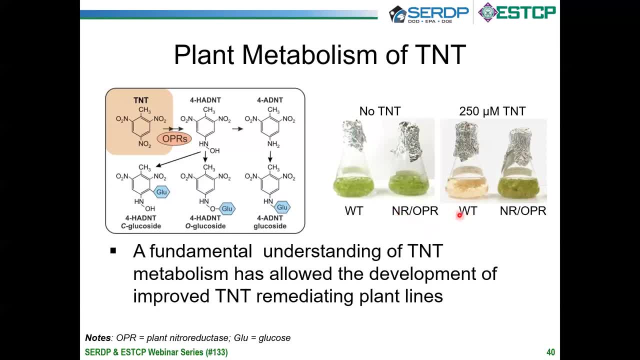 And this works remarkably well. So here you can see. so here you've got the wild type plant that's not transformed or modified in any way. Here you've got the transgenic line in liquid media containing no TNT. You can see the cell. 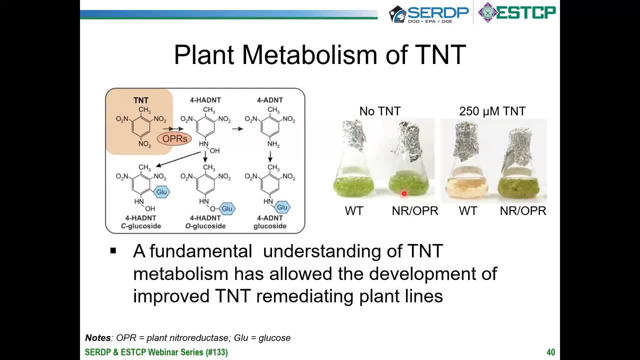 the plant cell. the plants are green. They're healthy. In the presence of 250 micromolar TNT. you can see the wild type plants are now dead. They're chlorotic. They haven't removed any of the TNT from the medium. 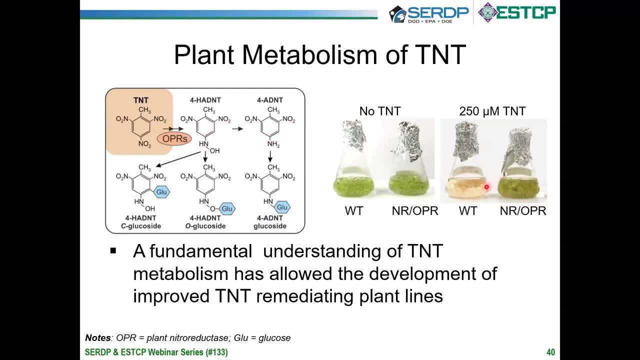 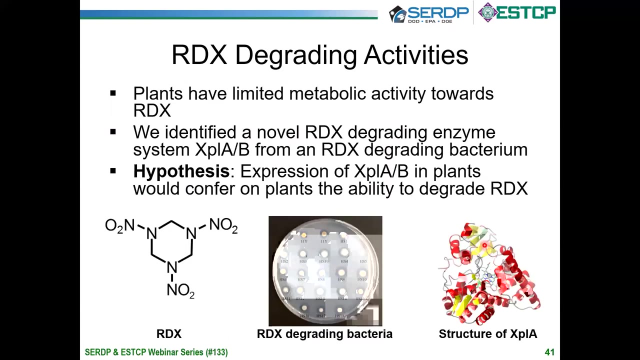 Whereas the transgenic lines are green, healthy, They've increased in biomass and they've removed all the TNT from the medium. In fact, these plants work so well that they'll remove basically saturating concentrations of TNT from the medium, So that was really an exciting result. 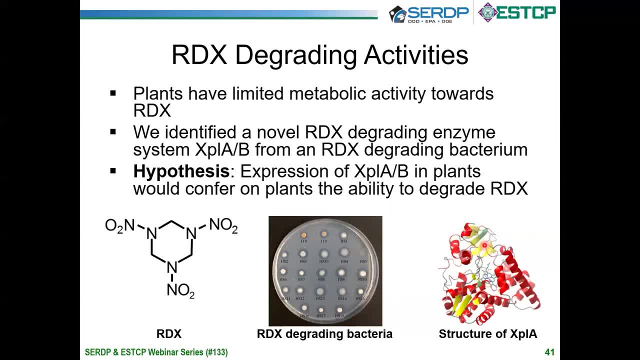 But we needed to go on and engineer our plants to take up and degrade RDX. So we couldn't find, or we don't know of any plant enzymes that do this. So our hypothesis was to express in plants a bacterial enzyme that could degrade RDX. 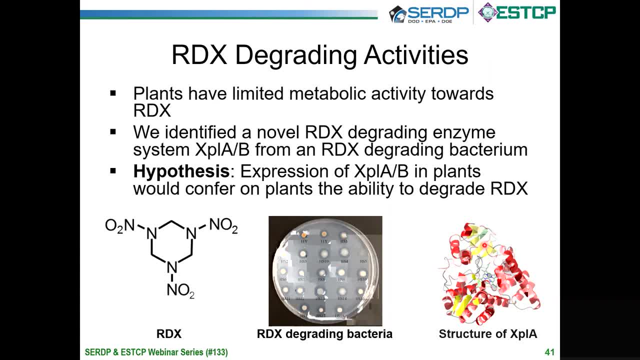 And we've gone out and done sort of classic selective enrichments in the past where we've isolated bacteria from RDX contaminated soil that could utilize RDX as a nitrogen source for growth. So you can see these bacteria going on the Zagar plate here. 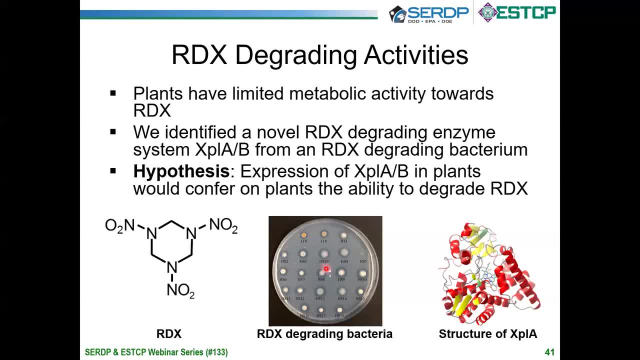 using RDX as a nitrogen source for growth, And in any of these bacteria we identified the enzyme that was mediating this degradation of RDX, And we call this enzyme XPLA. And XPLA is rather a novel enzyme. In fact, that's a cytochrome P450.. 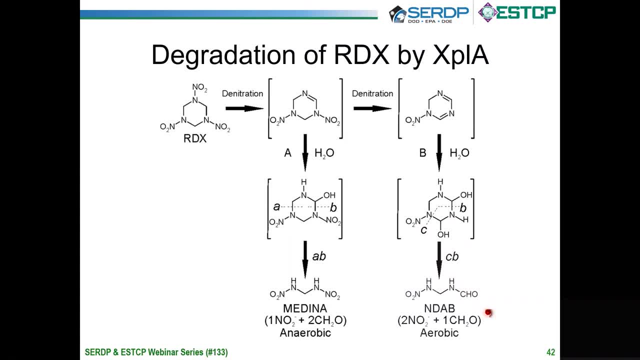 And it's novel because, unlike most cytochrome P450s, it doesn't use molecular oxygen in its reaction mechanism. So this enzyme, what it does? it reductively clips off nitro groups of the RDX molecule. So here you can see: the enzymes remove two nitro groups of RDX. 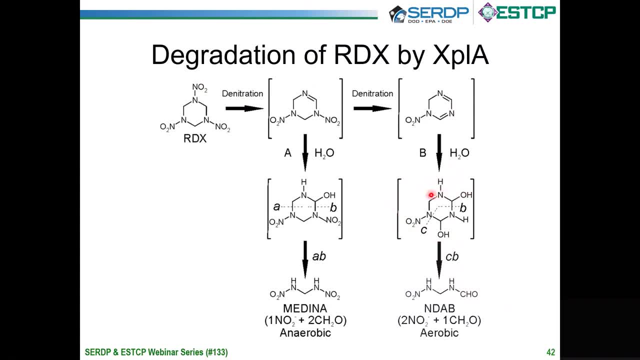 It then goes on to that forms this unstable intermediate that basically falls apart to generate these non-toxic metabolites, MdA as a butanol, MdAB- two equivalents of nitrite and an equivalent of formaldehyde, And it's the nitrite that the bacteria are using. 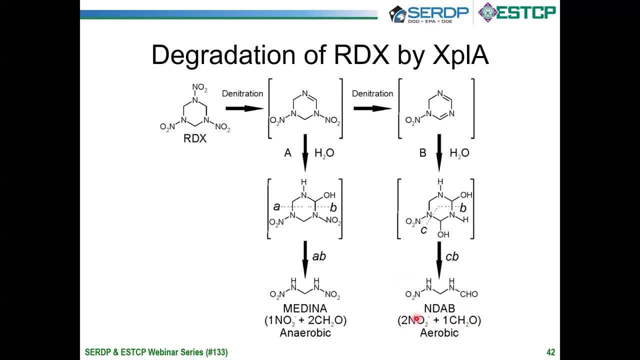 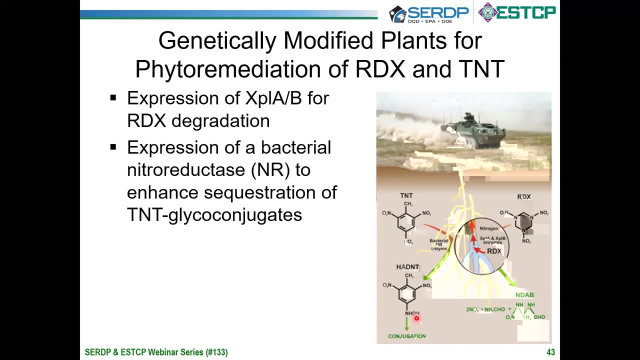 as their sole nitrogen source for growth. So our strategy in terms of engineering plants for the phytoremediation of RDX is quite straightforward. The idea being is that we'd express XPLA and its partner reductase XPLB in plants. 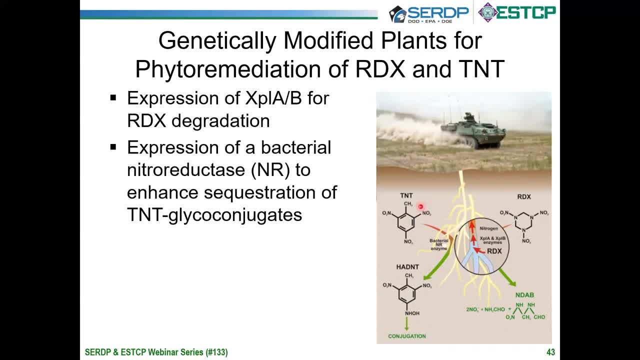 along with this bacterial nitro reductase that reduces TNT to the hydroxylaminodynitrotoluene derivative, which then gets conjugated to sugars and the TNT gets locked up in the biomass. So with RDX it would get broken down to metabolites. 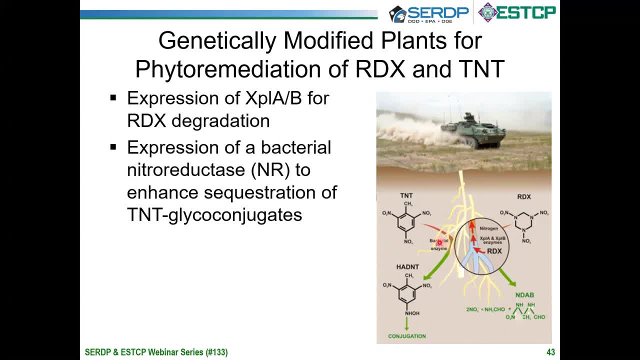 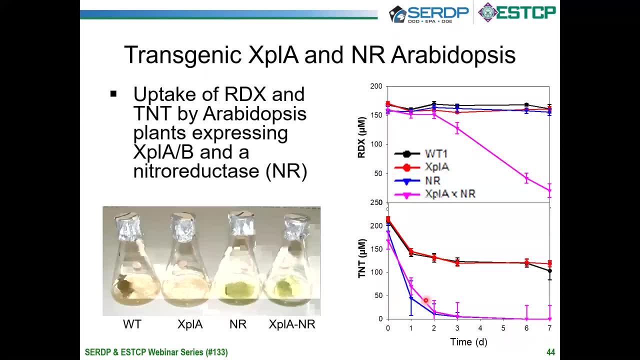 that the plant can actually utilize, Whereas with TNT, these conjugates would be locked away in the plant cell wall. So what you can see here are Arabidopsis plants in liquid medium, And the liquid medium contains TNT and RDX, And in the first flask we have a natural wild type plants. 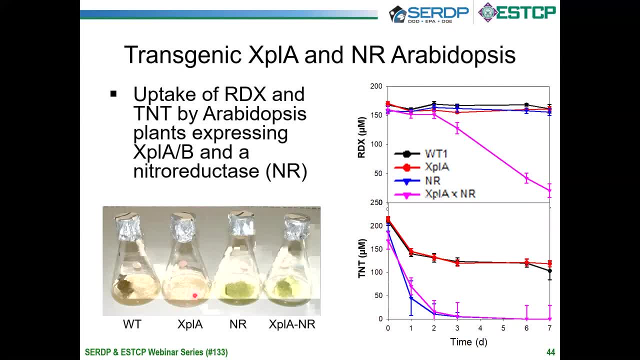 In the second flask we've got transgenic lines expressing XPLA and its partner reductase, XPLB. In the third flask we've got plants expressing the bacterial nitro reductase. And in the final flask we've got the plants expressing all those genes. 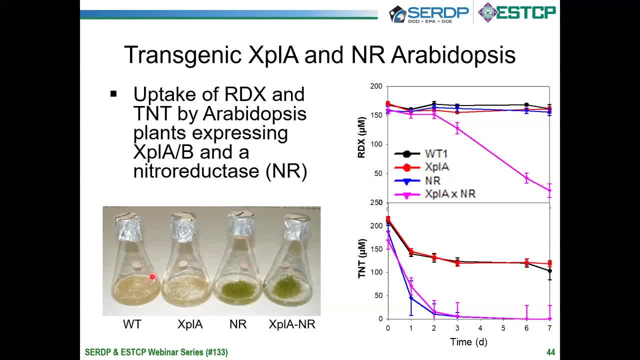 XPLA, XPLB and the nitro reductase. So you can clearly see that the wild type plants are dead And if you look at the graph, you can see that they've hardly removed any of the TNT and none of the RDX. 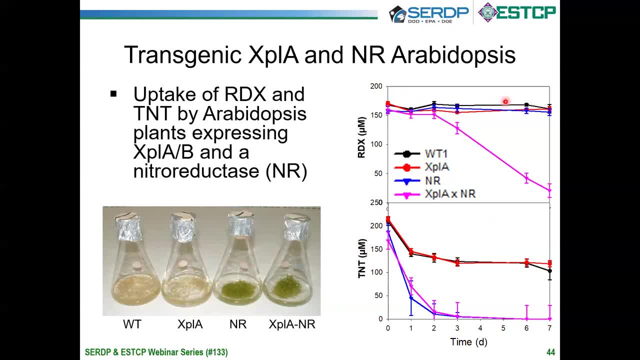 And the same is true for the XPLA lines. The plants have been killed due to the TNT toxicity, Whereas with the nitro reductase lines you can see that within in blue here- in a matter of two days it's removed all of the TNT from the medium. 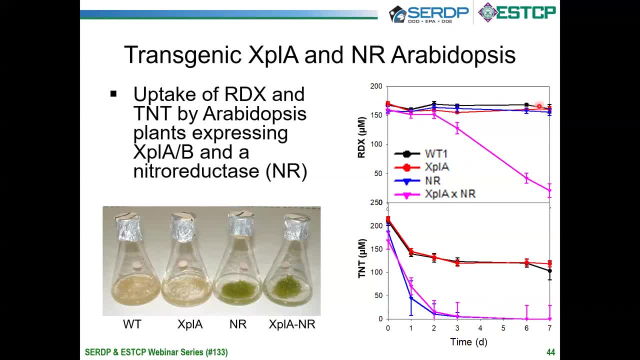 but it's unable to remove any of the RDX, Whereas with the multiple transgenic line you can see that, like the single nitro reductase line, they're dead, But the plant lines are able to remove the TNT within a couple of days. 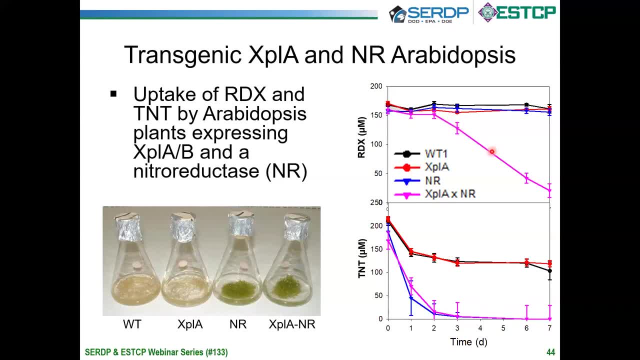 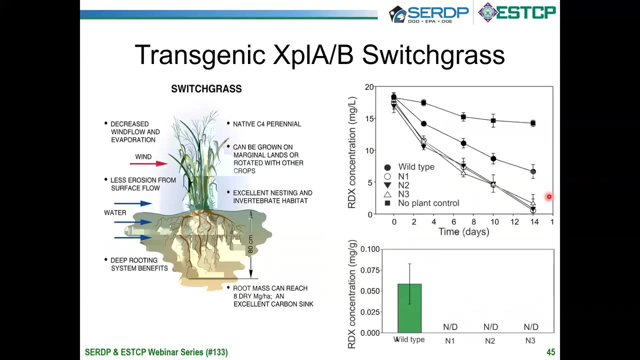 And then the plants are able to then degrade all the RDX from the liquid medium. So this was an important finding and an exciting result, And this then spurred us to go on and engineer plants that would be more appropriate for use in the field. 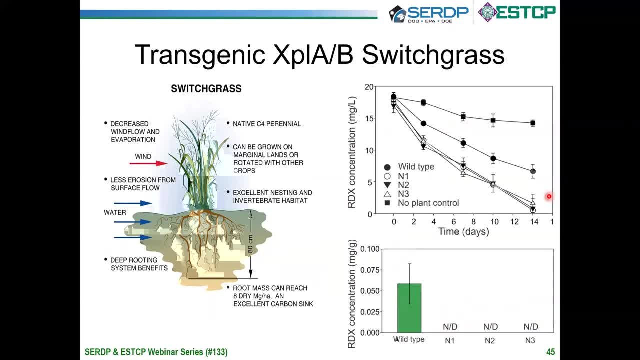 because Arabidopsis is a model plant. It's too small. it's completely inappropriate for phytoremediation applications. So, in collaboration with our colleagues at the University of Washington, we went on to engineer transgenic switchgrass. And the reason why we chose switchgrass- 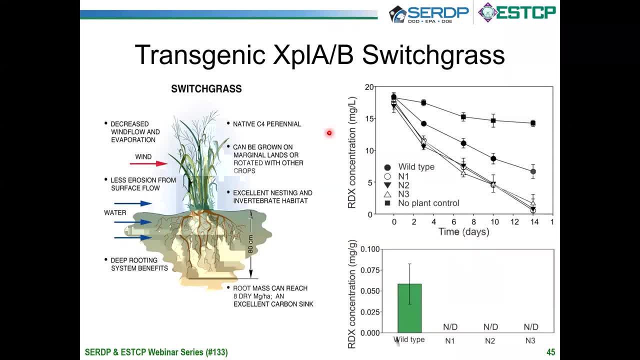 is that switchgrass is native to many US military ranges. It produces a large amount of biomass. The roots will penetrate quite significant depths- up to about a meter in the soil- and have very dense root systems. So those root systems cover a large surface area. 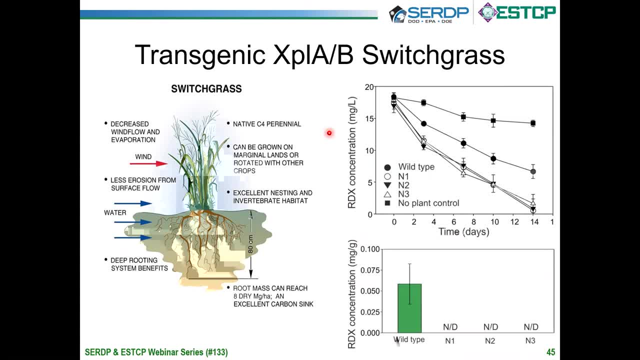 And so the other important factor for choosing switchgrass is that, due to the bioenergy programs, there are now good genetic tools for genetically modifying switchgrass. So much as we did with Arabidopsis: we expressed our two ends or three enzymes in there. 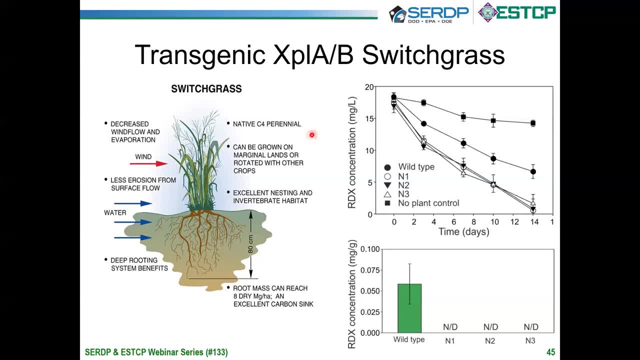 XPLA and XPRB and the nitroreductase, But for now I'm just going to focus on the results that we've got for RDX. So we tested our transgenic lines out, as we did before, in liquid medium. 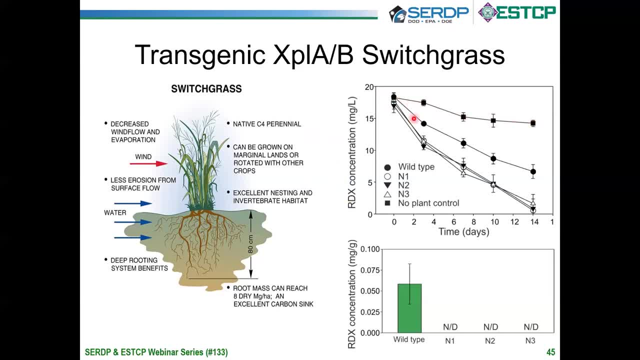 And you see in the no plant control there's very little RDX being removed from that medium over time. The wild type plants are removing RDX from the mediumness because the switchgrass has got quite a large amount of biomass and it's taking up RDX. 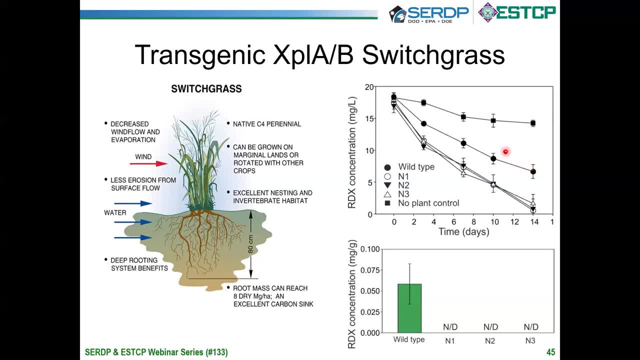 into that biomass And that's why you're seeing the removal here of RDX from the liquid medium. But you can clearly see that the transgenic lines are much more rapidly removing the RDX but, importantly, they're degrading it, And that's what you can see in the second graph. 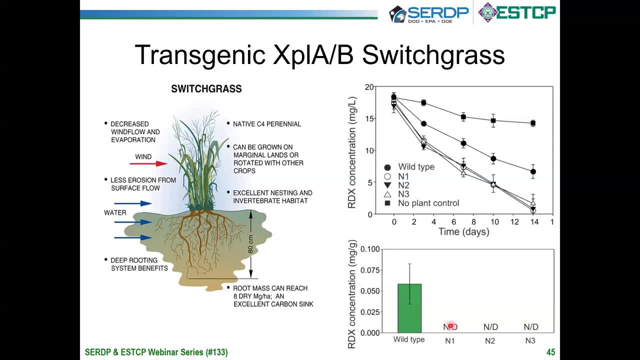 But the independent transgenic lines. when you assay the plant tissue, you cannot detect any RDX, whereas you've got significantly significant quantities of RDX being measured for the wild type lines, And that mirrors that auto-radio graph that I showed early on. 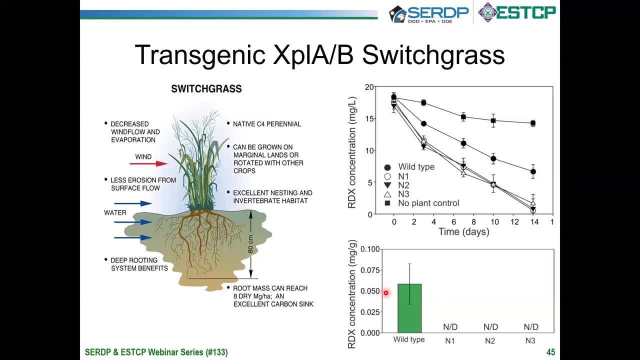 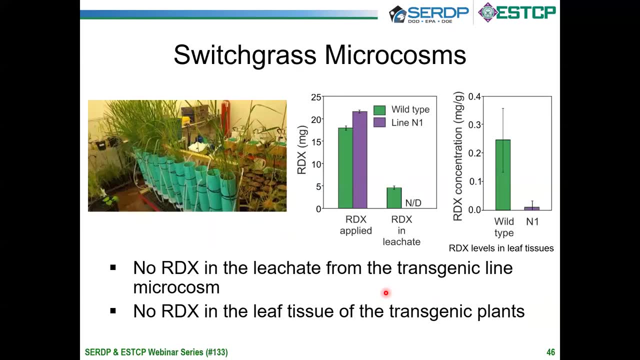 where you've seen RDX being translocated throughout the whole plant and remaining there. So we then needed to go on and do soil studies. So these are soil microcosm studies. So these are experiments where we're wanting to mimic effectively what will happen on a military range. 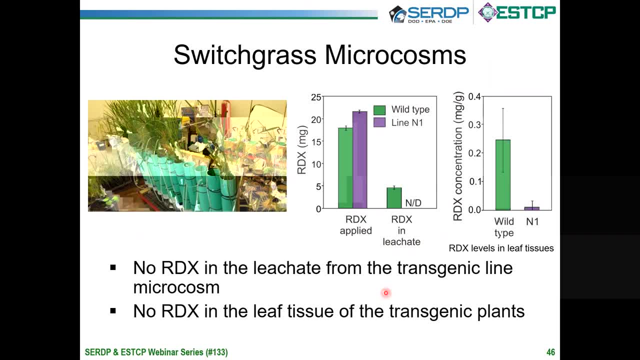 Where you've got particulates of RDX that will be dissolved and migrate into the soil. So we watered in RDX into the microcosm, left it there for a period of time and then we flushed through the remaining RDX and measured it in the leachate. 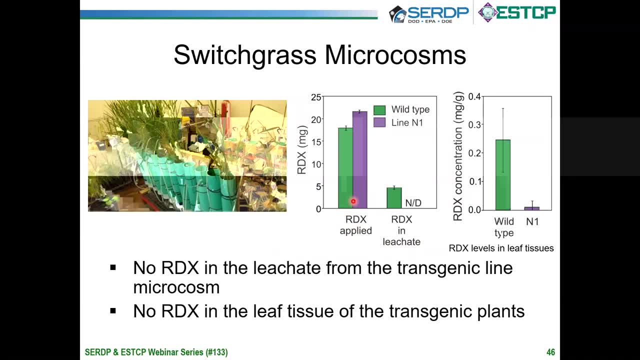 So what you can see here is that we could measure RDX in the leachate from the wild type plants. so this is getting washed through the microcosm, Whereas with the transgenic lines we were seeing absolutely no detectable RDX. 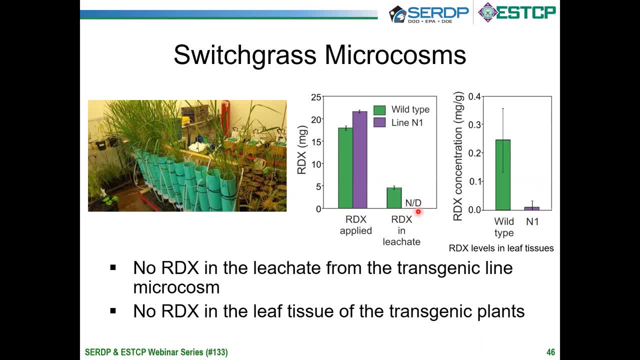 coming through in the leachates. The plants had taken up and removed and degraded the RDX, preventing it migrating any further through the soil And again, mirroring what we see in the liquid cultures, we see no or very little RDX being detected. 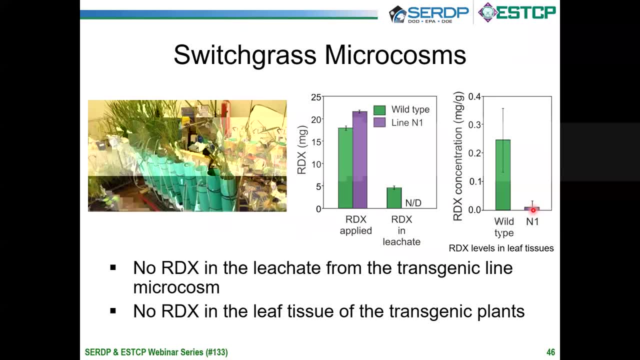 in the leaf tissues. So this was a fantastic result, And we've done these trials in the lab and in glasshouse studies. But really to demonstrate the efficacy of these plants, we needed to test them in the field, And so we're very fortunate to be able to do field trials. 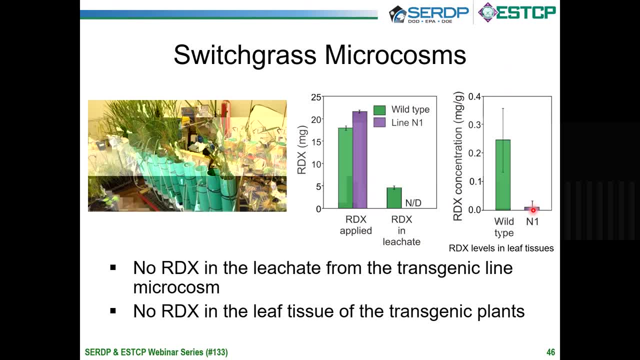 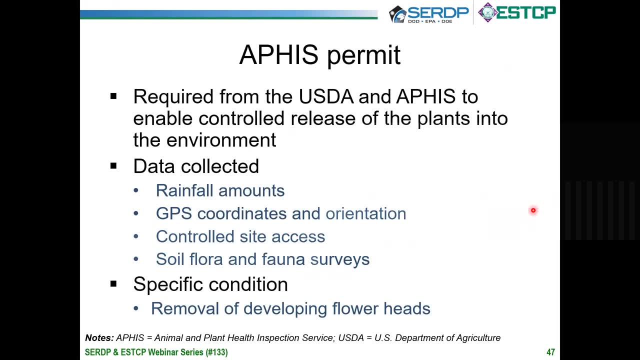 at Fort Drum in New York State And the next Oh. so before we could do the trials, we needed to get a permit from USDA and APHIS to enable the controlled release of these transgenic plants into the environment. And as part of that permitting process, 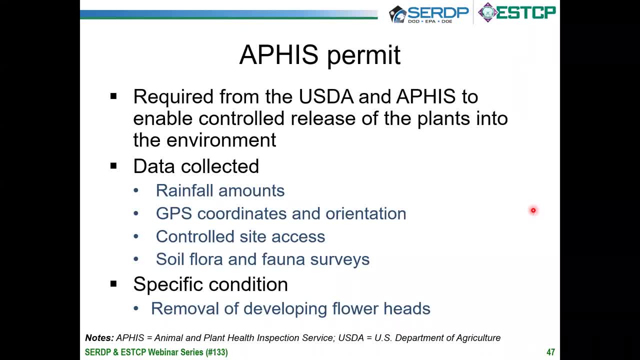 we needed to collect some data. We needed to log the rainfall amounts on the plots, We needed to provide GPS coordinates of the sites, We needed to make sure that there was only controlled access to the sites And we needed to survey the soil flora. 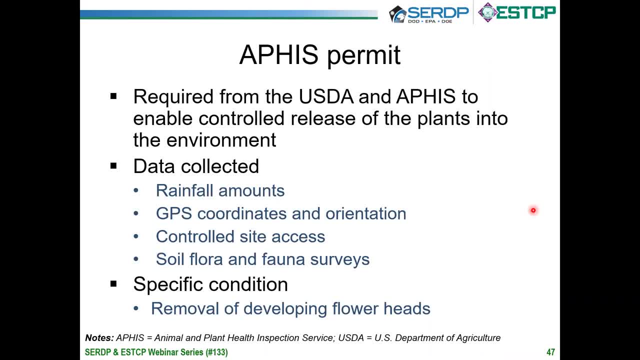 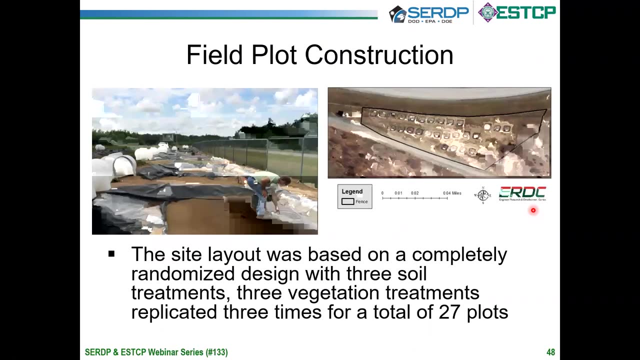 and fauna at Fort Drum around the test sites And, as a specific condition, we needed to remove the developing flower heads from the plants to prevent cross-pollination with other grasses at Fort Drum. So here you can see some images in terms of the construction of our field plots. 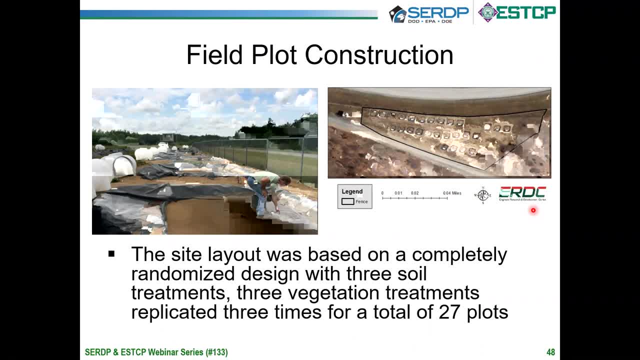 The site layout was based on a completely randomized design. We had three soil treatments and three vegetation treatments, And these were replicated three times, resulting in a total of 27 plots, which you can see from this aerial photograph of the site at Fort Drum. 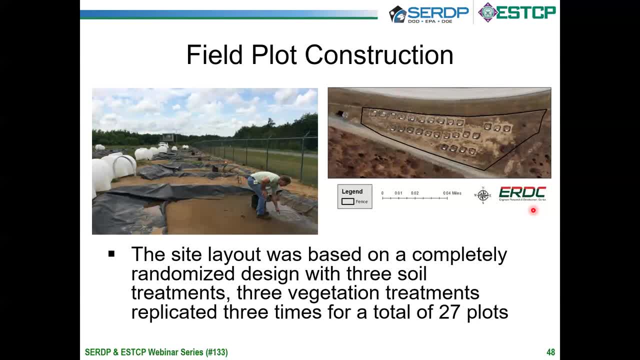 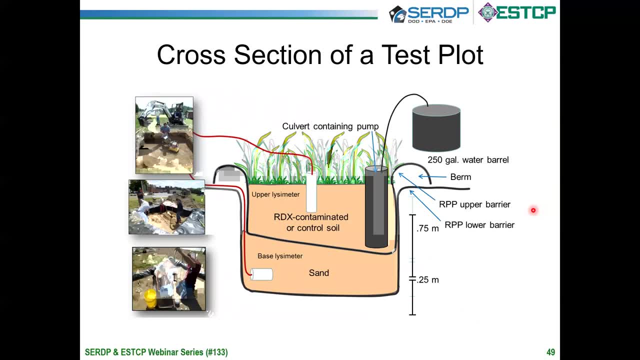 The plots were three meters by three meters And this next slide shows you a cross-section of the plot. So the plot was about a half a meter deep, The soil from Fort Drum to fill the plots, And we contaminated the plots with RDX. 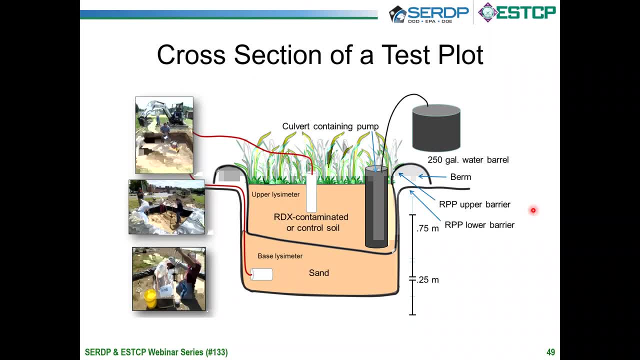 by mixing RDX with fine sand and putting that on the surface of the plots to a concentration of about 100 parts per million, which is around the concentration you'd find around a low-order detonation. Then in these plots we had lysimeters. 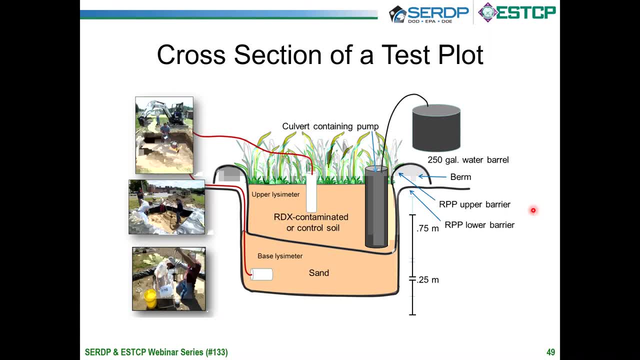 so that we could take soil water samples and measure the RDX concentration in the soil water Over periods of time. we had a culvert in there with a pump so that in cases of heavy rainfall we could pump out excess water into a holding tank. 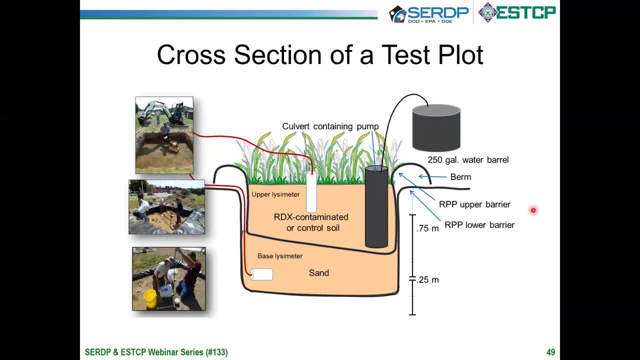 We also had an irrigation system So if the plots needed watering, we could water them from the water in the holding tank And we would sample these through the growing season. We'd take samples from the lysimeters and from the plants And we'd take samples from the plant leaf tissue. 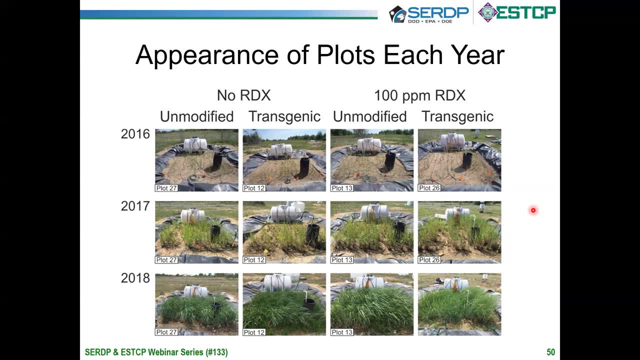 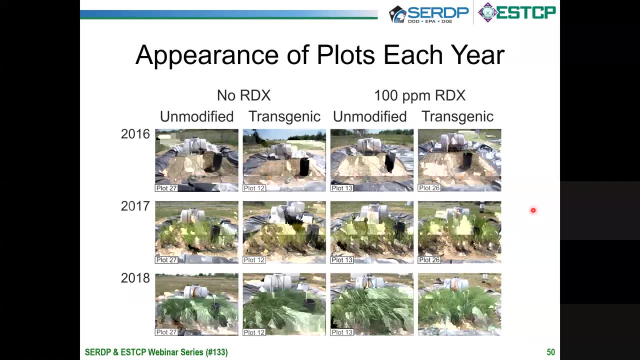 So this slide shows the appearance of the plots each year. So we got our permit in the summer of 2016.. So we were able to get our plants into the ground, which was a real champagne moment for us. And then we had 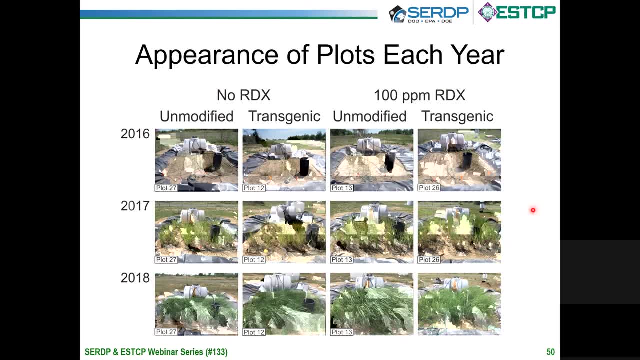 Well, so it was late summer, so we weren't able to get the plants into the ground. We weren't able to get the plants established enough to take any samples, But in 2016 and 2017, we had a terrible winter in New York State. 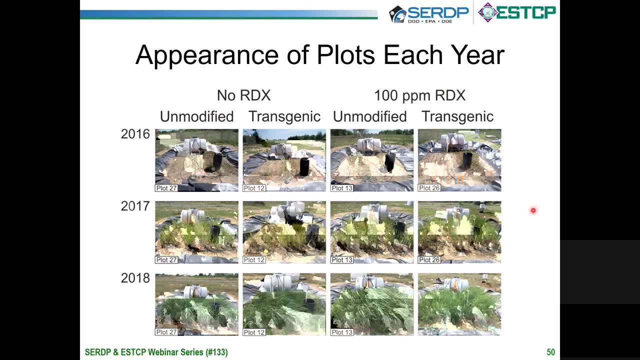 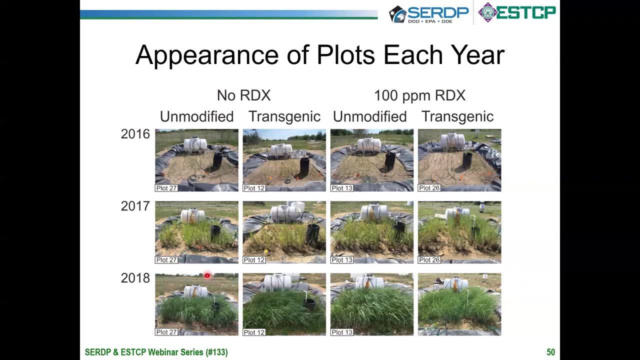 followed by one of the wettest summers ever in 2017, which meant the plants took a while to get established, And it wasn't really until 2018 that we were able to start taking samples from these plots, And you can see quite clearly in 2018,. 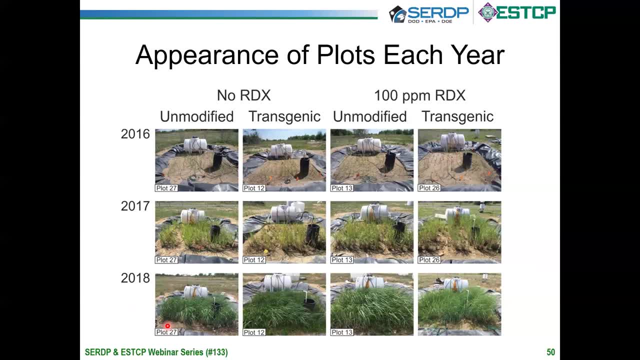 the plants had a really sort of dense coverage in the plots- Good canopy coverage, And what you can see here are representatives of unmodified plants growing in a plot with no RDX. This is the transgenic lines growing in a plot without RDX. 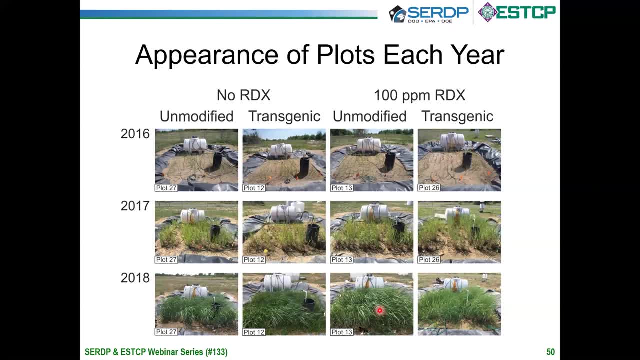 Here you can see the wild type plants growing on the plots in the presence of 100 parts per million of RDX. And here's the transgenic lines. So in terms of physiology of the plants, just looking at them, there is no significant differences. 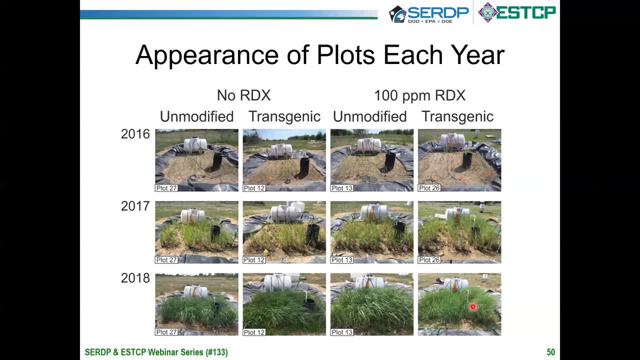 in terms of the amount of growth that we're getting on these plots. So in 2018, in the growing season, we took monthly samples where we'd take leaf material and analyze them for RDX content and take soil water samples from the lysimeters. 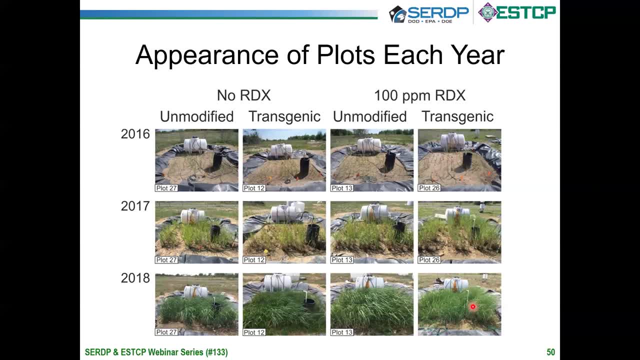 and determine the RDX concentration. We've got huge amounts of data which we've collected over this period and done a whole series of different types of analysis on it, which is not time to tell you about today, But these are presented in the report. 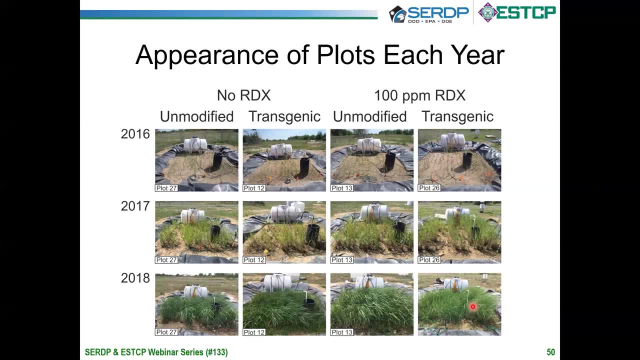 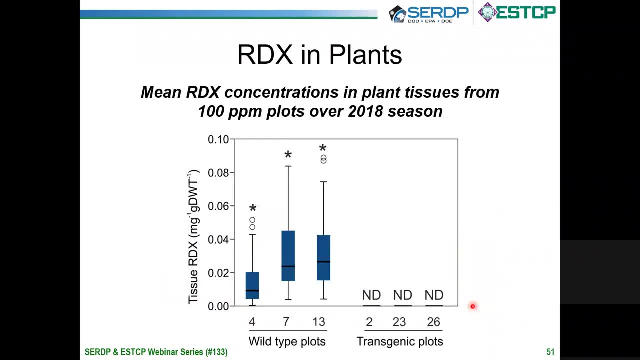 on the ESTCP S-ERDIT website, But I will just show you two slides that summarize our findings from our field trials. So this slide shows the mean RDX concentrations in plant tissues from the 100 part per million plots over the 2008 growing season. 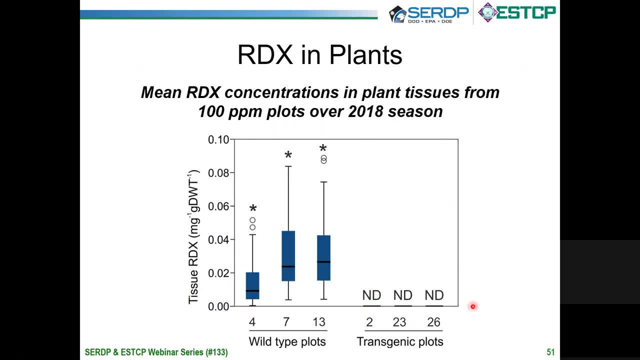 And we were delighted to find that they mirrored the results that we had in the glasshouse, the greenhouse studies and lab studies really very well, in that we were seeing significant amounts of RDX accumulating in the plant tissue in the wild type plants and absolutely no RDX could be detected. 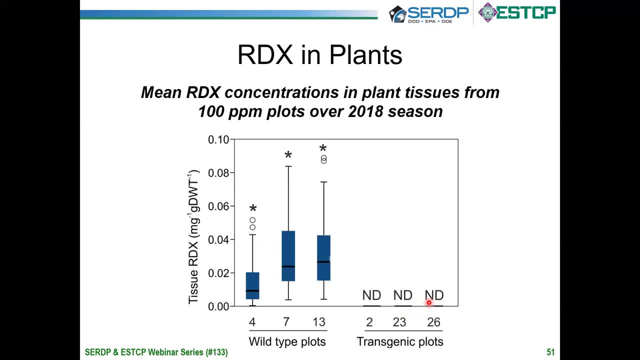 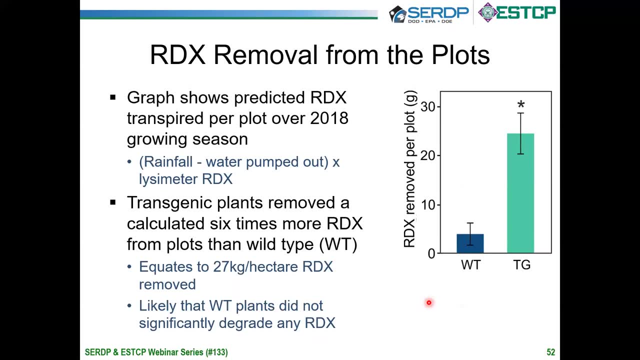 in the transgenic lines. So we then went on to calculate the amount of RDX that was removed from the plots, And we were able to do this by the fact that we knew the amount of rainfall that landed on the plots over the year. 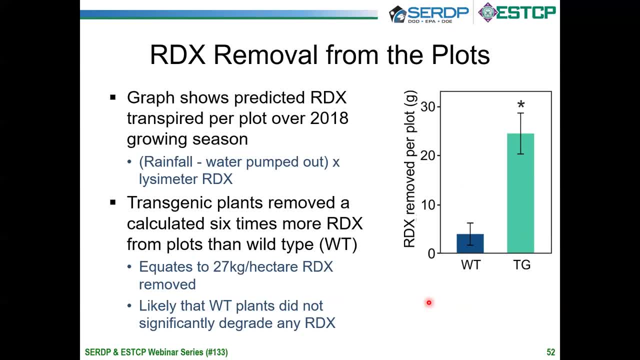 We know the amount of water that was pumped out and we know the concentration of RDX in the water from the lysimeter and from the analysis of the samples taken out from the lysimeter And the transgenic plants removed about six times more RDX from the plots. 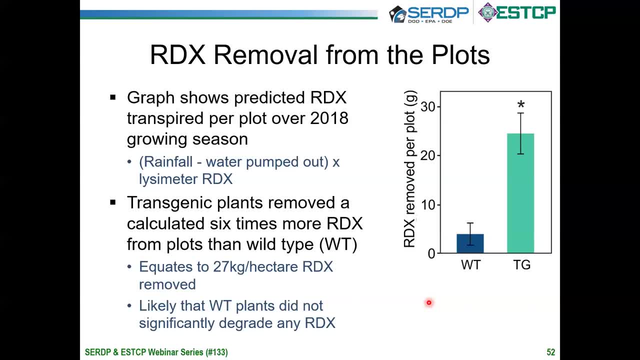 than the wild type plants, And this equates to something like 27 kilograms of RDX per hectare, which I think is quite remarkable, considering these are unoptimized systems And we were getting removal from the soil by the wild type plants. but you need to remember, of course, 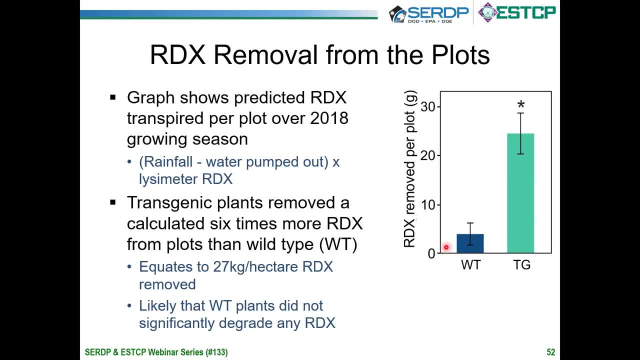 that our RDX in those wild type plants is not being degraded. So when the plant dies, that RDX is being returned back to the soil. So any plants on a contaminated site is therefore likely to accumulate RDX in the aerial parts of the plants. 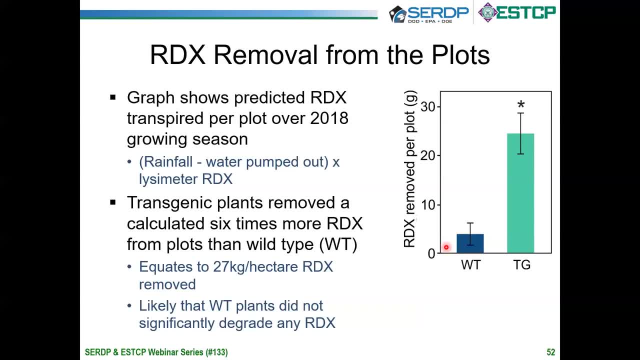 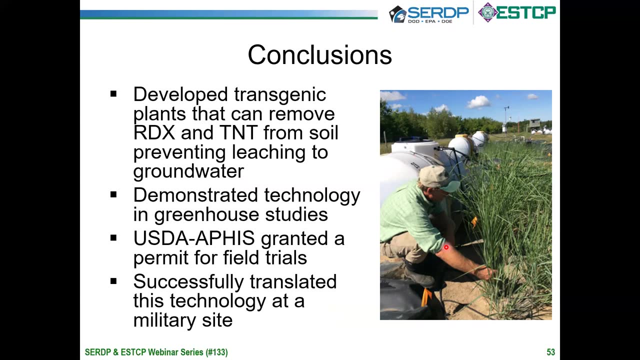 And so the RDX there will be available to herbivores grazing on any of these plants On contaminated sites. So, in summary, we've developed robust transgenic plants that can remove RDX and TNT from soil, potentially preventing leaching into groundwater. 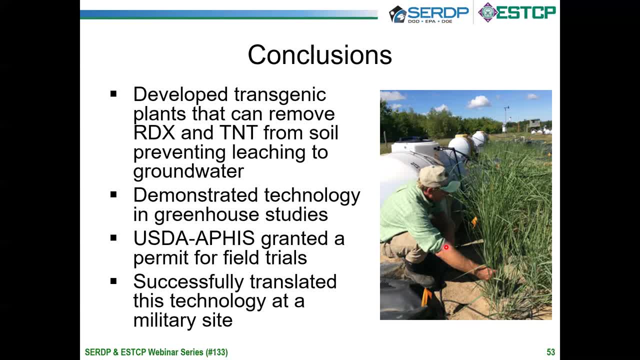 We've demonstrated this for both TNT and RDX in greenhouse studies. We were then granted a permit for field trials for RDX degrading plants, and we've demonstrated that this can be successfully translated to a military site In terms of benefits to DoD. 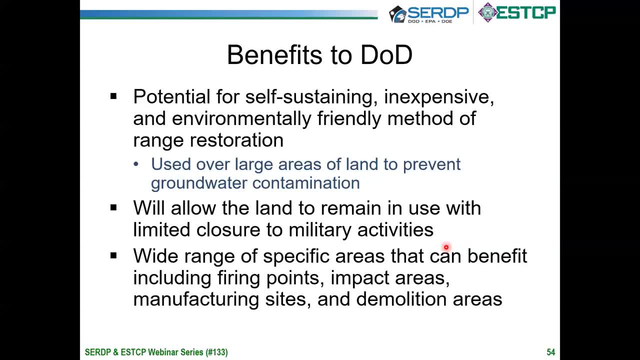 so these plants have the potential for self-sustaining, inexpensive and environmentally friendly ways of range restoration that can potentially be used over large areas of land to prevent groundwater contamination. Importantly, they will allow the land to remain in use with limited closure to military activities. 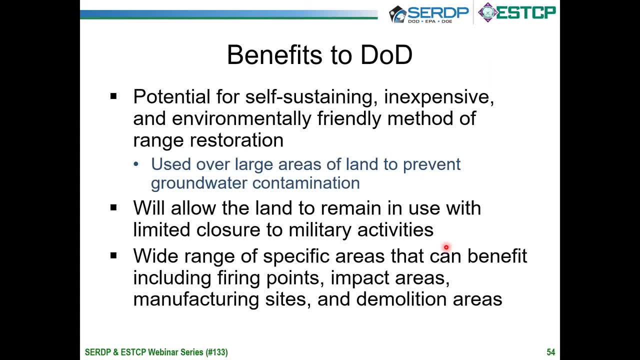 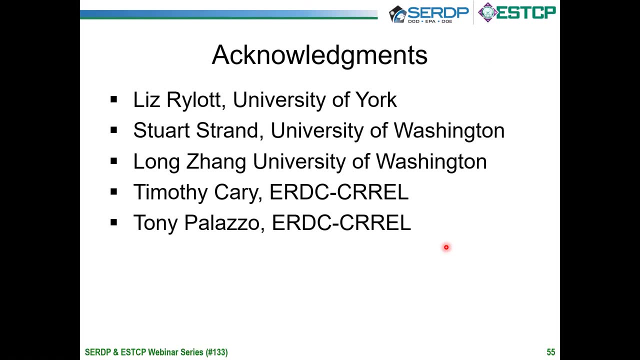 and a wide range of specific areas that can benefit, include firing points, impact areas, manufacturing sites and demolition areas. I would just like to finish by acknowledging my colleagues and partners on this project, So Liz Reilert, who works with me here at the University of York. 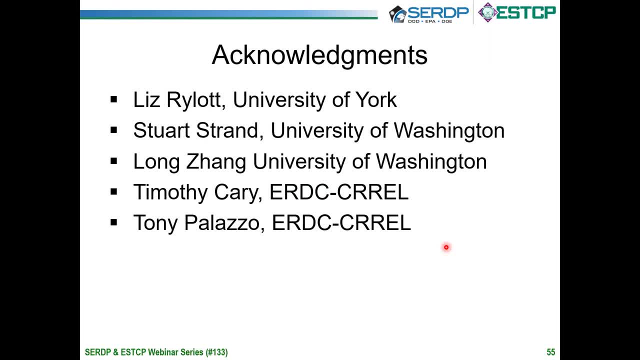 Stuart Strand and Long Zhang at the University of Washington and Tim Carey and Tony Palazzo at ERDC-CREL. And finally, just thank you. I'd like to thank you for your attention and I'll be very happy to answer any questions. 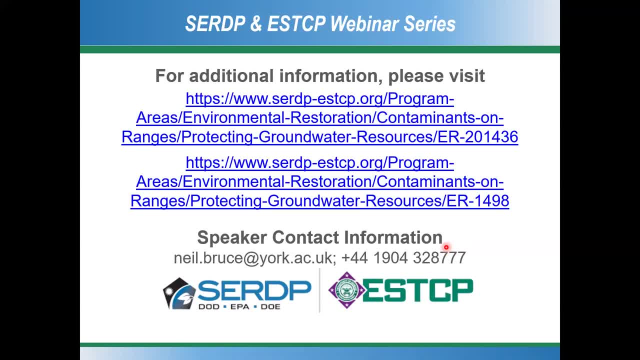 And, as I mentioned earlier, there is some more detailed information on the results of our field trials on this ERDC-CP website. Thank you, Thank you, Neil. First question is: how deep can the root system go to uptake and then remove RDX and or TNT? So with the switchgrass they can grow to a depth of about a metre into the soil. Great, thank you. And how long do you think that the degradation with the switchgrass can persist? So as long as the plants are alive, they will have that capability to degrade RDX. 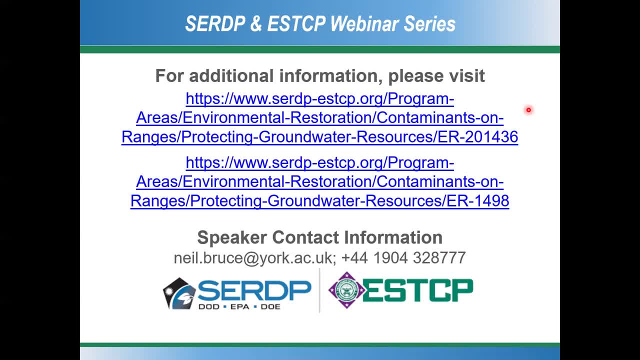 because the gene is being expressed along with other constituent expressed in the plants. So the plant is continuously making the enzymes that degrade RDX. Okay, excellent. This question is from the Hawaii Department of Health. In the field experiments were multiple lysimeters placed in some plots. 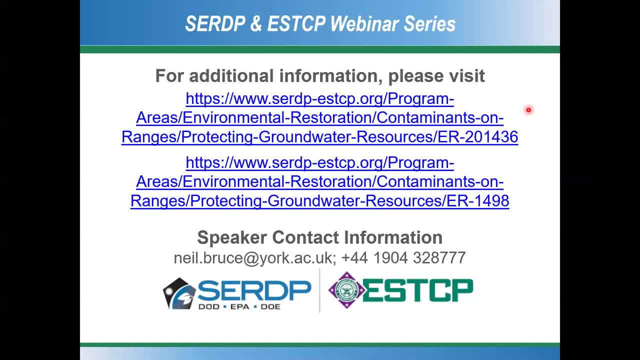 to look at the variability of RDX in soil moisture. Yes, we did have multiple lysimeters in there. We did see differences in the movement of RDX through that soil, which perhaps wasn't surprising, because obviously it's not a completely homogeneous system. 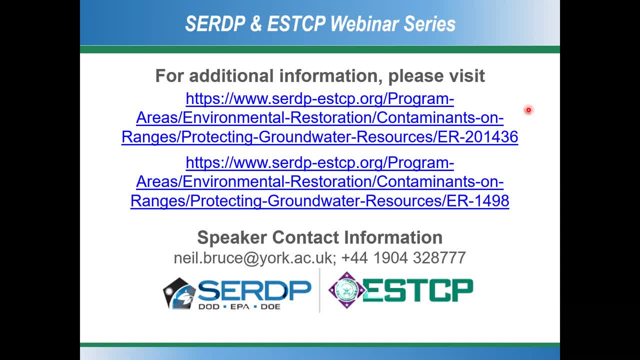 So we were taking multiple samples and then taking the average from them. Okay, And how are the plants affected by chunk explosives, from low-order detonations? Did you consider pieces of the explosives? Yeah, so they're not affected, So obviously they can only take up RDX. 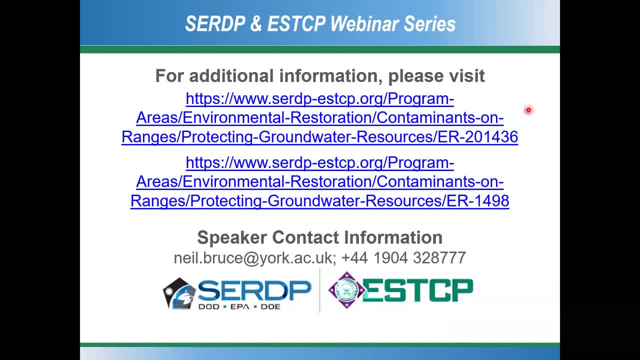 when it's in solution, So when it's in a particular soil, when it's in a particular form, it has no effect upon the plant. Same with TNT: It's only when it gets dissolved that it starts impacting on the plant in terms of toxicity. 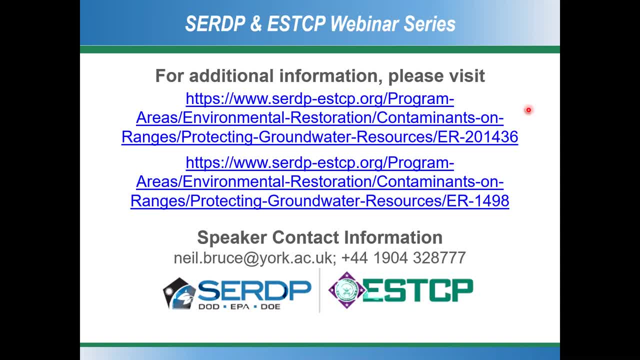 but also in terms of being taken up and degraded and sequestered. So that's what we were trying to mimic in these plots, where we're using particulate RDX mixed in with sand. So we've got, hopefully, a fairly homogeneous coverage on the surface of the soil. 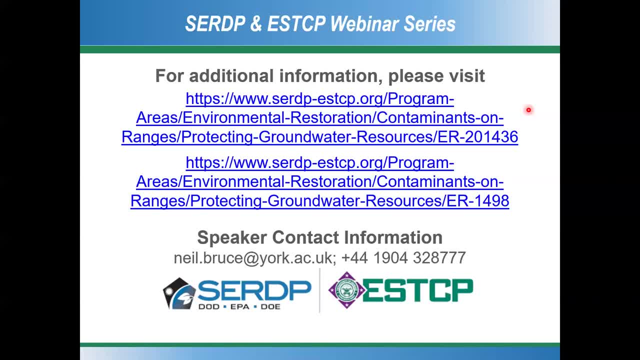 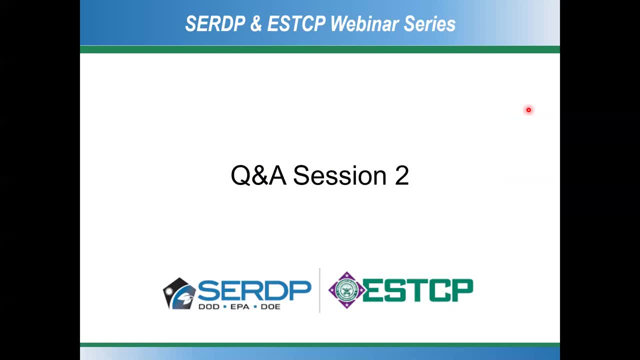 And then, when it rains, that RDX is then being dissolved and is then migrating through the soil and then being taken up by the roots of the plants. And since the root system is limited to the top meter or so, in that situation can the explosive migrate below that horizon depth? 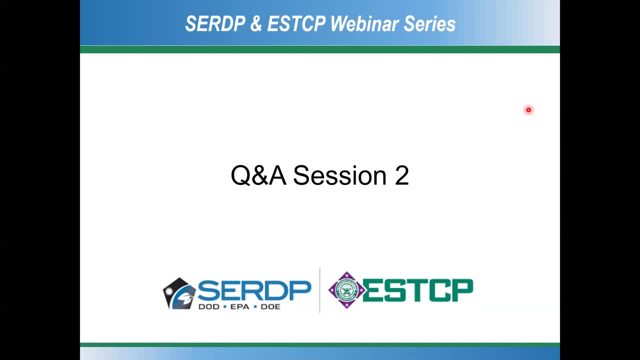 So it will really depend on the amount of vegetation on the site. So obviously the RDX is going to come into contact with the root systems. So, as we've found in our soil lysimeter studies there, we didn't see any migration beyond the root depth of those plants. 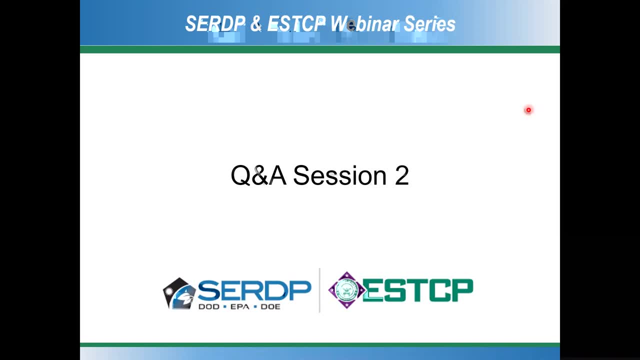 Out in the field. you're not going to have that same amount of coverage of biomass, So whether you could capture it all we don't know yet. One of the next stages will be to carry out trials in plots that are not lined. 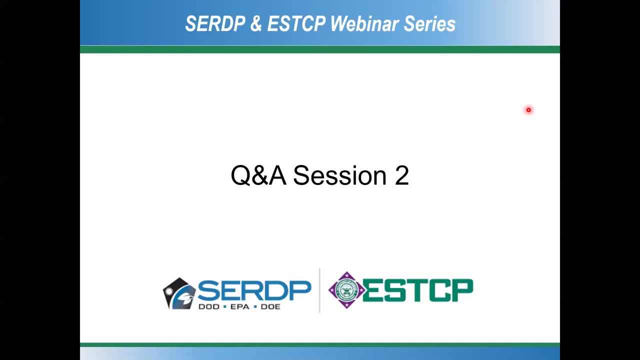 So that would be a further stage ahead, really, in terms of where we need to go in terms of the evaluation of these plants. So those trials: I forgot to mention that those plots were lined So the RDX couldn't escape from those plots. 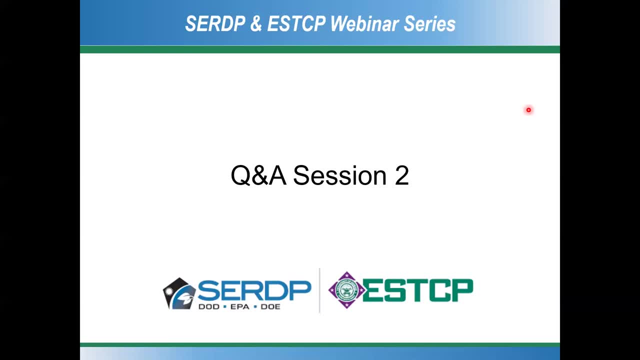 Thank you. This question is from the US US Army Chemical Biological Center. Have you looked at different uptake rates relative to soil types or properties? That's a really good question And it's not something we've compared So in Fort Drum. 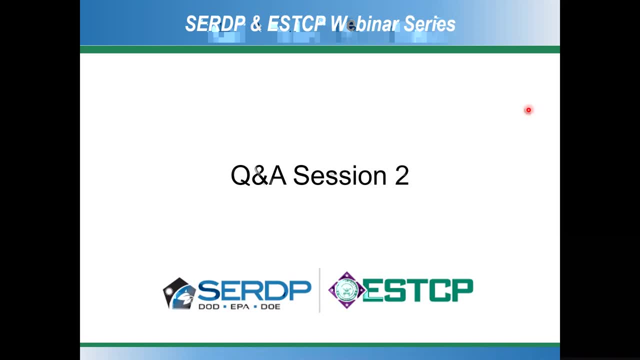 it's a very sandy soil So RDX will migrate through quite quickly. Those soil microcosm studies that I showed were done in a sandy soil. Here at York we've also done some work with sort of compost, rich soils With RDX. you don't get so much interaction between the organic components in the soil, But TNT that will make a big difference. So TNT will bind quite tightly to organic material and clays which will limit the speed at which it migrates. So it's an important question. 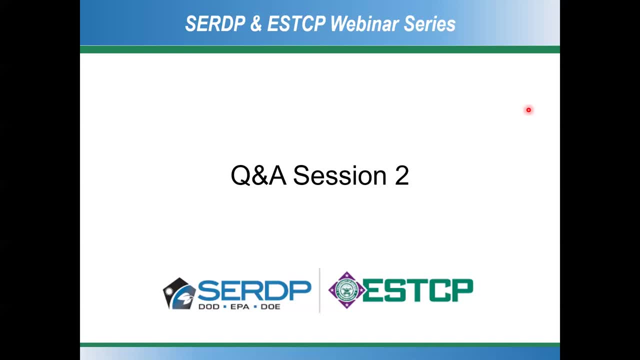 and not something we've fully evaluated yet. OK, thank you, And we have one last question for you And then we'll bring Dom back for questions for both of you. Do you think that the enzyme XPLA could be used to treat RDX? 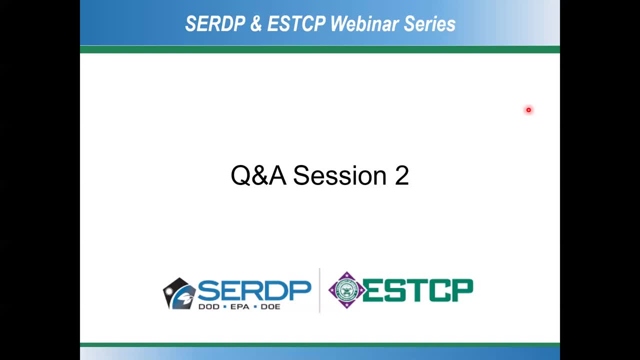 in a groundwater plume. somehow It's a nice idea. Part of the problem of using purified enzyme is one its stability, And secondly it requires a cofactor for activity, And that would just make it too prohibitively expensive to ever use the free enzyme alone. 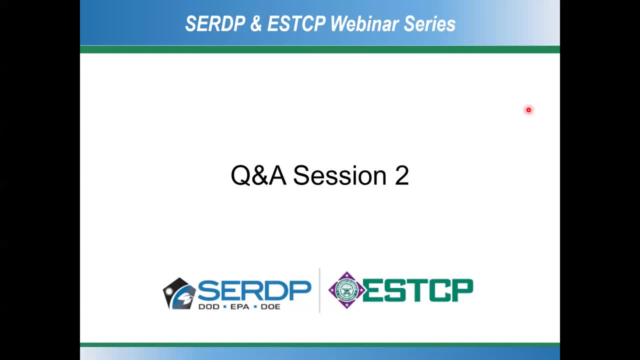 OK, thank you, Neil. All right, we have Dom back on the line. Dom, we received a few questions from the audience about the applicability of the quantum chemistry approach to other types of contaminants. So can it be applied to metals and organometal compounds? 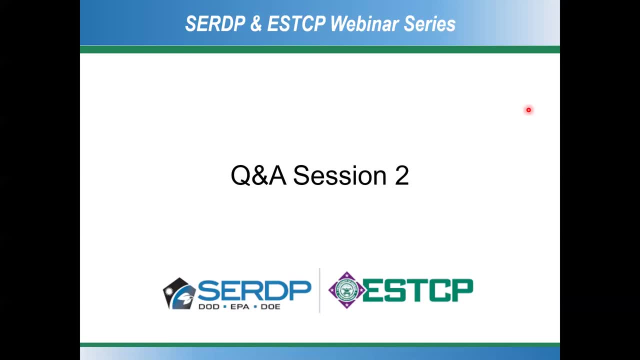 like methylmercury, And then I think you had also mentioned PFAS a couple of times. Yeah Well, metals. The problem is that the electrostatic energies involved in ionizing chemicals make the current formulation of the Abraham model inapplicable. 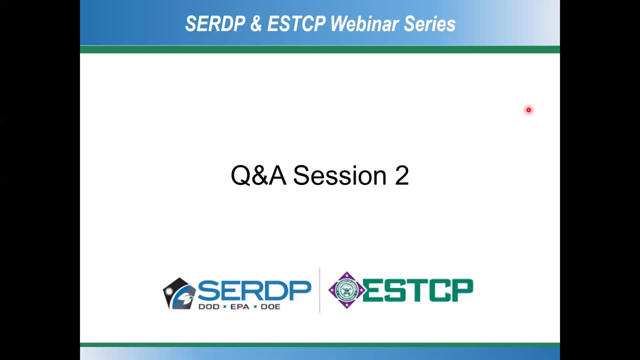 I mean if you had a neutral, for example a methylmercury, dimethylmercury, for example, it's possible Calculating solvation for organometallics. I don't know if it's ever been tried. 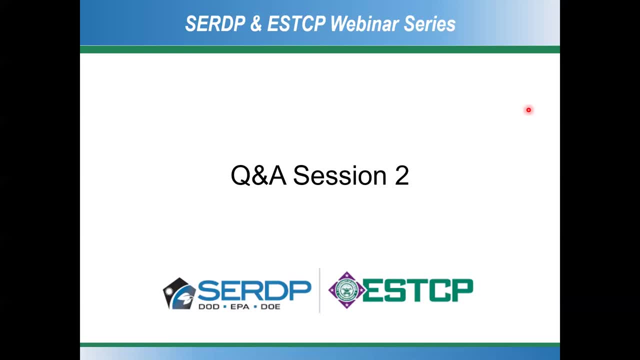 but certainly there's a fair amount of data. So that would be an interesting exercise. The mercury as a molecule, as an atom, in a calculation could be difficult. It's rather large but there has been experience doing those sorts of organometallic calculations. 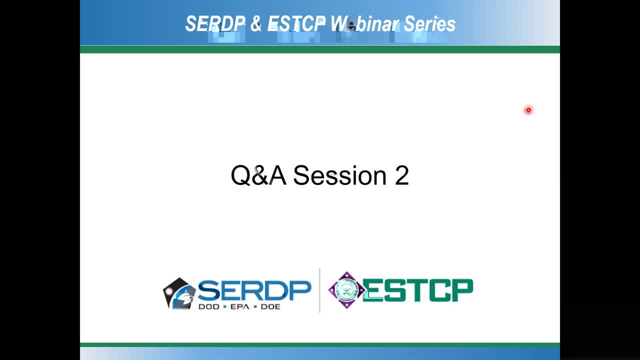 So I think it's possible. The problem with ionized chemicals, specifically anions and fluorinated material, is that the quantum chemical solvation models don't work very well at all for anions in their current state of applicability. You need to. 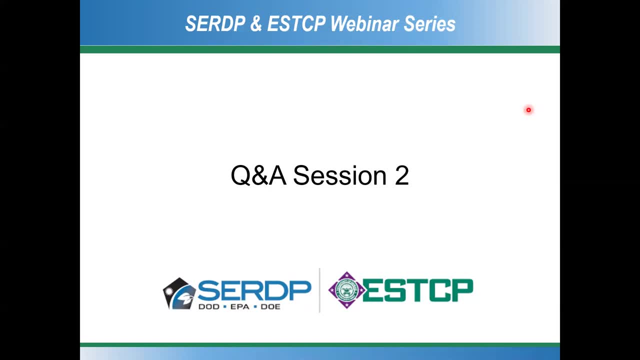 and the reason is that they are. is that the well? first you have to calculate solvent water partition coefficient for anions. You can do it. the calculations will produce numbers, but then you have to deal with a regression and it is not clear that the numbers are good enough. 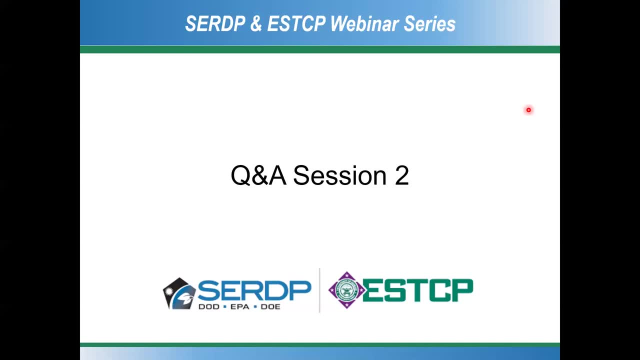 to be solved by the multiple. the multiple 53 data points approach, So overwhelm the errors with a lot of data. It's sort of a standard statistical way to attack it. We are working on some methods which both improve the solvation calculation and also make a direct estimate. 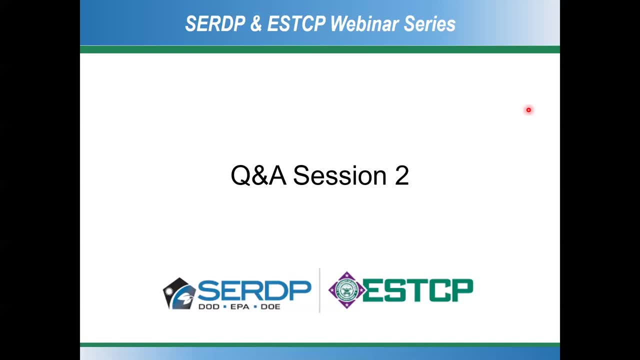 of the hydrogen bonding and hydrogen accepting capability of PFASs. It's simplified because they have the donation and accepting group is in the at the carboxylic head of the thing, of the molecule. So it looks like it might work. 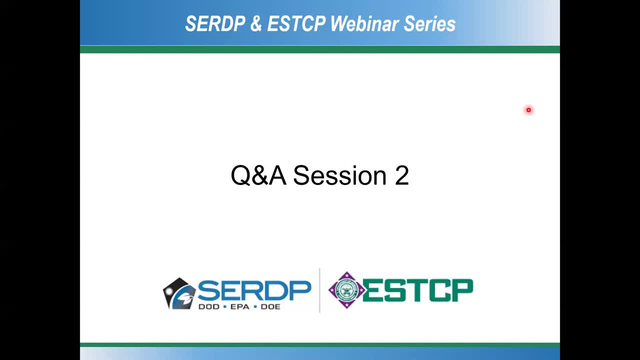 but right now it's pretty difficult. I should also tell you that Abraham and Accree have published a method that generalizes the model and adds an additional term- J terms, lowercase and uppercase J terms- to deal with the electrostatic and ionic contribution. 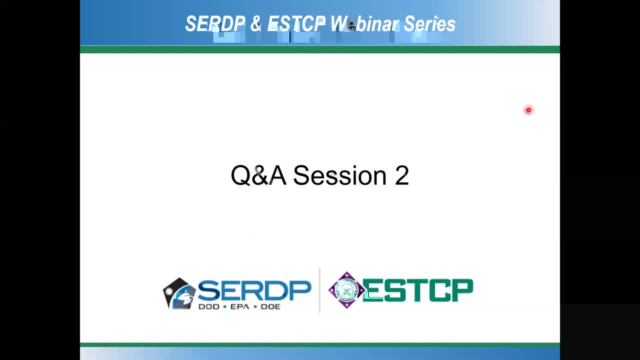 then cationic contribution. The problem is that you haven't got system parameters for the Js And so you can't use all of the system work that's been done over the last 40 years And as a consequence it's not terribly practical. 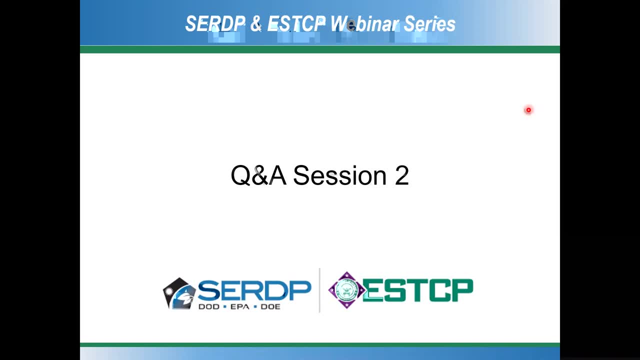 So the methods we're attempting to use, which are showing some promise, I might say, utilize currently available system parameters and calculate the normal five solute parameters, but using better and better adapted methods for charged compounds And also the fluorinated piece. 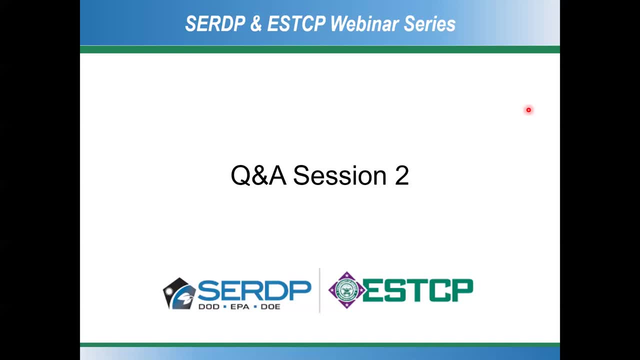 by the way, fluorine atoms are also something of a problem from quantum chemistry, although that's pretty well understood nowadays. Okay, Thank you very much, Dom Neil. there's a similar question to you. Do you think that this plant system, or others, 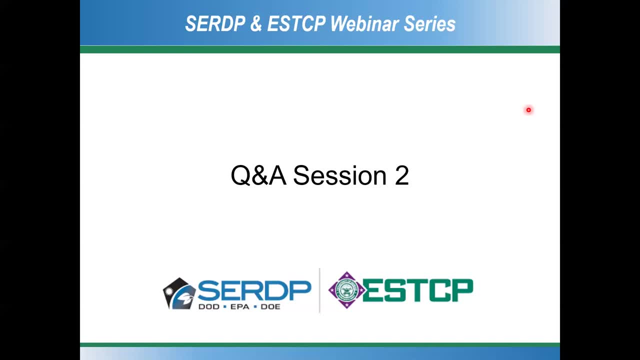 could be applicable to other explosives compositions in the future? Absolutely, And of course, TNT and RDX are looking to be replaced with incestive munitions And so, for example, Dinan dinitroanisole we've shown has the same mechanism of toxicity. 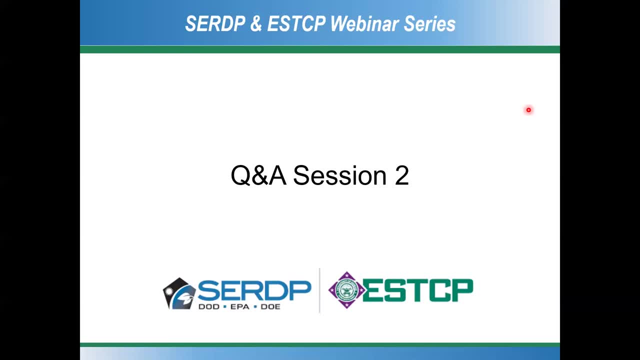 as TNT And the enzymes that that are active against TNT, that detoxify it, have no effect on Dinan, So that gets up into the aerial parts of the plant. So that's going to be more challenging, I think, to resolve. 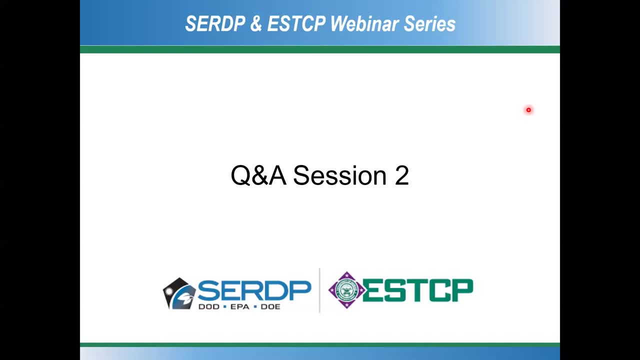 And likewise, NTO is much more polar than RDX and migrates very quickly through the soil And, like RDX, the plant has no activity towards it. So I think with again, with both types of explosives, we're going to need to take a. 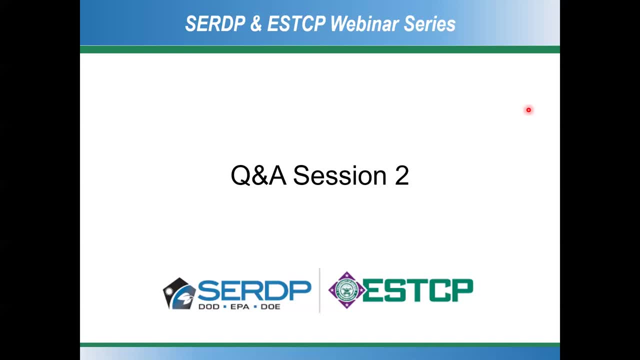 you know a GM approach in terms of engineering plants to be able to tackle them. But yes, absolutely, And there are many examples now of other organic pollutants that can be remediated using this type of technology. Thank you, Neil. we also have a follow up clarification. 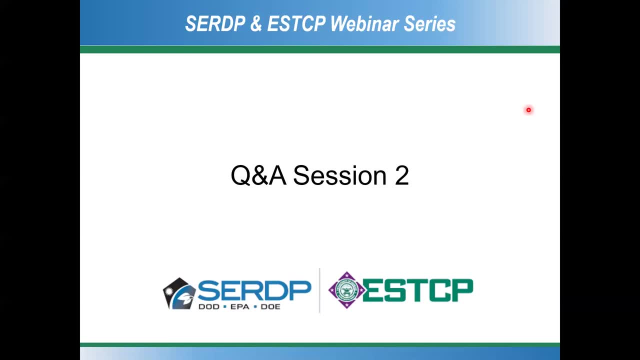 question from earlier. Detonations can result in cratering in the impact areas. Have you considered whether grass cover could be maintained in a cratered area? No, we haven't, But of course agronomy of these sites is an important part of maintaining these sites. 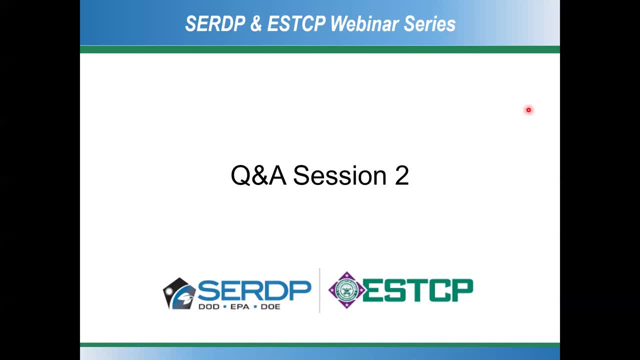 So yes, if there's a huge explosion, you'll remove all the plants that are there. that's in a case of hoping that you can replant those particular sites. But you know, I think there's. yeah, clearly, if you've got a six foot crater. 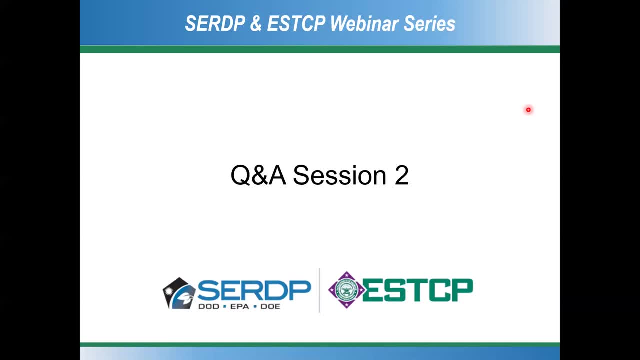 then it's going to be challenging for any plants to survive that sort of detonation. Sure Well, this time I would like to thank both of our speakers very much for the very excellent presentations and for answering so many questions. And our next webinar in the series. 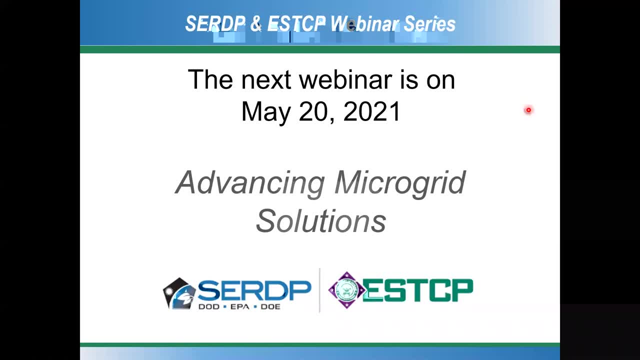 is on Thursday May 20th and it will present DOD funded research efforts to improve and enhance microgrid solutions on military installations. Registration is open now, so please visit the CERT of an ESTCP webinar webpage to register both for this next webinar. 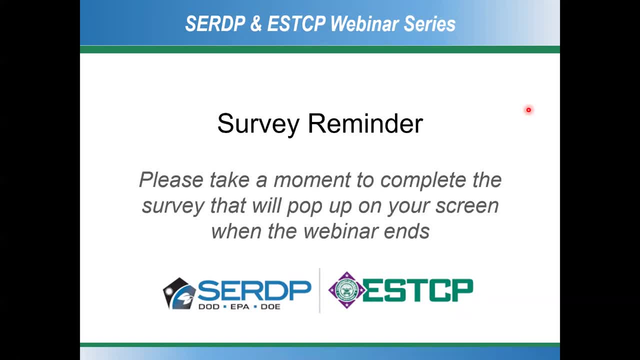 and other future webinars. Before we wrap up, I would like to remind you that both the audio and a copy of the presentation of today's session will be archived on the webinar webpage in case you would like to refer to them in the future. 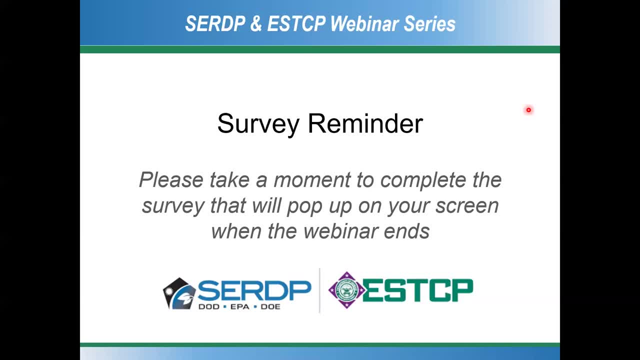 We would appreciate it if you could please take a moment to complete the survey that will pop up on your screen at this time, And this concludes today's webcast. Thank you.